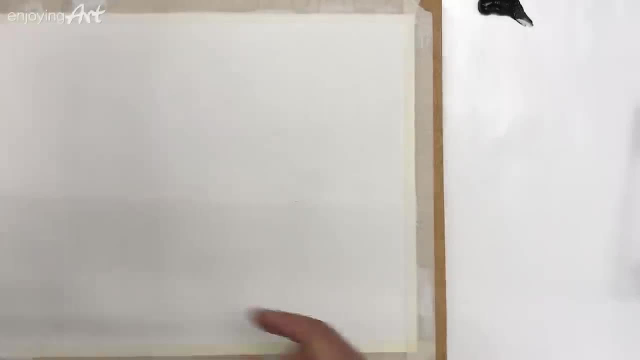 You know acrylic colors. they dry pretty quick And you don't really want to give too much. Try to have the best estimate so that you don't need to waste the color. That's good. Before we're going to start, make a grid. 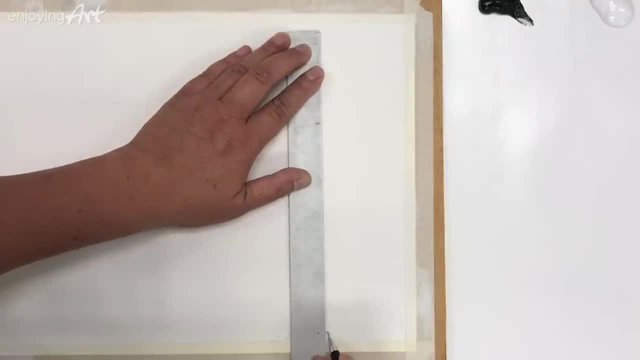 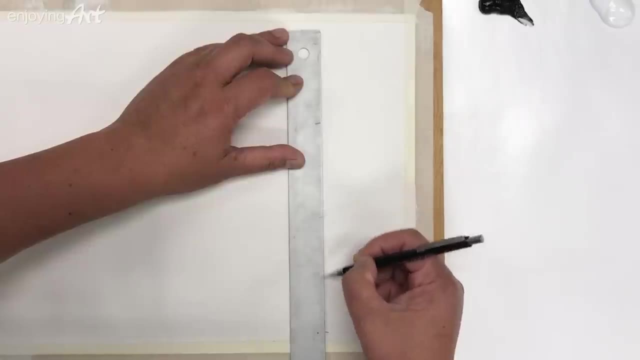 This is the top, This is the bottom, So let's divide it to five. So there will be two probably here And let me see Two probably here, and then three on this side. It's beautiful, You don't have to make it exactly. 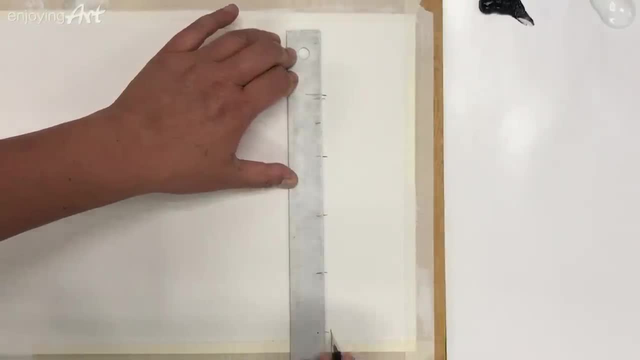 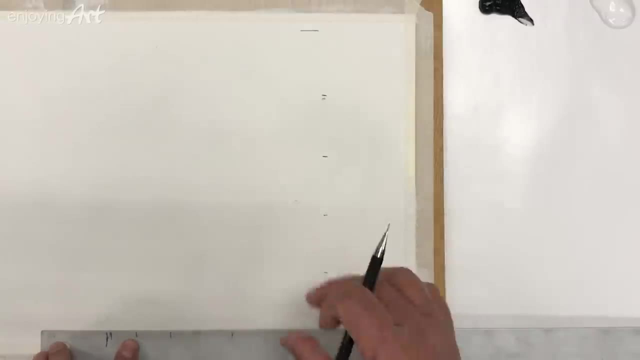 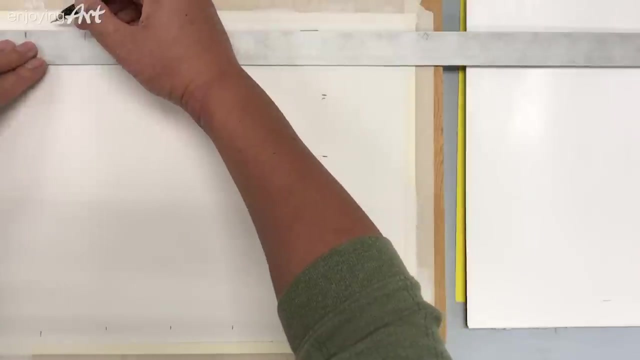 So now one, two, three, four, five. Going to turn around, I'm going to center this on the width, So that way the height and the width are exactly the same, Approximately over here. I'm going to draw the line all the way here. 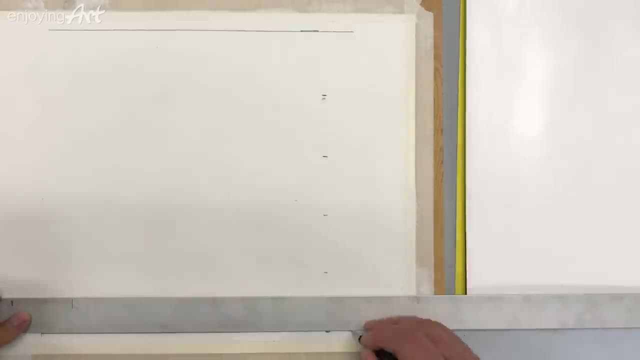 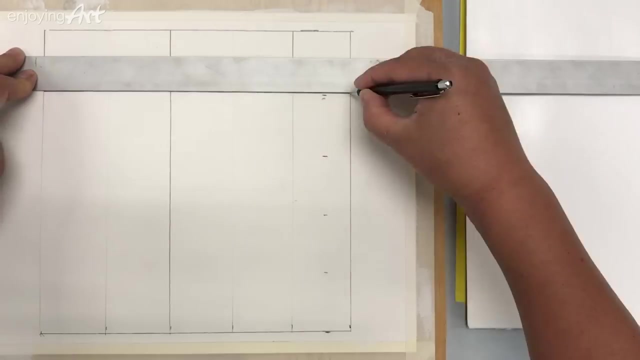 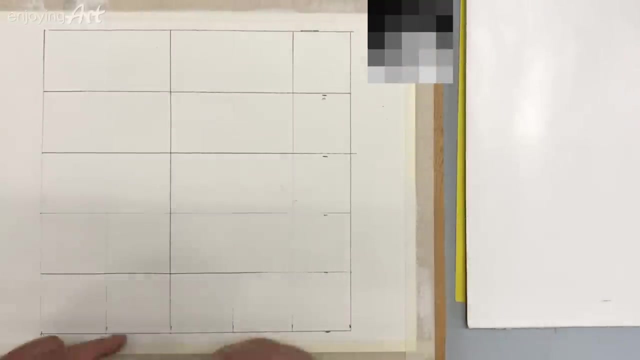 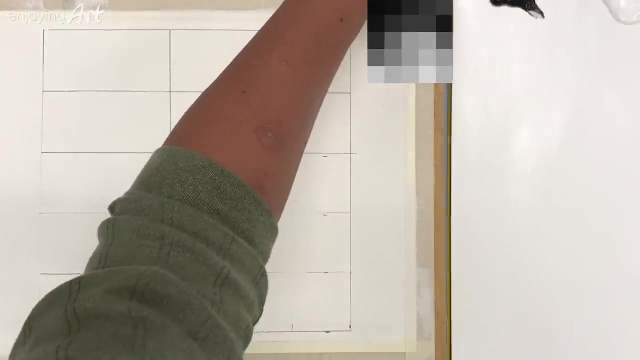 Okay, cool, We're ready. We're looking at the grid. Let's take a look at which one is the darkest color On the left top corner right. Okay, this is good, So take a little water, Put this down here. 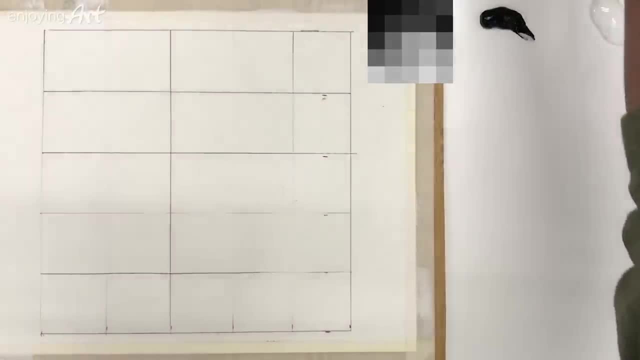 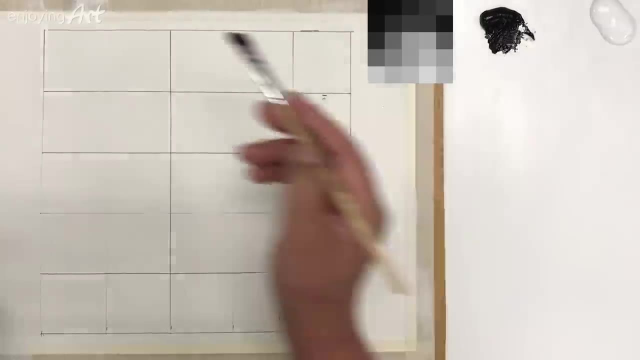 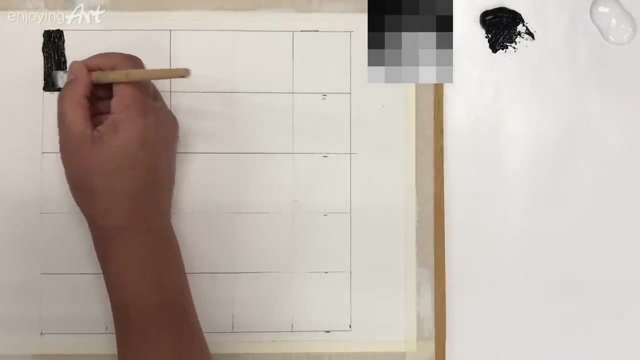 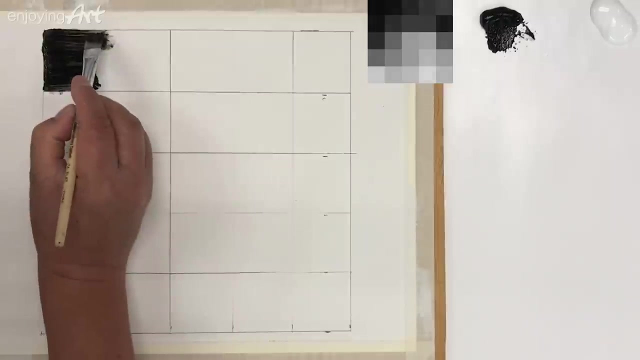 Okay, We're going to just take the whole black. The darkest color would be here. Take the black. I'm going to make it in here After you mix with a little water, because you have to dilute it a little bit so that you will be able to move the color right. 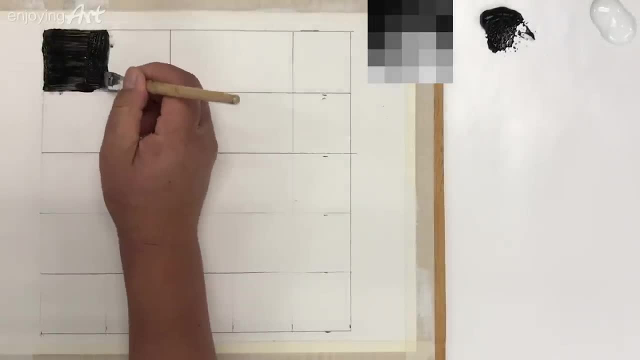 So I'm going to put this color over here so it looks a little bit lighter. That's okay. If you want it to be darker, you can come back. And by the way, the acrylic colors: after it dries it always looks a little bit darker than when it's wet. 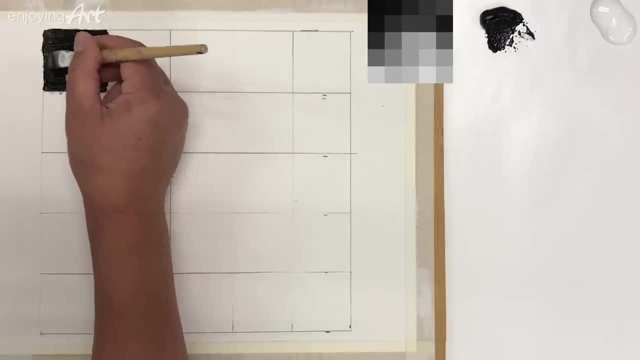 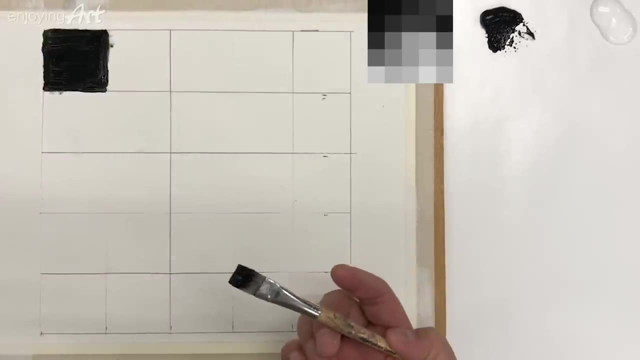 It's kind of very different from watercolor. Watercolor is just after it dries, it always looks lighter. Now what's the other color? Similar or maybe a little bit lighter, And let's see We can adjust the color. 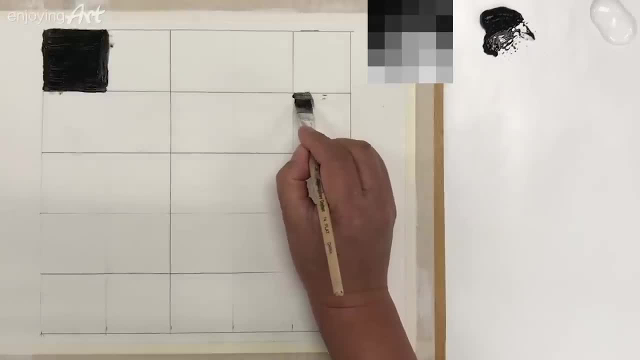 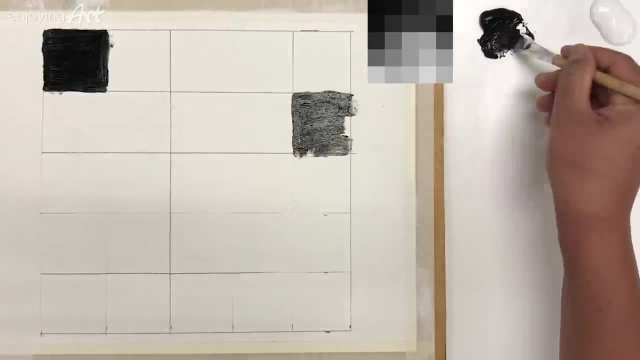 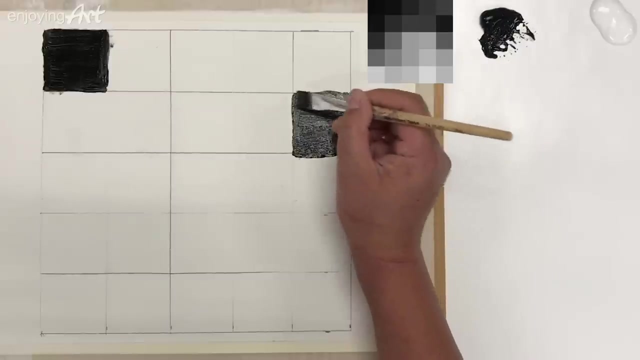 I think there's a color over here that's also very dark. right, Looking for that color, I'm going to make it in here. This color also very dark, So you don't have to go by like a one square and then a square next to it. 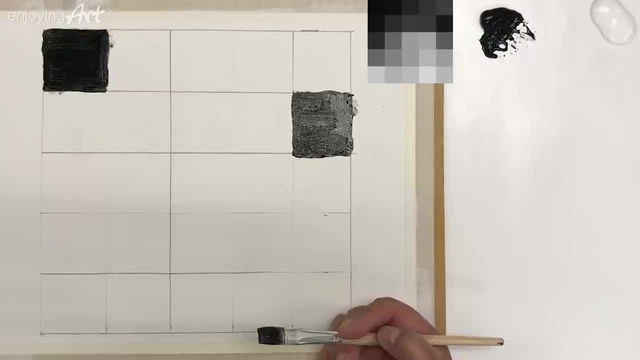 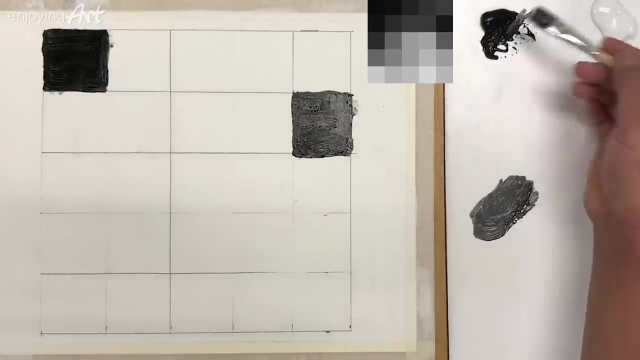 Looking for that for now. Now we're going to looking for the color a little bit lighter And a little bit lighter, And then take a little bit water. I'm going to put it over here, So let's see, I already mixed this color. 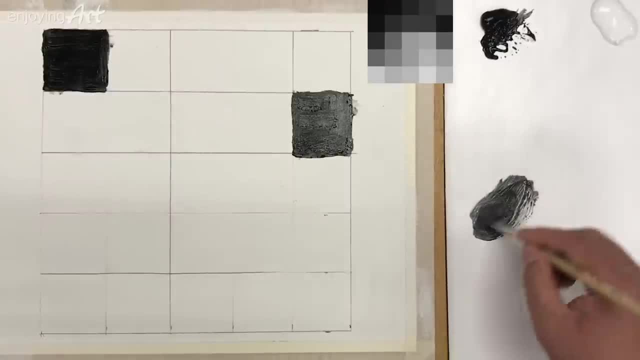 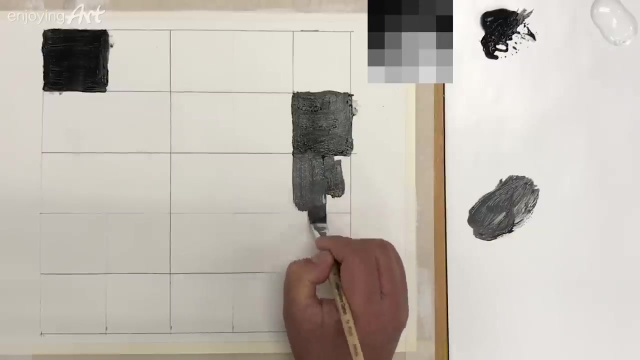 And maybe it's just thinking about compare. What color is this color? I think this color is very much here. Still look a little bit too dark. I'm going to mix a little bit white into here. I'm going to mix this color. put it over here. 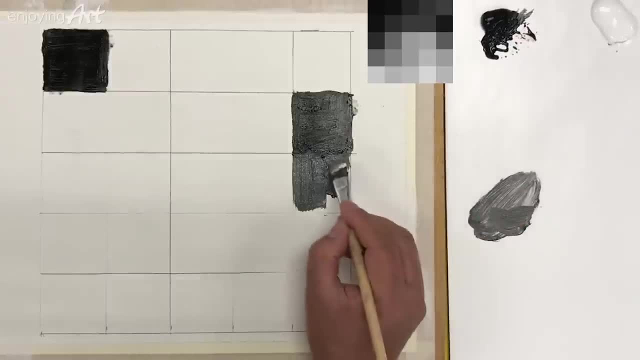 Maybe even a little bit white Like this. You're going to see after you dry. you're going to make another assessment, Compare the colors. Oh, this color still need to be lighter, And then you can mix the new color, right. 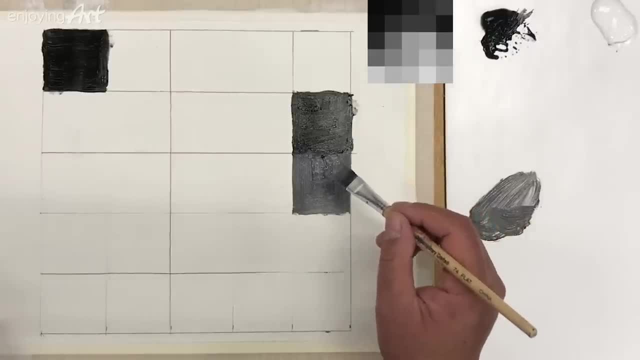 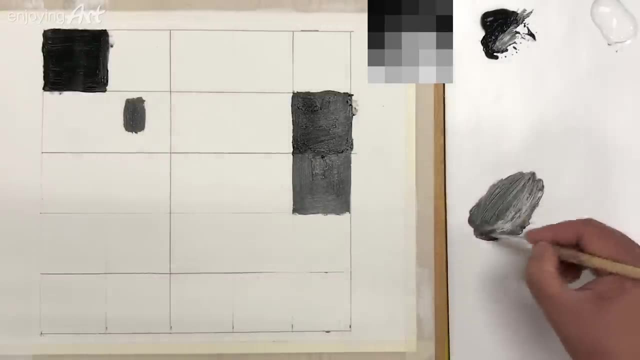 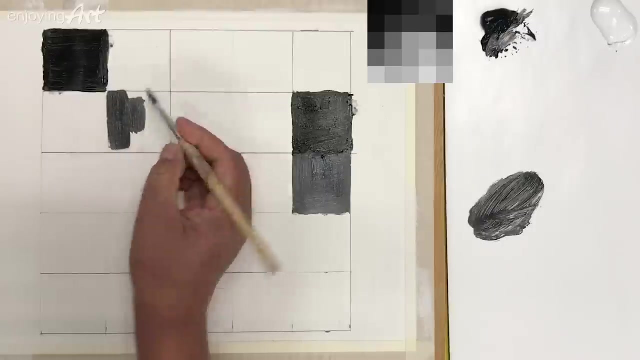 Okay, Compare this color. which color is similar? I think this color is similar. Over here, maybe a little bit darker, I'm going to put a little bit black color in here And this color is similar. So your eye, keep comparing. 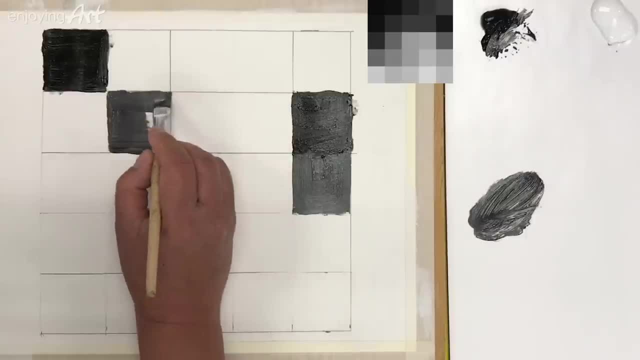 Comparing, comparing, comparing. Also, if you, when you're doing a complete painting, you look at a color over here and then look around in a whole painting, compare And they say, oh, it is the same color on the forehead. 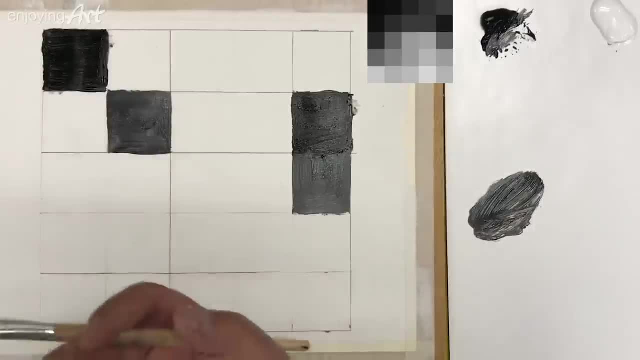 Actually in the neck. In that case, you can put that color in the neck as well at the same time. So before you wash your brush, right? So the same thing similar that we are doing here. Let's take a look. 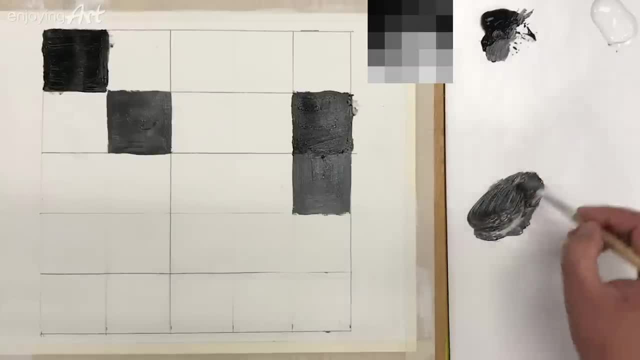 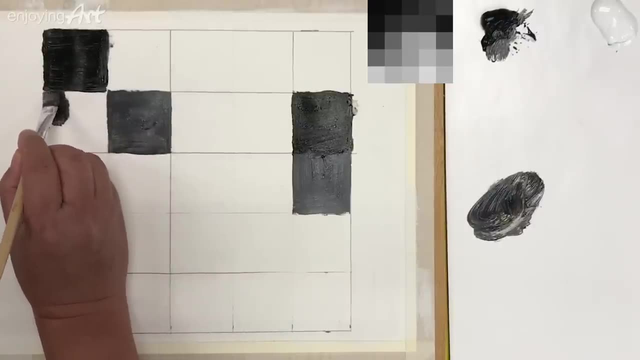 I'm going to add a little black. Then take a look And this color, actually this color a little bit darker than this but a little bit lighter than that. So you always compare, Compare and compare the color And let's see. 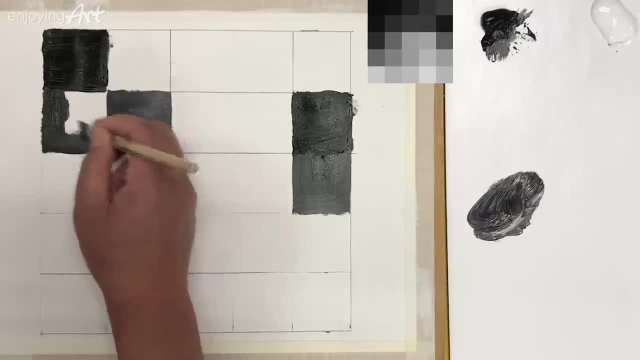 Do a little bit, Put the color in Like this, Lighten in And, as you see me painting last week, the process is to circulate. You're not just trying to finish the forehead before you're doing anything else, because you just put the base color and then you come back. 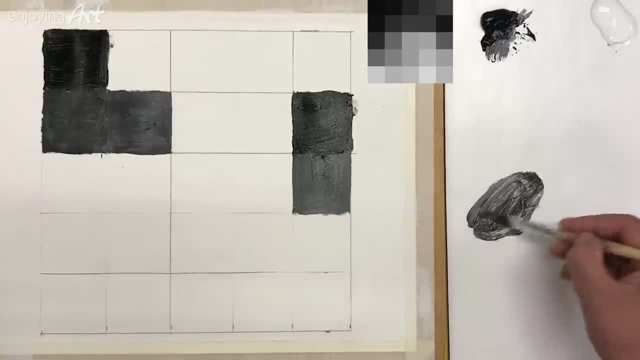 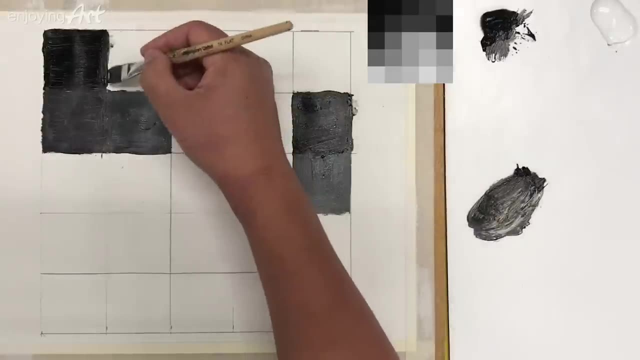 and get more and more into the smaller, smaller shape and smaller, smaller details. Now I think the color up here I'm not sure- from a little bit distance that could be this color a little bit darker than that. So I'm going to add a little water. 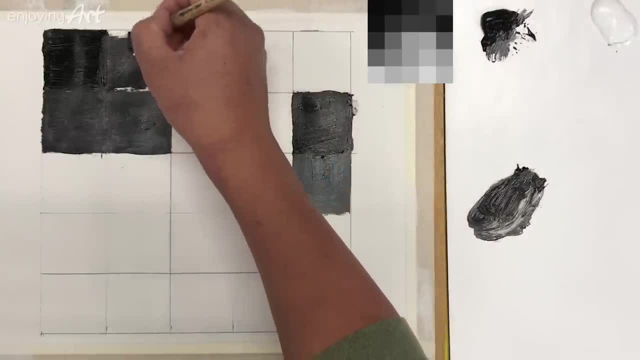 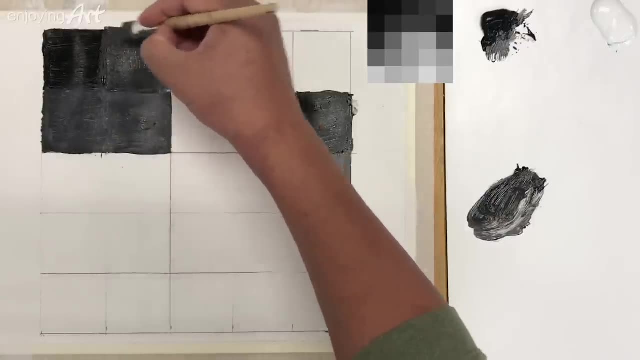 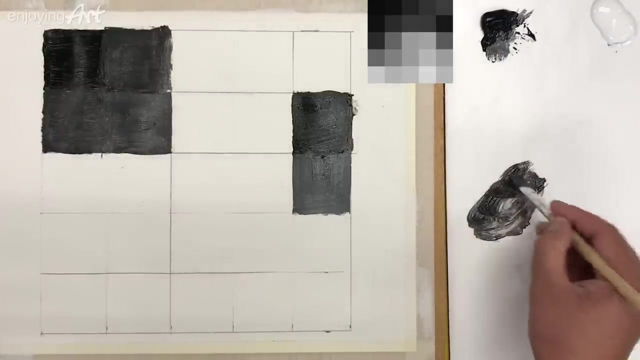 I'll make it a little bit easier to move. I'm going to move the color. So this color a little bit darker, a little bit lighter than this, but a little bit darker than that. I'm not sure that it's actually much dark enough compared to this color. 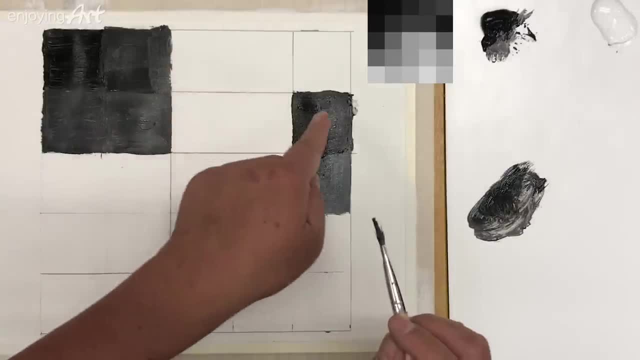 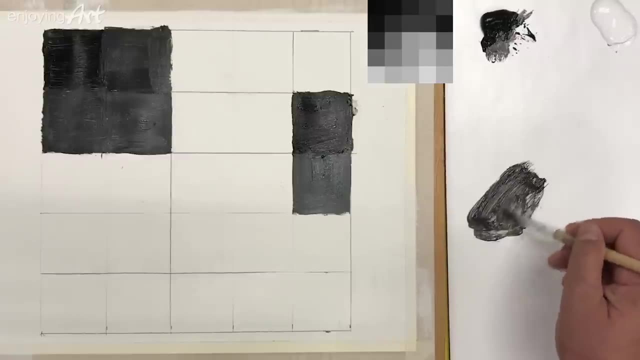 Okay, this is good. Now take a look at this color. This color a little bit lighter than that, but maybe a little bit darker than this color. I'm going to mix that color. So that means definitely, compared to this color, a little bit lighter. 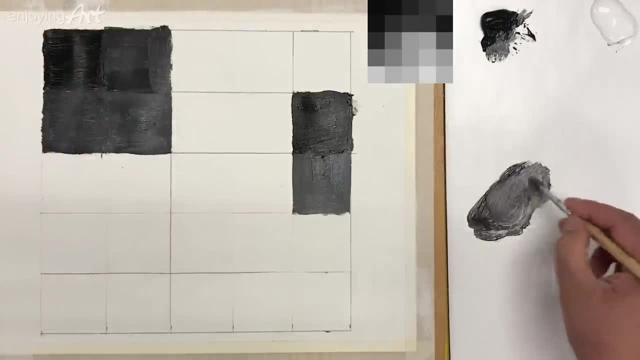 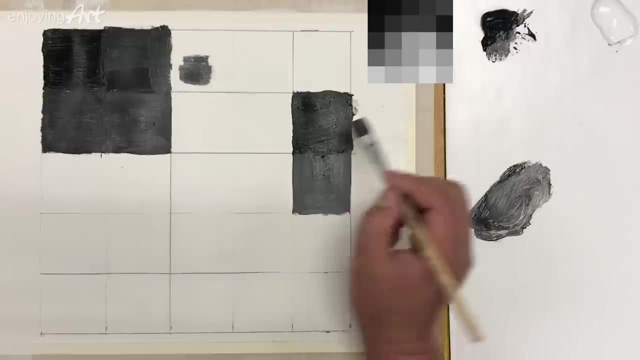 So I'm going to take a little white- right, Let's put it on first- And definitely a little bit darker, because this color, oh no, actually a little bit lighter than this color, but a little bit darker than this color. 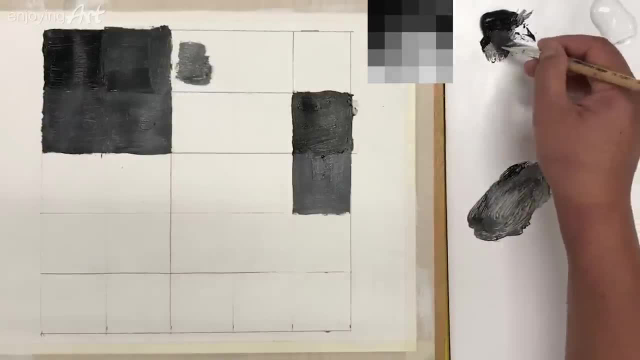 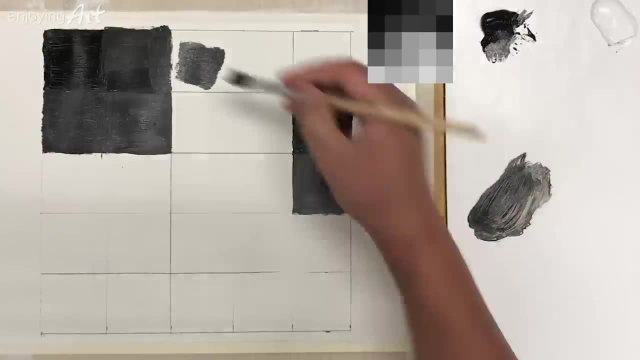 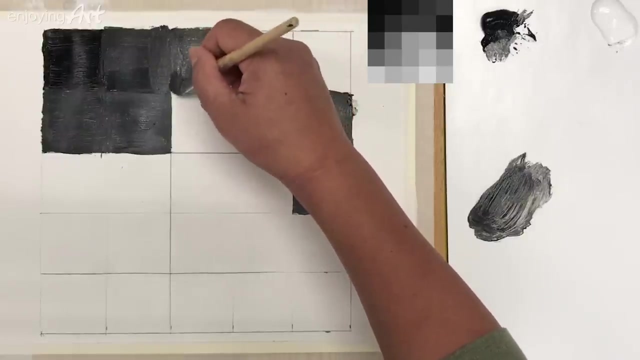 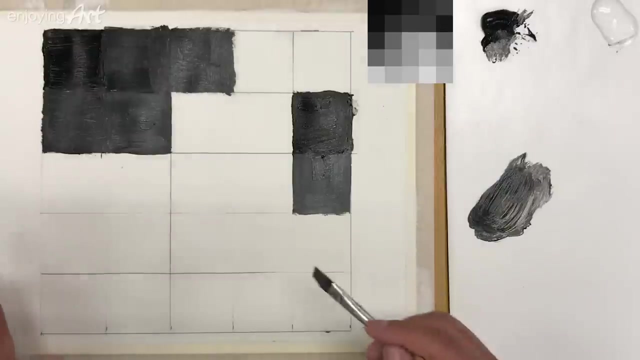 So take a little black color and put it on. I think still need to be a little bit darker, Okay, like this. Then I have to make it very clean in the square And we're going to see the difference, Okay, between this color and this color. 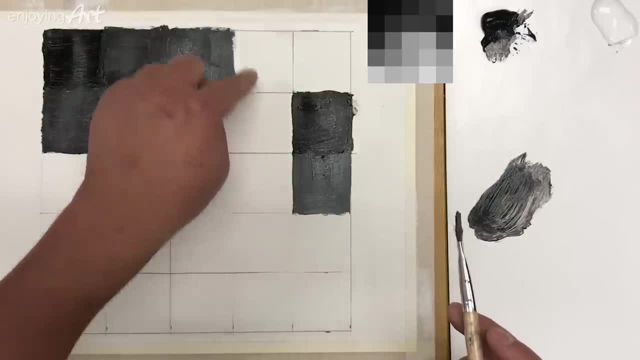 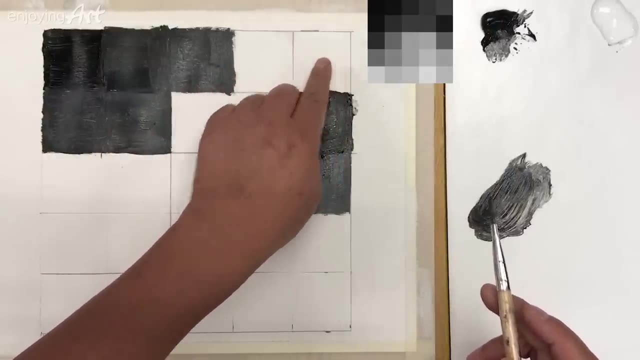 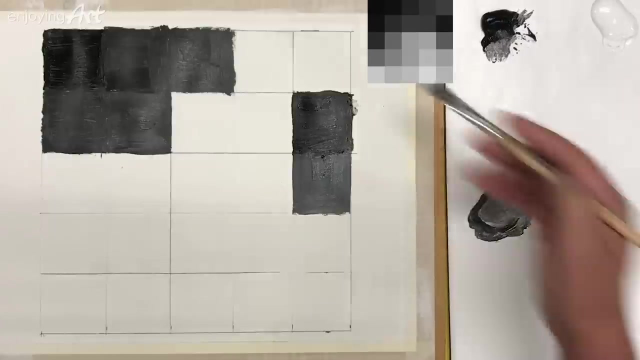 this color looks very much the same, right? Actually, there's one, two, three, four very similar, But this color, I think, a little bit darker than this color, right? So? but this color definitely lighter than this color. So what I can do is just take a little white, right. 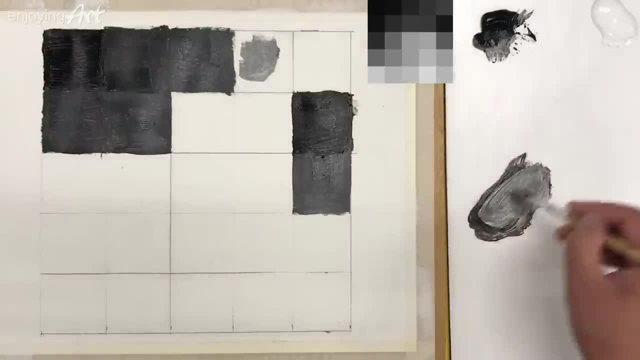 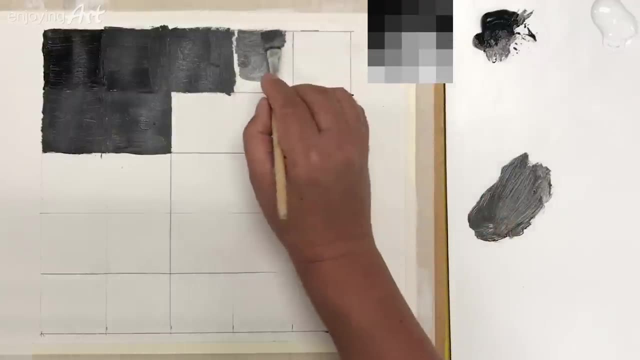 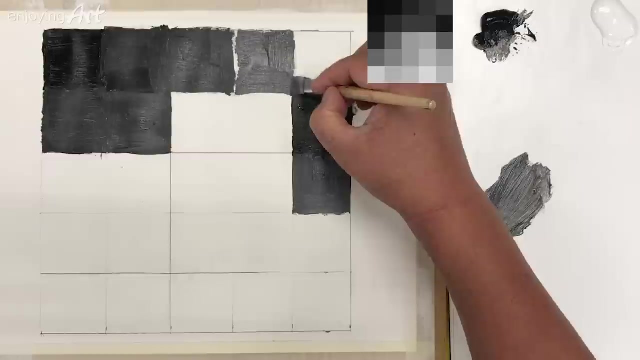 Put it over here. Oh, probably a little bit too light. Let's take a look. But you never know, After you dry probably look too dark or maybe dark enough. Okay, And the painting process is always, every step, every action that you take. it involve what observe. 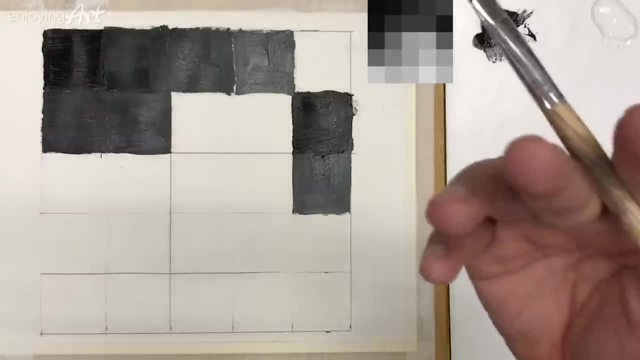 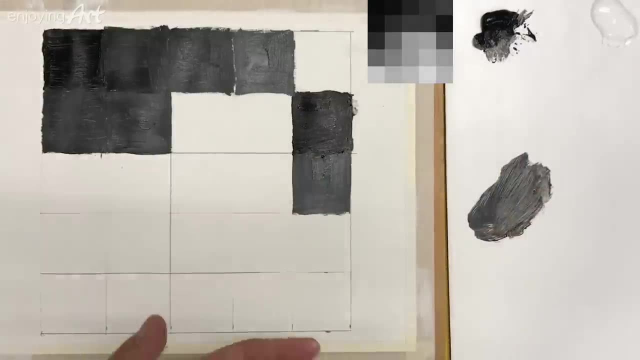 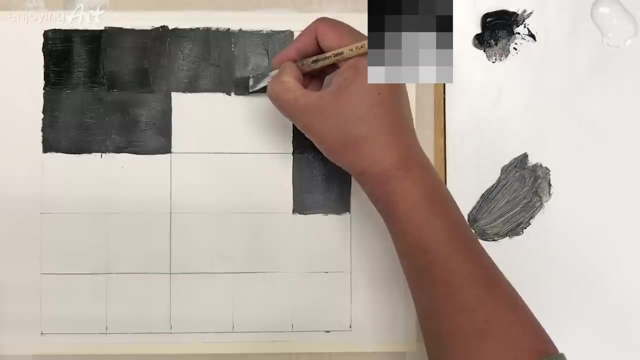 either observe from the real setting- like I want to put an apple over here, a person sitting in front of you- or observe from the reference. And second thing, after you observe, you still need to analyze it. So every action that you take, 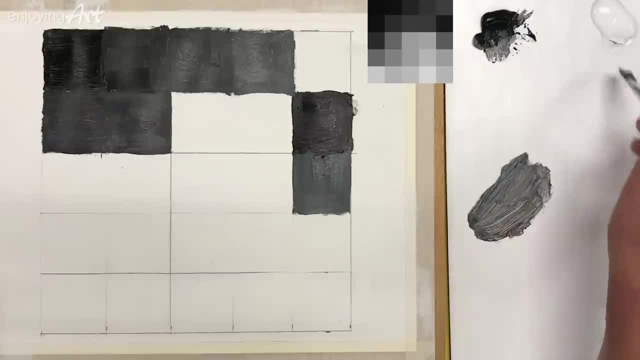 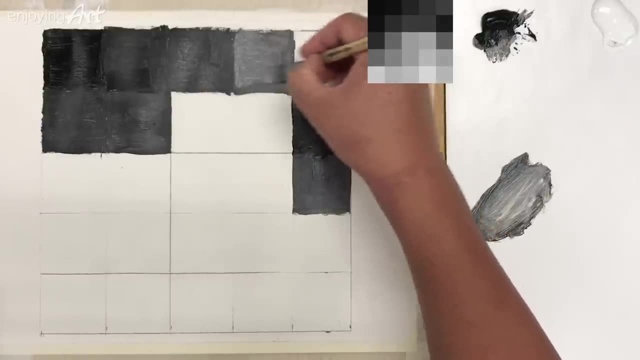 it is the time that you're making a choice. I think this can be a little bit lighter, Otherwise, between these two color looks too much together. Okay, Like that. So actually better off, it's just flash over, Okay. 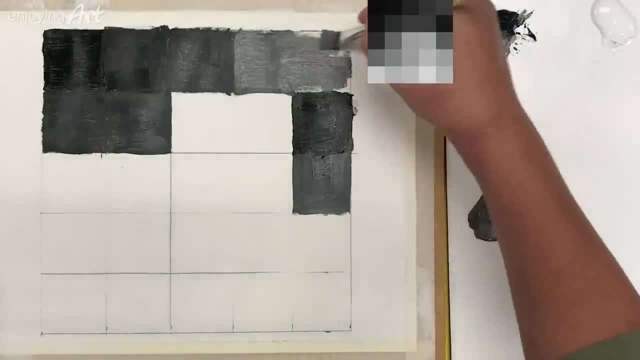 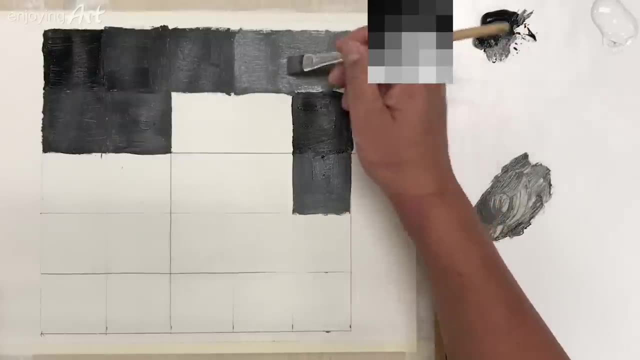 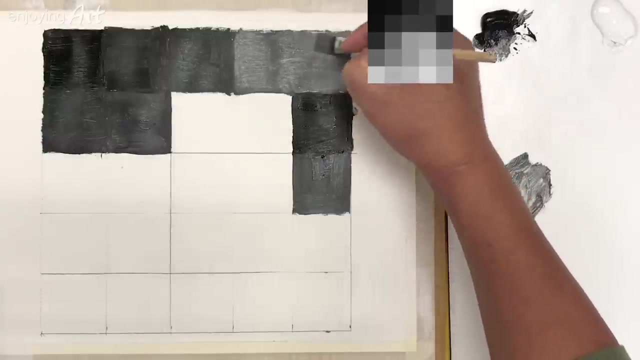 Because these two colors too much, look too much the same, And maybe a little bit, little bit lighter than this color, And then later I just going to mix a little white into this color. But I will do it the first step first. 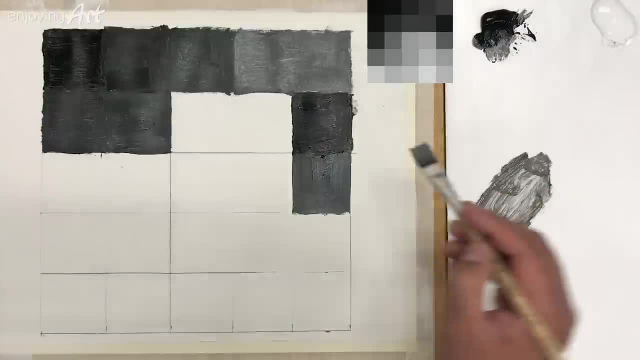 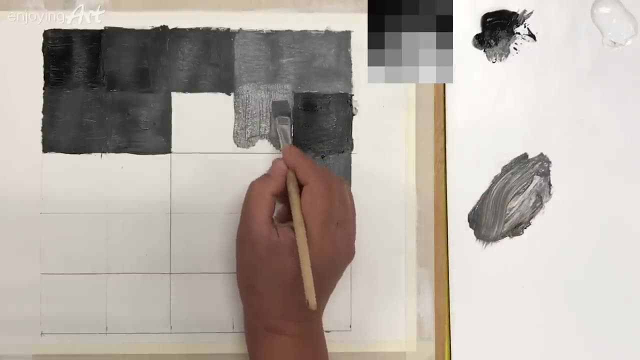 And okay, Like this, I'm going to take this color quickly, Also make it into here. Okay, Very quick Look at between this color and that color and how much difference. And maybe not enough. It should be a little bit darker. 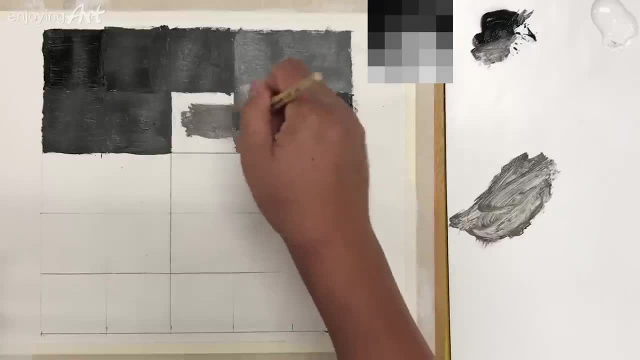 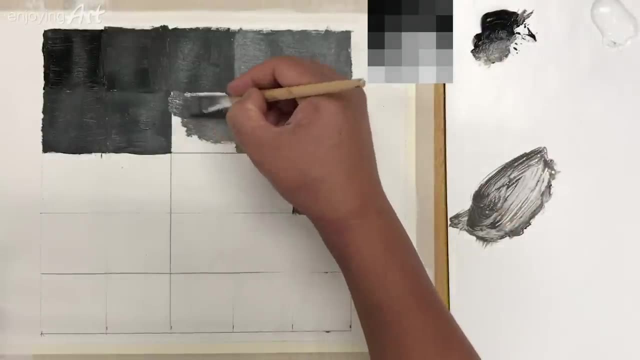 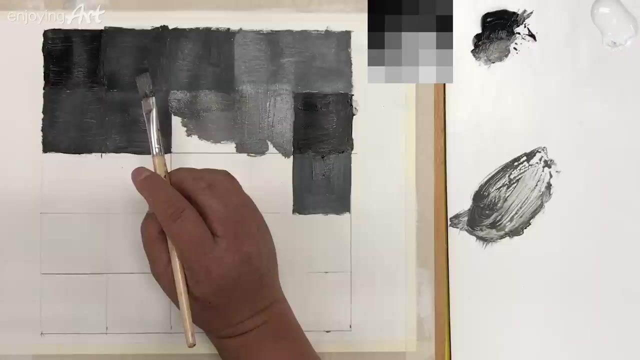 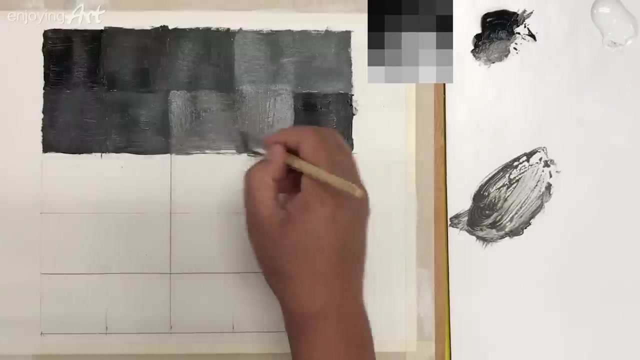 I'm going to see Make a little bit darker And go all the way over here too, But this color maybe a little bit darker, So let's see, Like this And a little bit, Okay, Continue over here Now. this color, this color. 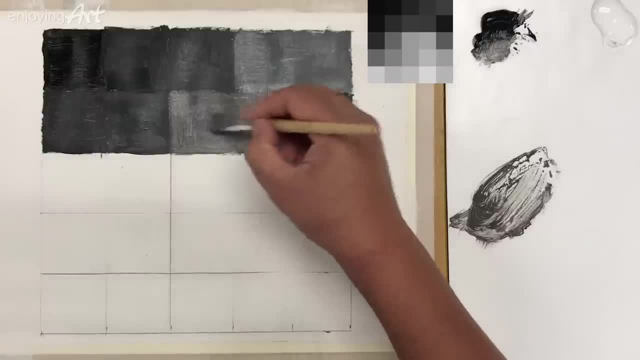 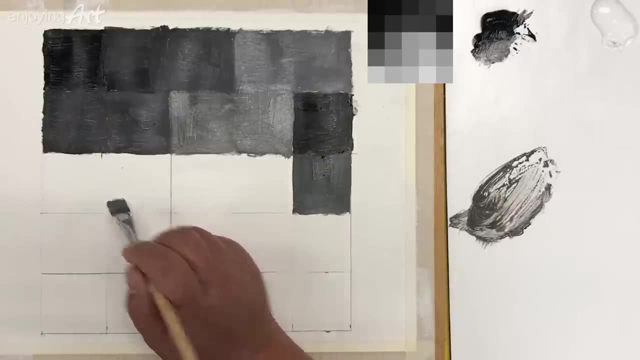 it should look similar, But now we're going to make it a little bit different. Let's see, Oh, this color also similar to this color, Right? Maybe a little bit lighter than this color. So it's easy, Add a little white into this. 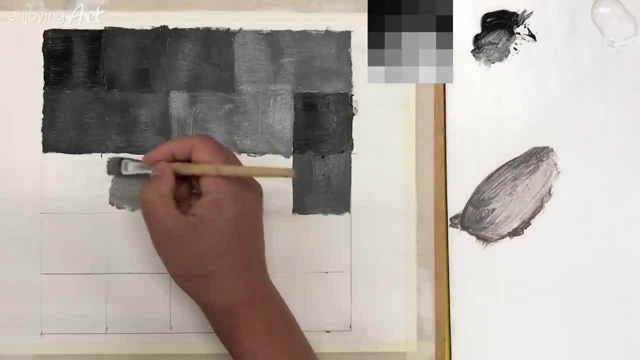 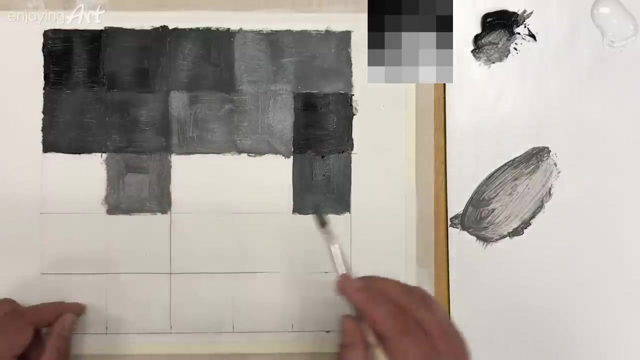 I'm going to put that maybe too much white. So always compare, Always compare. And so, okay, You don't need to be sure at the beginning, Just have to test the color, Just put it on and test it. Okay, Now I'm going to. 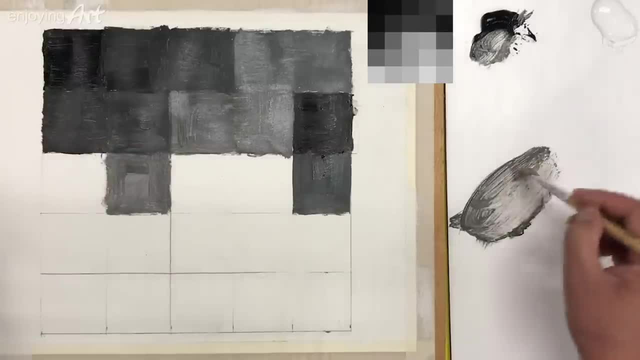 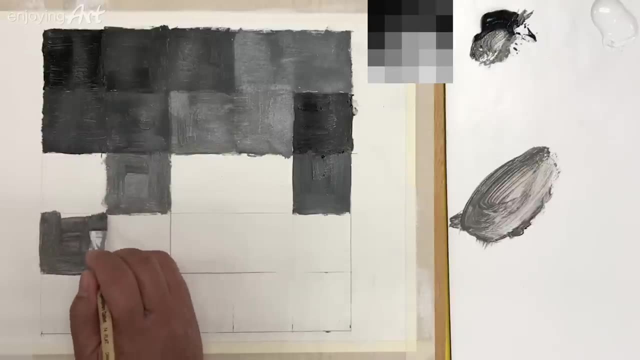 Looking for, this color Looks like a little bit darker than that. I'm going to take a little black in here And mix into this color. So this process: I expect you probably will spend a pretty good 30 minutes on it, Or maybe a little bit more. 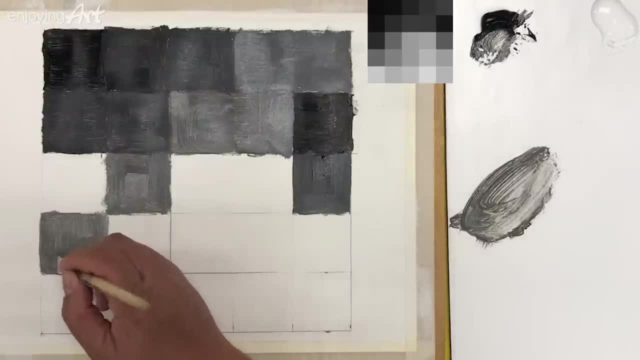 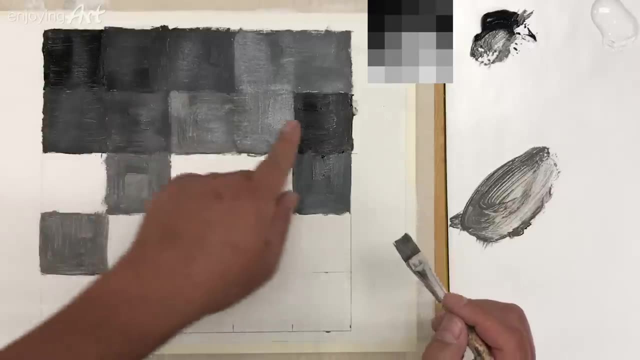 So the first round, you need to fill in all those squares before you do the adjustment. Like: this color compare with? to which color Compare? I think compare to this color And maybe this color. Let's see, I'm going to put that color in first. 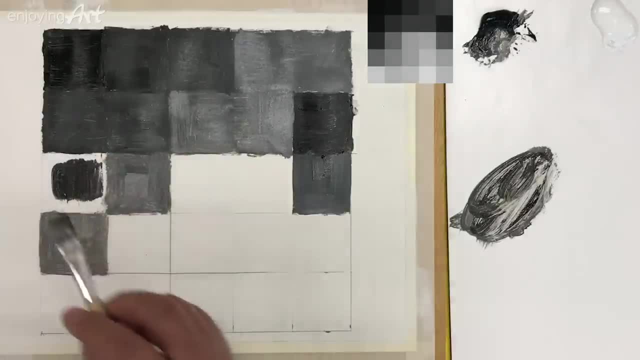 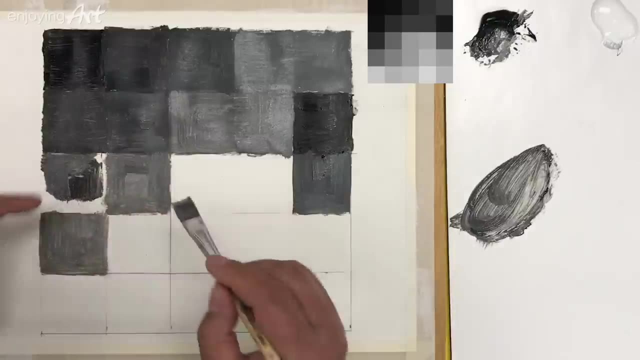 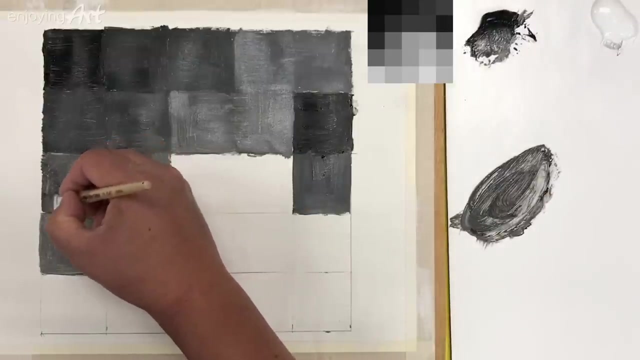 And make a little black, A little bit darker, But this color lighter than that. So I'm going to see Make a little white into this, But make sure that it's darker than this. So I'm going to get a little black color. 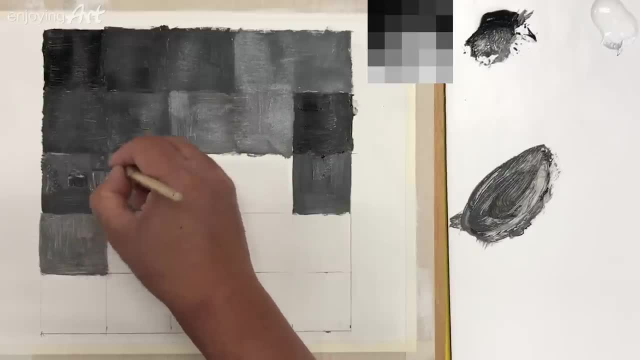 Okay, So, So. So Painting and drawing is very critical. that you Get On the habit of analyzing- It's also called critical thinking. So You don't want to? just Okay, I'm going to mix one color. 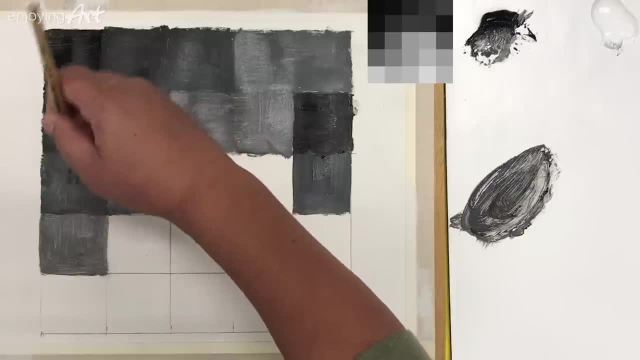 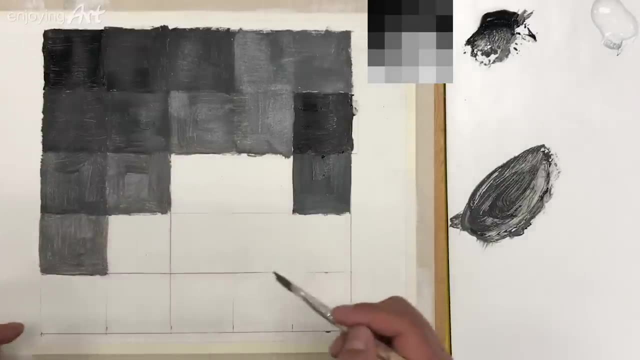 And put it over here. I don't really care how it's going to compare with other colors on the same canvas, And they're probably gonna come up with something really bad. Now those colors all look similar. Oh, it's a little bit terrible. 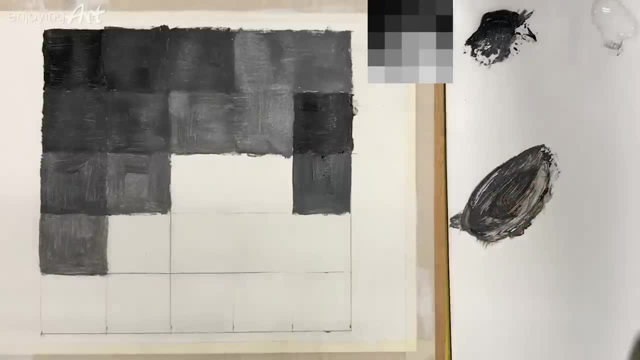 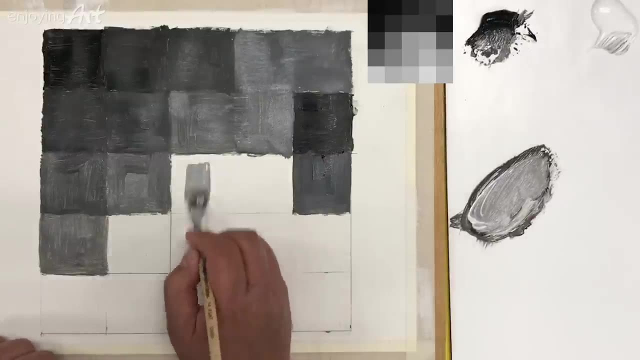 But it's okay, it's the first step. Now, the next thing I wanna do, I'm gonna mix a little bit lighter color Now. I'm gonna get a little bit lighter color Now. take a look, These two colors look very much the same. 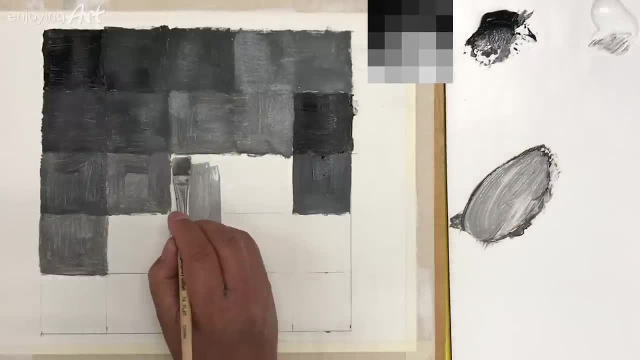 So I'm gonna blend that same color into this two square Right here, Right here, Like this, And then take a look And this color and also similar to this color, but probably a little bit lighter. So I'm gonna take this a little white into here. 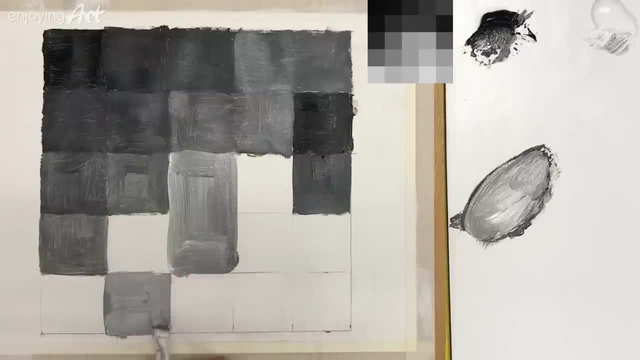 So it's very easy, But you need to have patience. Sometimes you cannot just do one stroke and then you finish it. Now take this color. Now, actually, this color a little bit darker than this color, so I'm gonna add a little black into here. 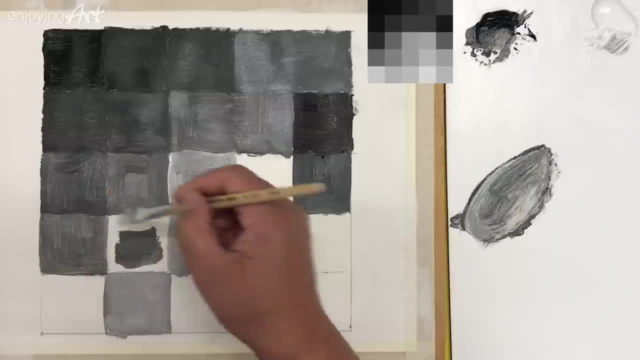 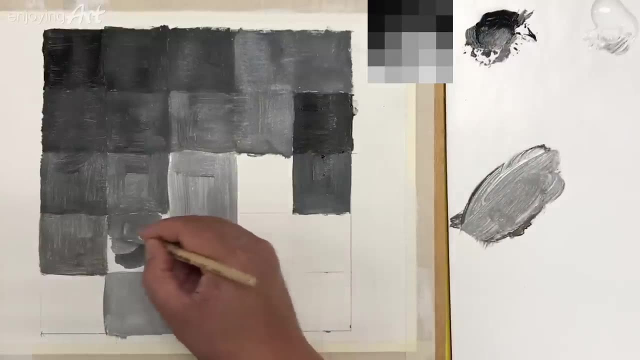 I'm gonna see, But this color should be a little bit lighter than this color. So I'm gonna see, Maybe a little bit too dark, So I'm gonna add a little white color. So make a guess and put it on, And then we're going to do adjusting. 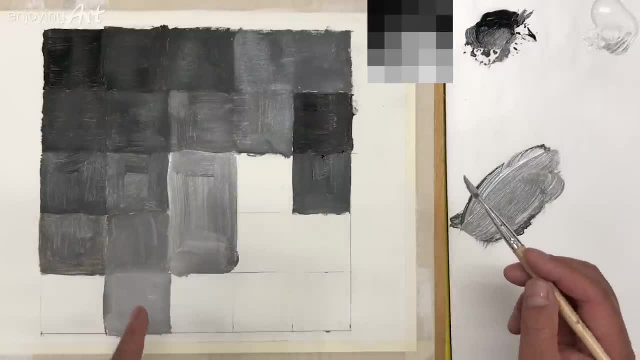 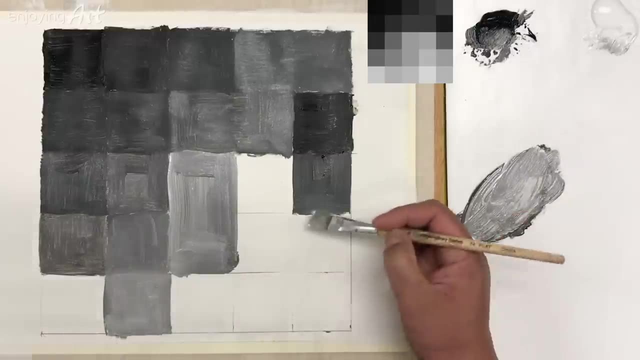 Okay, Now the other color. oh wait a minute. This color And this between this color and that color is this color. So I'm gonna add a little bit lighter and then put it here And so on. So we're almost there. 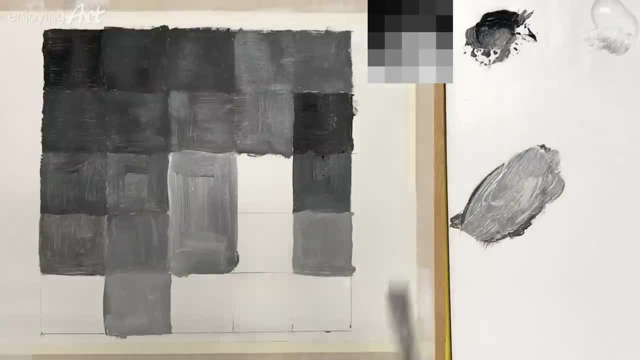 The first one. So take it like this: And now this color is similar to this color And it looks like this color already too dark, right? So I'm gonna make this a little bit lighter And maybe a little bit lighter, put it over here. 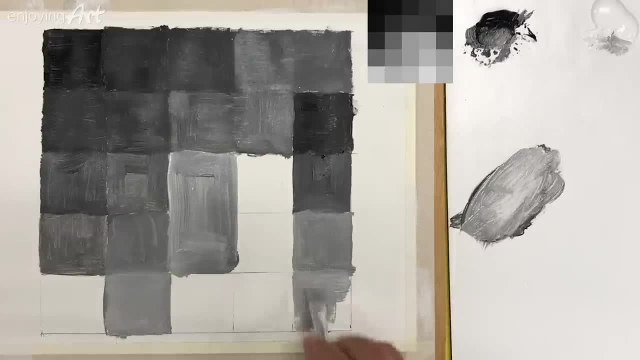 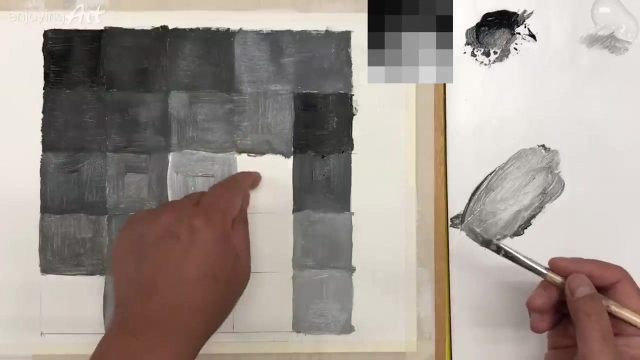 Okay, Like this- I have this color in here. Look like this too is not different enough And add a little bit white under here. Now the other color should be a little bit lighter, And this color is similar to this color, but I think this color a little bit lighter than this. 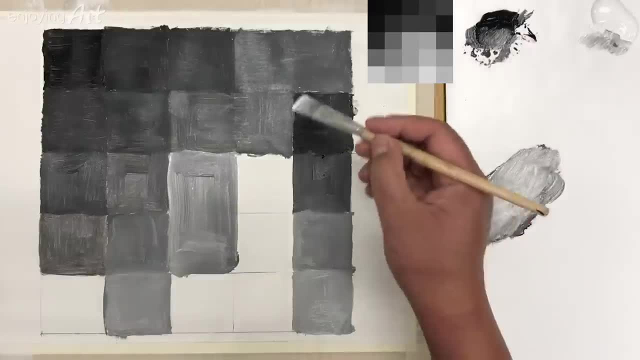 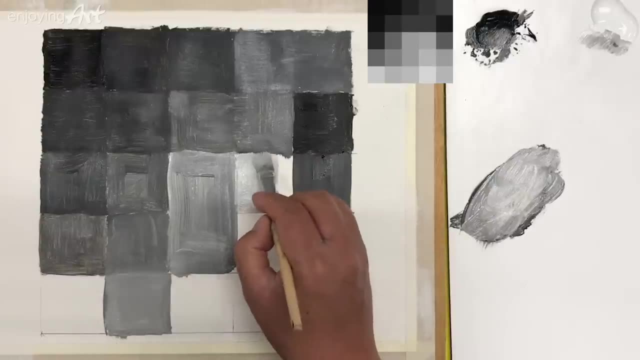 This one. So I'm gonna add a little white and then put in here And imagine if you are able to mix the color in a correct value. even just with black and white colors, you can compose a pretty decent painting together. And now what we're gonna do? this color a little bit lighter. 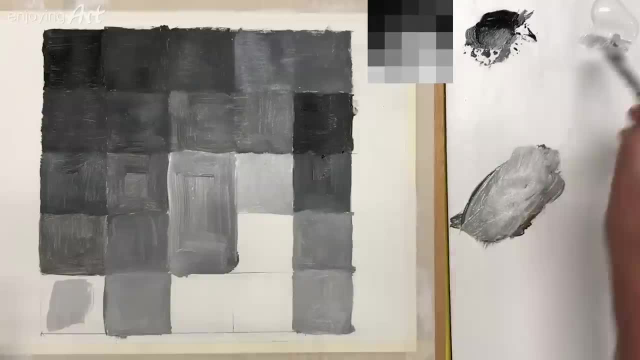 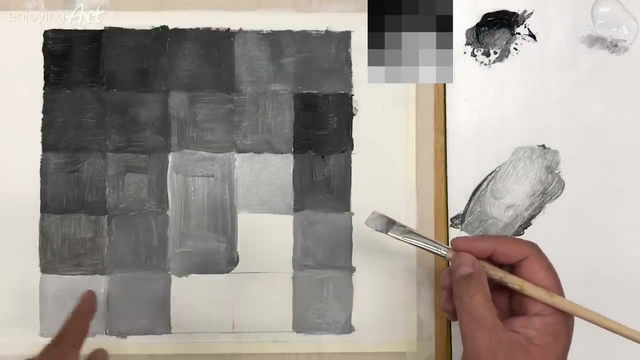 So let's get a little white, a little bit more white. Take a look, Maybe a little more, And put it over here. okay, like that, A few more squares to go. I think this color, I think a little bit darker than this. 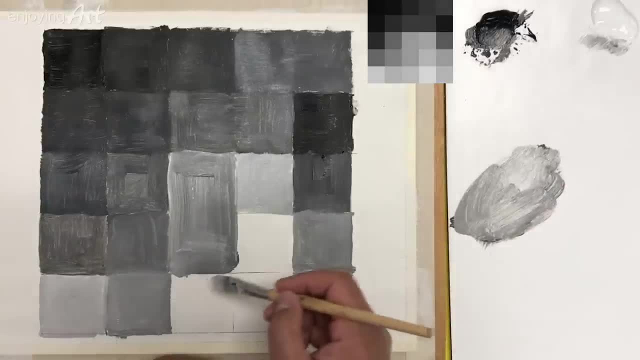 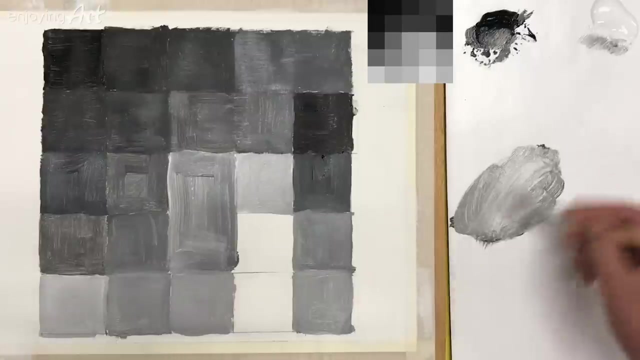 So it makes that into the darker color and put it here. Okay, now take a look between these two color. This color similar to this color, right, And let's put this color in here, But this color definitely lighter than that color. 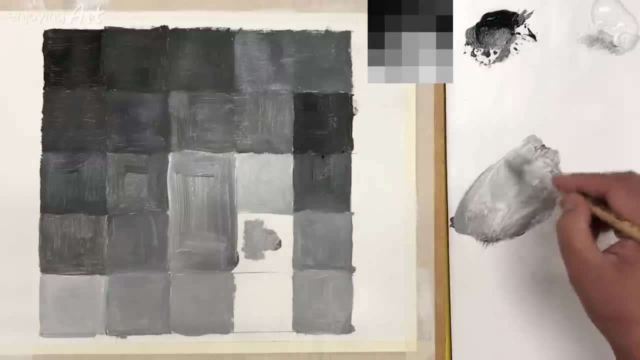 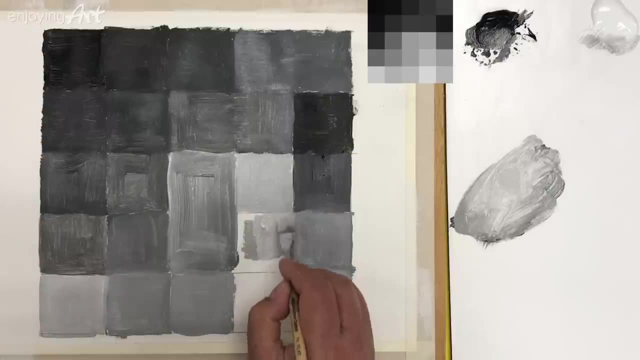 So I need to have a little bit more white color in here. Comparing, comparing- that's the key To find the value, because everything is in a certain order. Just how you are going to discover that relationship and capture it, that is very critical. 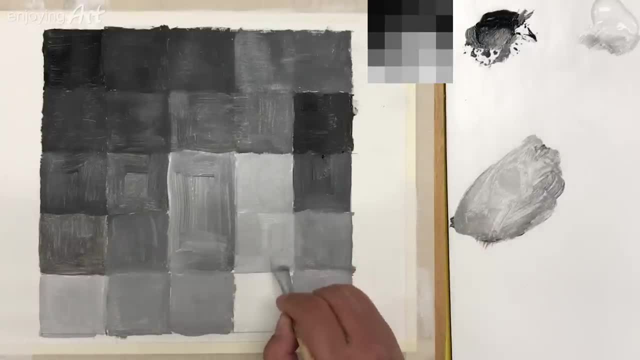 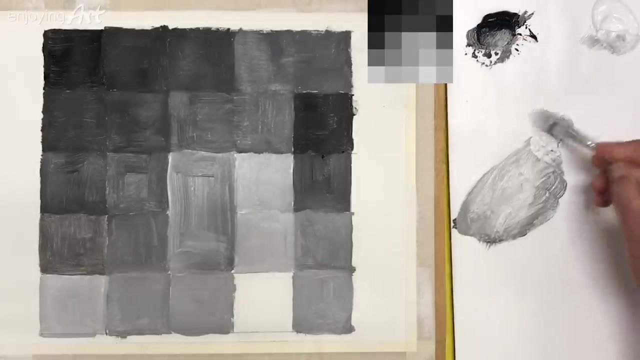 to be able to do a good painting. I think this color can be even a little bit lighter. Let's get a little bit more white. put it over here Like this: Now, this one is the lightest, So I'm going to get a lot more white. 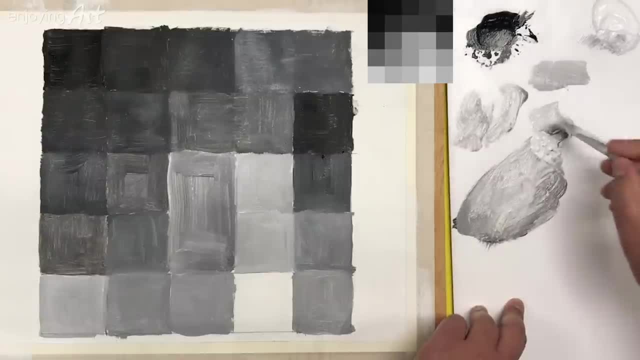 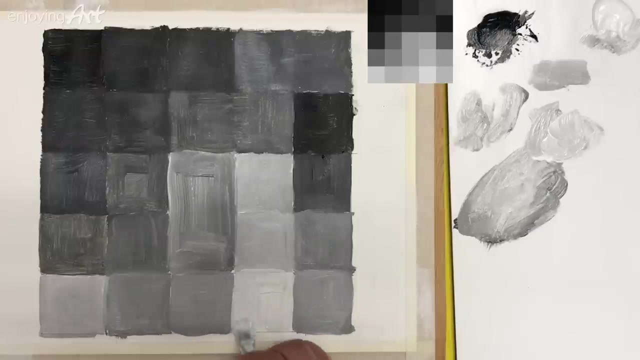 I'm probably going to get rid of most of the paint in my brush here. So just get a little bit more white. Otherwise the color just get a little bit darker and darker, And this one is not pure white, but is the lightest among all these colors. 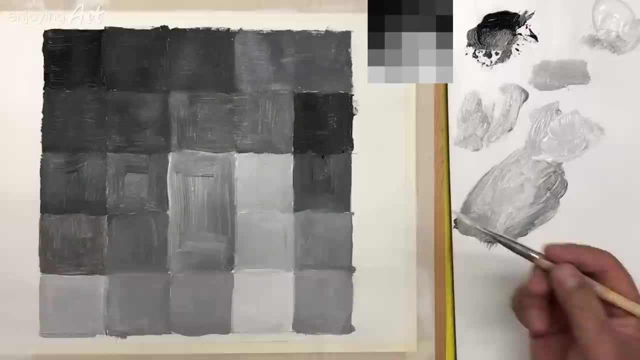 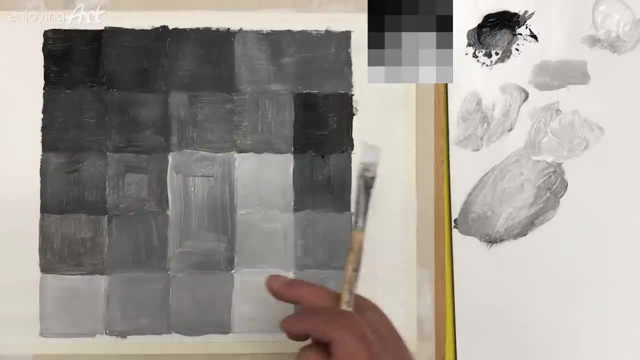 Now, that's good. Now the color also dry in everywhere else. Now let's take a look, Those color a little bit too smooth transition into this color. Let's take a look at how can we adjust it, adjust them. I think this color a little bit too dark. 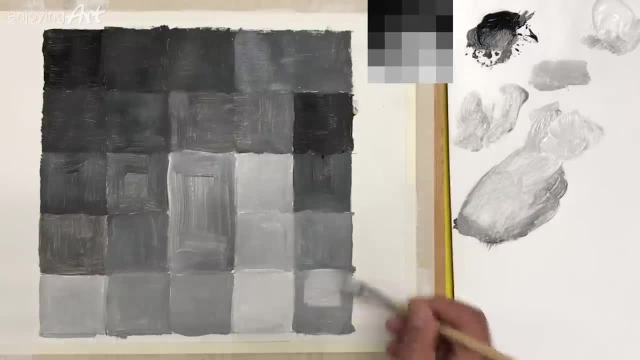 So what I want to do, I'm going to mix a little bit lighter color. Let's take a look. I think that is better. Like that, Okay, Like this. Let's take a look again. Squint the eye so you can see the difference. 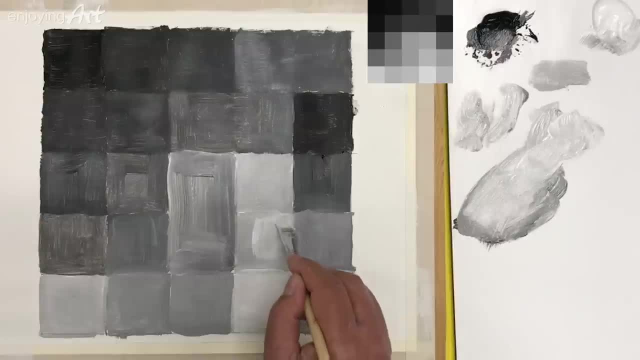 I think this color can be a little bit lighter too. I'm going to put a little white into this color And when the color is still wet on the paper, still a little moisture, it actually you mix the color directly with the wet colors. 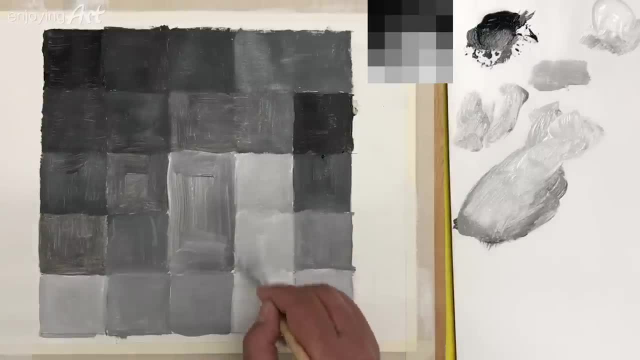 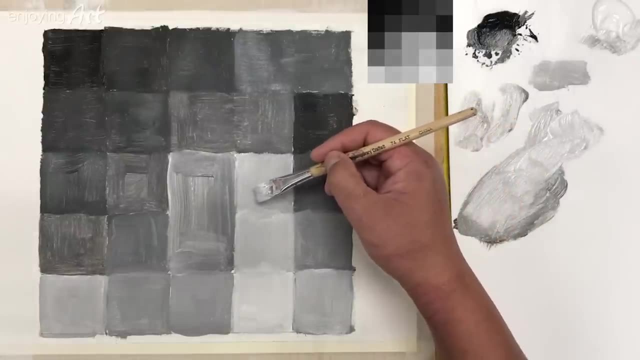 on the canvas or any surface that you use. Let's take a look. And this color now is pretty bright. Let's take a look. It's looking proper now because this color lighter than this and lighter than this and very much the same with this one. 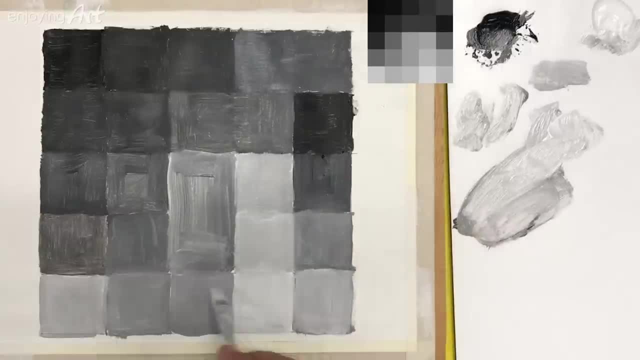 And this a little bit darker than that, So it looks like this color should be a little bit lighter. So when you look back to my videos painting a portrait, it's always comparing. It's the same exact process process, but this one is just a little bit more simple than dealing with complicated 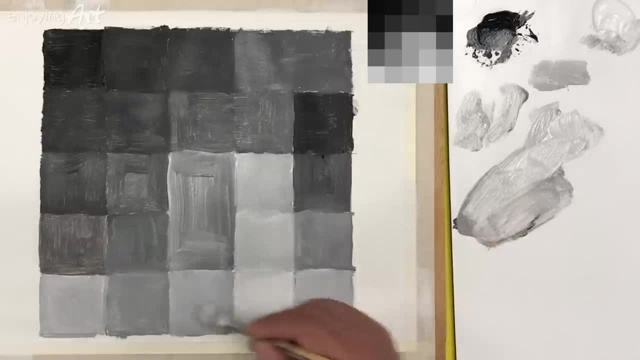 objects. So this one is a little bit lighter. Now feel a little bit better between these few colors. Okay, now we're going to continue. I think this color now, after it dries, looks a little bit too dark. a little bit I'm going to mix a little bit white into this color. 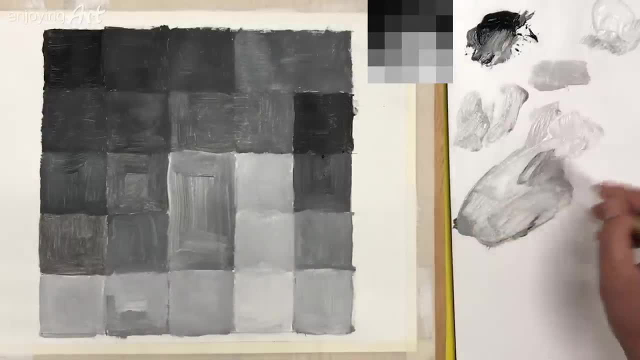 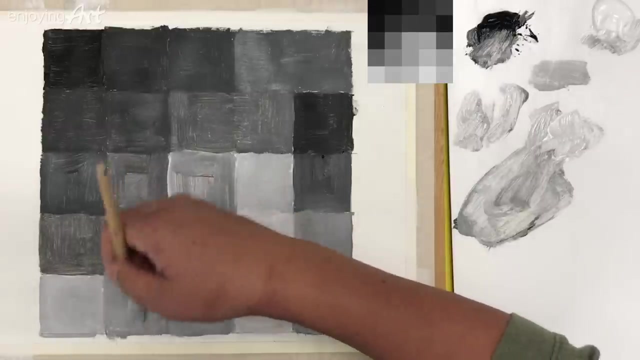 And now it's a little bit too light. probably Get a little bit dark color in here Now. blend it in Now this color, a little bit better. I think this will be better. I think it's proper Now take a look. 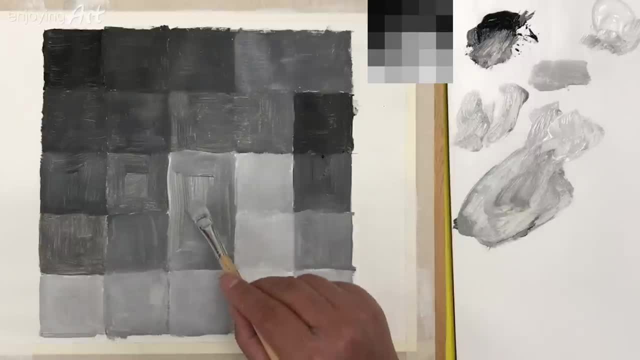 This color. can you tell me? this color is too dark or too light? A little bit too dark. You're right And I trust you. Okay, Now I put this color. Oh, this color looks pretty good And I put in this one shape. 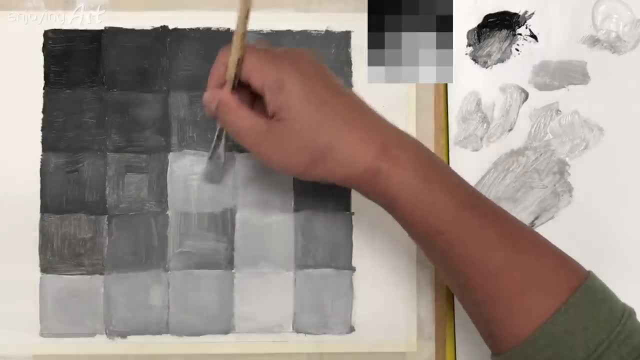 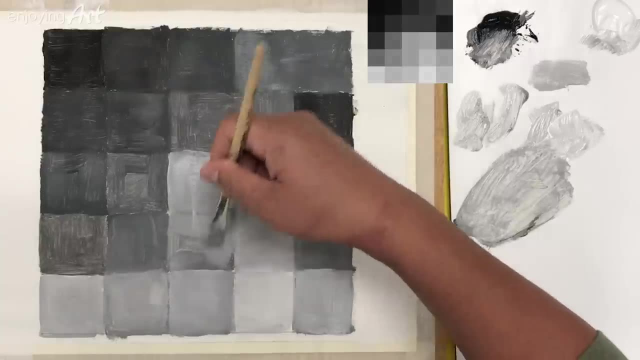 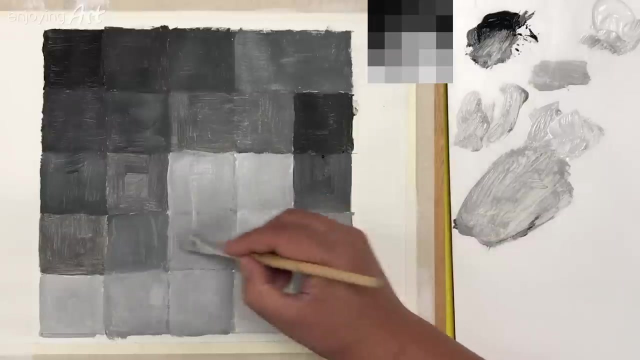 This is good right Between these two values. it's a very proper connection, And I'm going to put it in here too, because these two colors are very much similar, almost the same, like that. This is good, And the color get look a little bit thicker and then it look nicer. 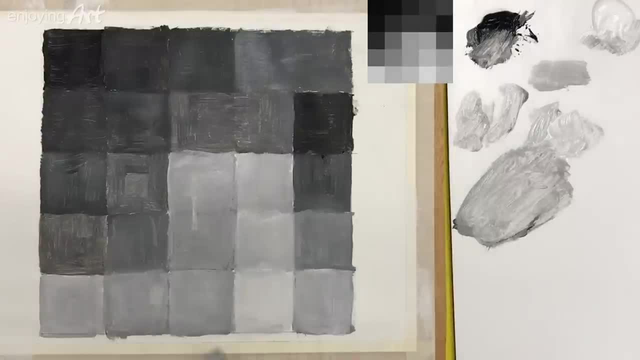 Okay, Now let's continue. How about this color? Hmm, It's very much there, this color. Maybe this color a little bit darker than this, but hard to say This one. Probably it's just a little bit darker, but it's not that much. 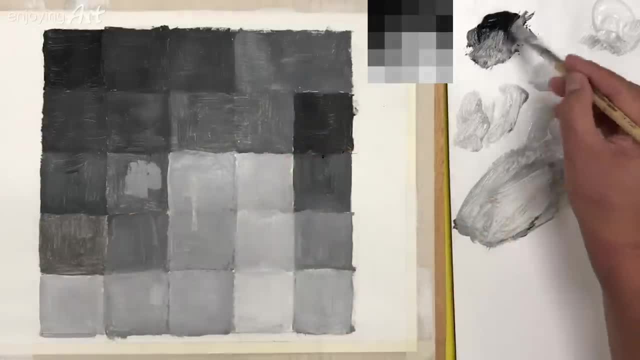 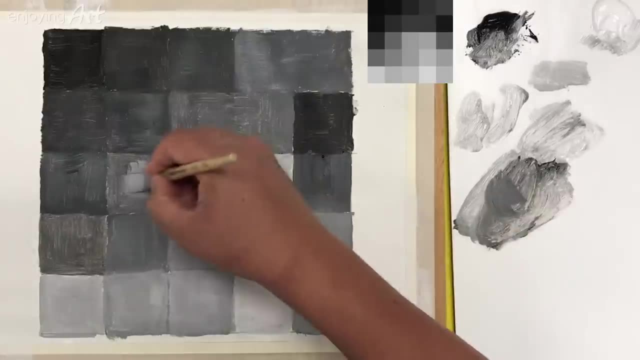 I'm going to see, I'm going to make this color ooh too light, right? So you're going to mix the black color with the white and test it. Oh, better, Good, Now we're going to put this color in here. 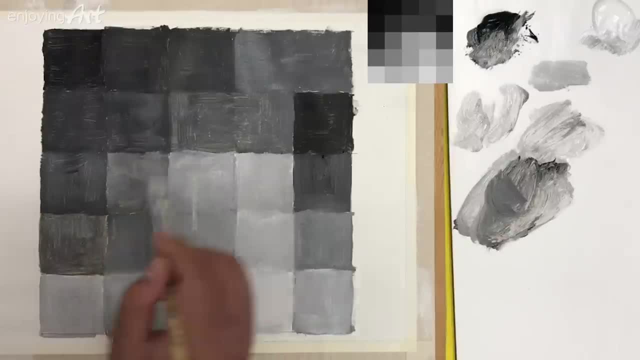 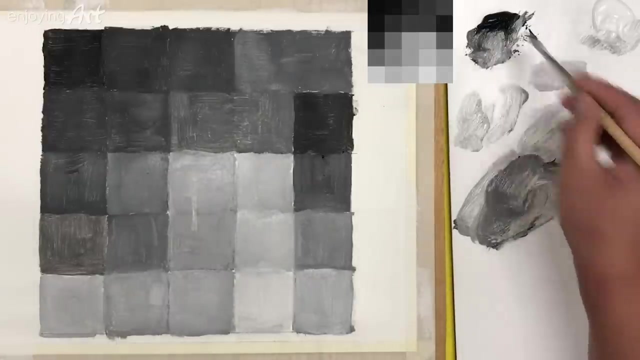 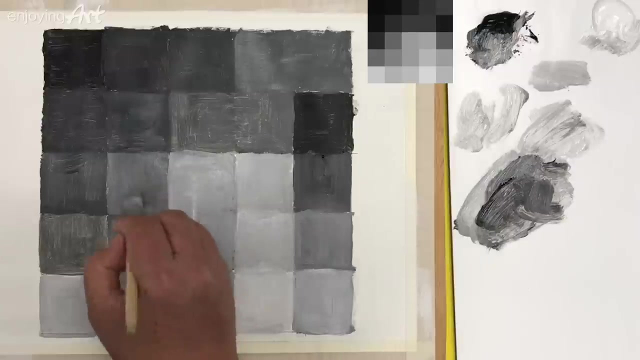 Put it over here. You got to have patience. okay, Especially in the future You could be a doctor. Okay here, And this one: I think if this color proper probably a little bit too light, Get a little dark color in here. 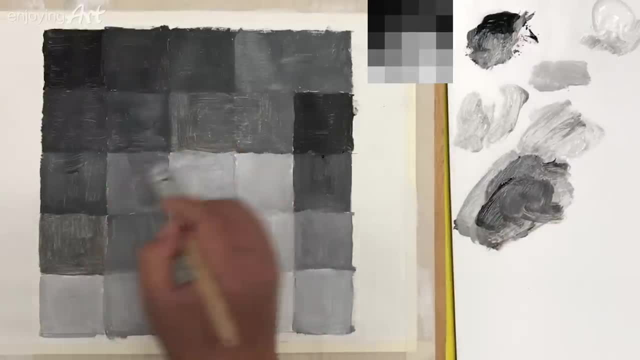 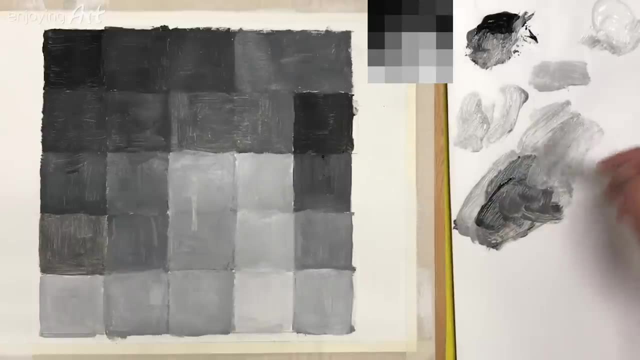 Yep, Probably better. Okay, But this color definitely need to be a bit lighter, So I'm going to take the light color mix into here. Let's take a look. Yeah, A little bit better Test it And it's just the right one. 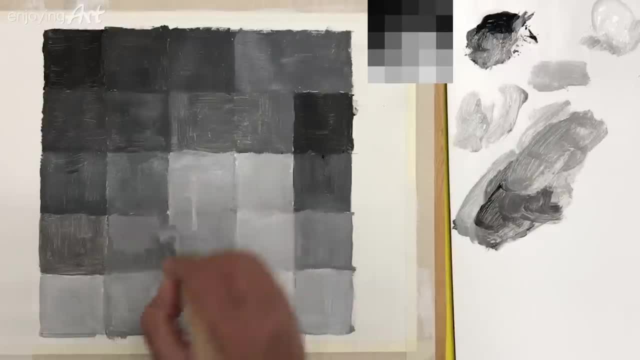 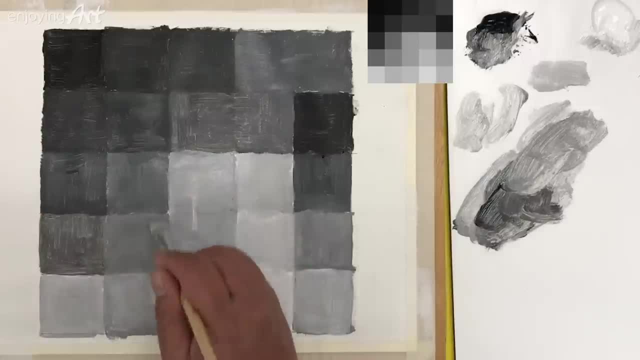 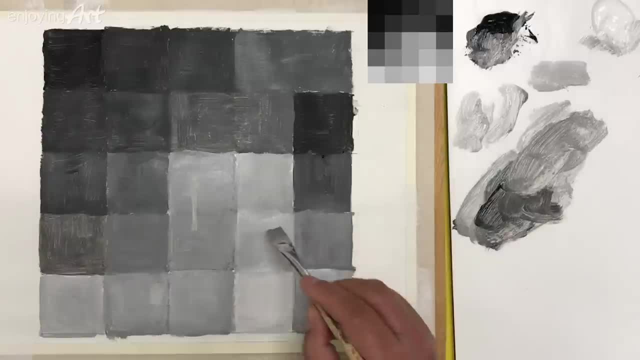 Okay, And take a look. I think this color. now, What about this color? This color? probably okay. Like this color. compared to this color, it's probably okay. Now I'm going to move on. I think this color is fine. 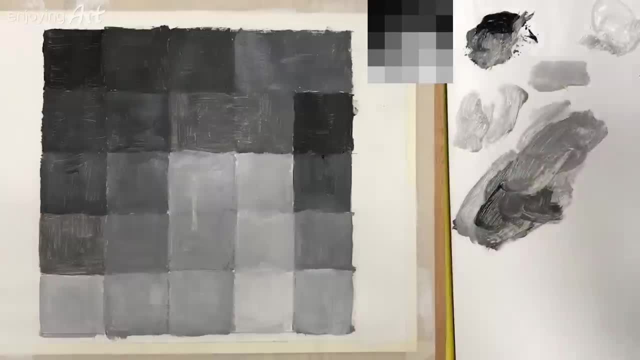 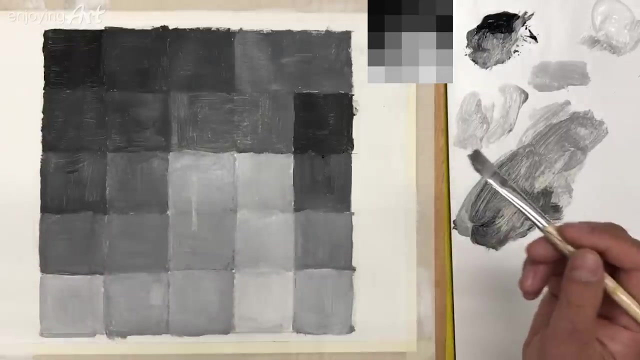 But this color should be similar to this color, little bit darker. Now I'm going to retouch into this color. Let's take a look. Is that a little bit better? Actually, that's already better Like this. No, Now it needs to be a little bit darker than that, So I'm going to get a little. 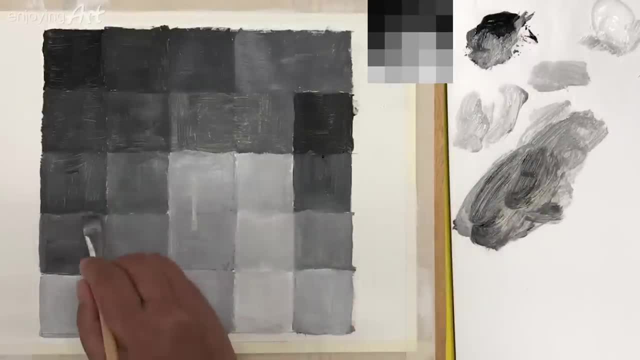 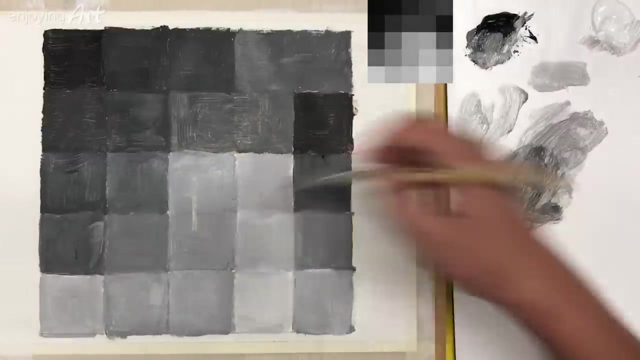 bit black color and mix it in to this square. So that's good, Let's take a look, Let's go around and the edge over here is not much sharp, so you can actually. you want to see a little bit clear and you can put the color right. 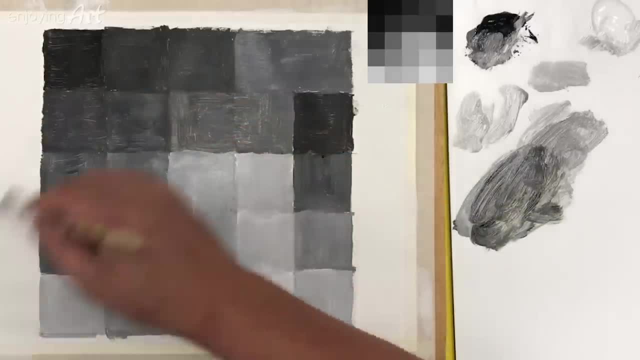 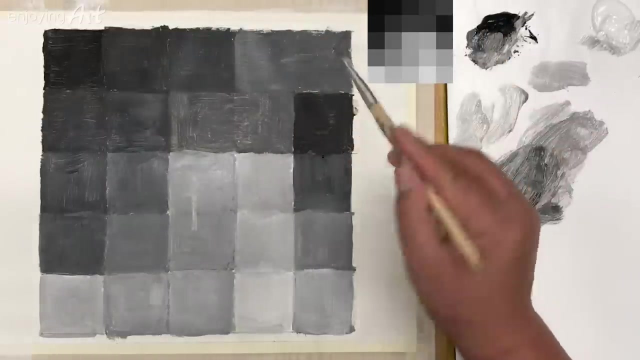 next to this. That's good, But you want to see the overall, the whole color and how it look like. And this color probably right. Okay, Let's move on And let's take a look at those color retouch. it Is the color a little bit too thin. I think this color 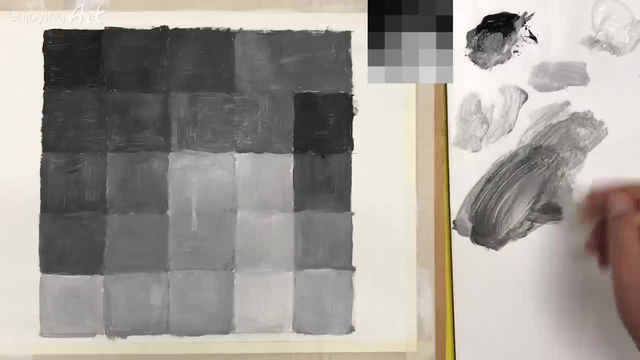 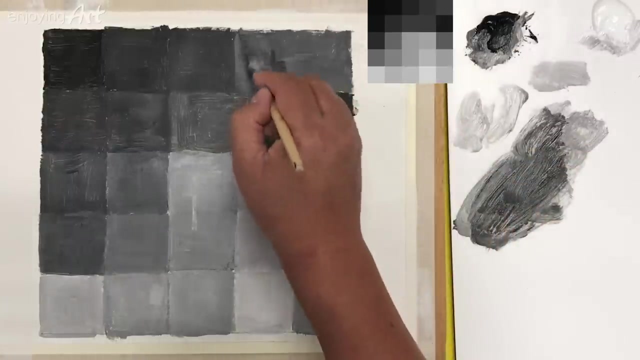 can be a little bit darker. So I'm going to take a little water to mix the color, Get a little bit darker, Darker. Let's see how dark the color supposed to be in this color And I think this color is a little bit darker and should be a little. 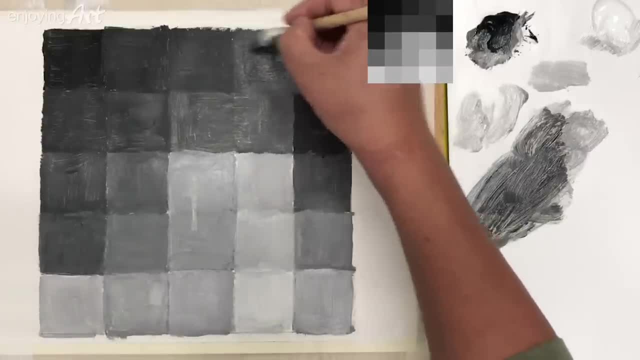 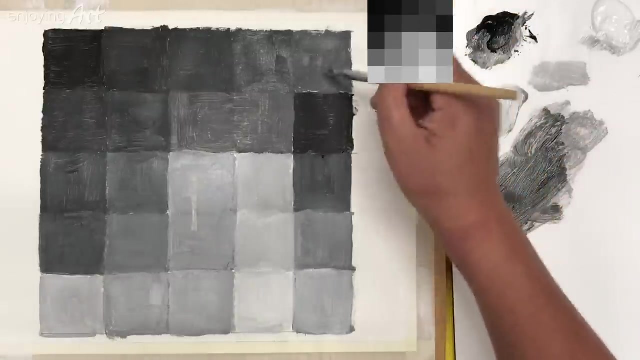 bit darker, Like that. I'm just showing you the process As you practice this, analyzing colors, and keep practicing and you're going to go faster and faster and maybe faster than me, And in that case you can finish a painting faster And this color is very much in the right tone. 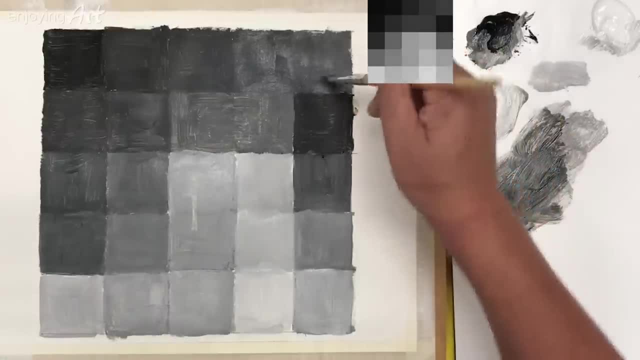 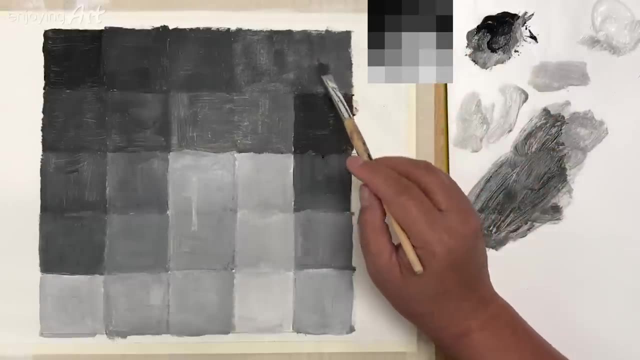 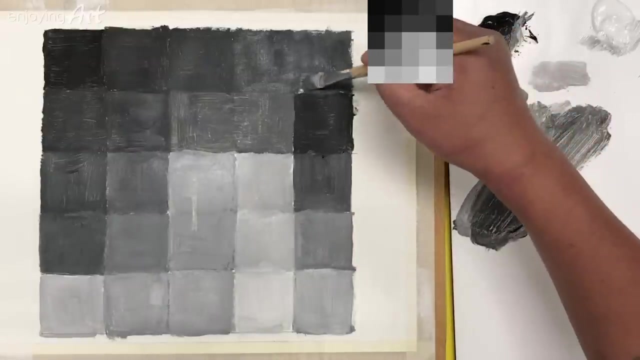 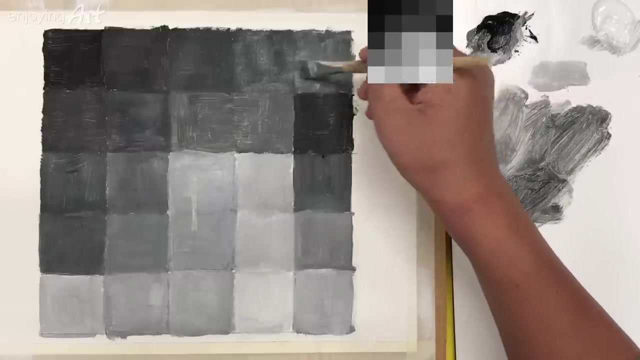 So let's see And compare these two colors. And this color a little bit lighter. So you make a choice: Either this color should be a little bit lighter than this, Or this color needs to be a little bit darker. Yeah, Let's see A little bit lighter. Let's see how it. 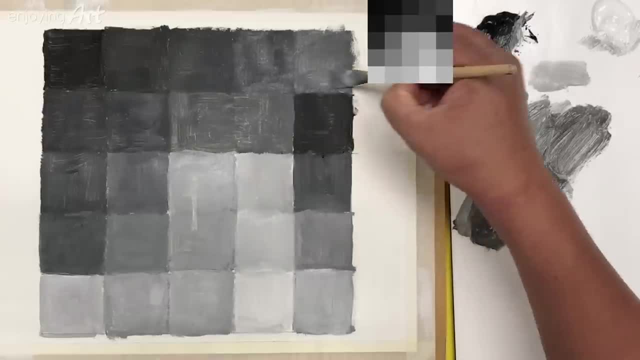 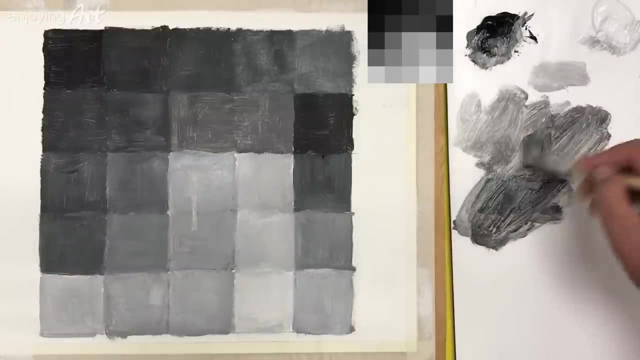 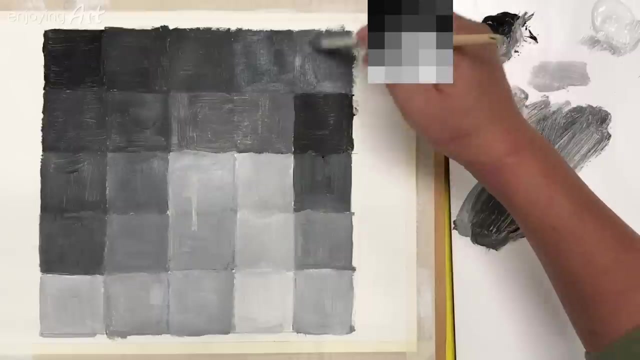 look. After it dries, you can see the true color. And now it's very much dry And let's see, I think it's a little bit too light. I'm going to mix a little dark color. Let's put a little dark color in here And I'll enjoy it And just say, okay, I beat myself. 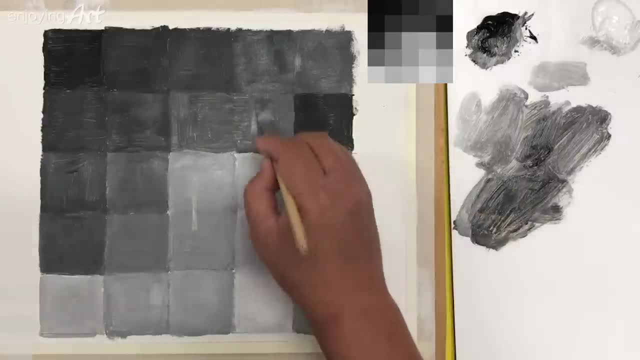 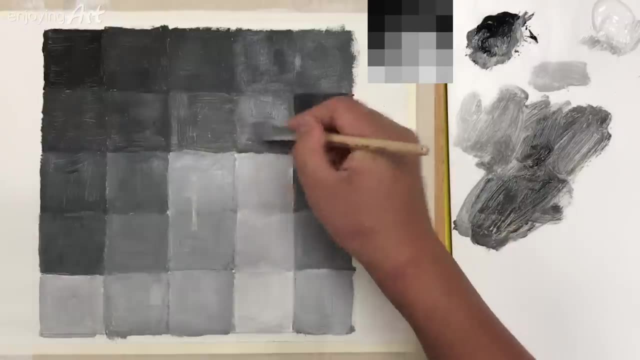 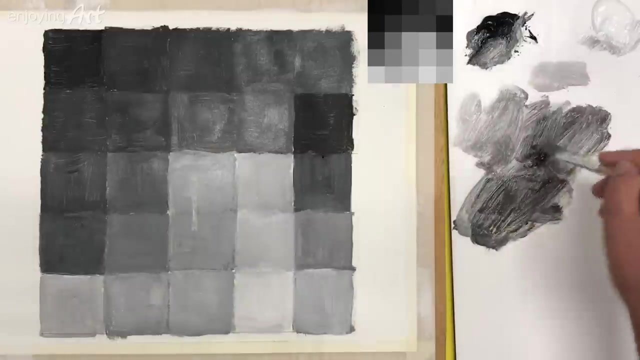 I got better. That counts right. Okay, I'm going to make this almost the same color, Just maybe a little bit lighter than that. Let's see, Like this, This color will be better. It's very similar, And this color actually a little bit slightly darker than this color. 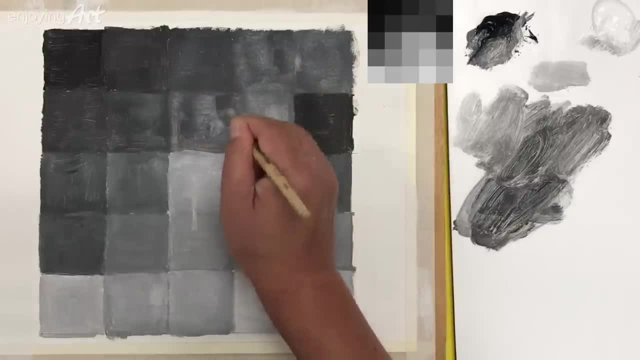 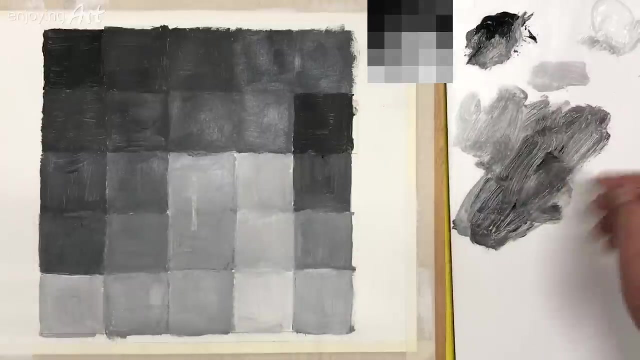 And I come in to pay more attention to the smaller contrast. Okay, I'll put it over here. I'll take a look And this actually a little bit better. Now I'm going to left over this color. I'm going to make it a little bit darker than this. Okay, Mix that. Okay, Yeah, Right. 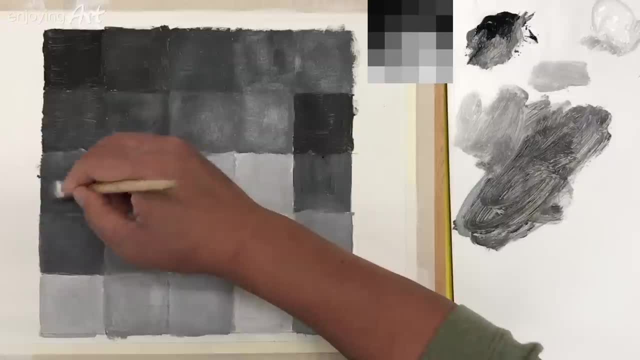 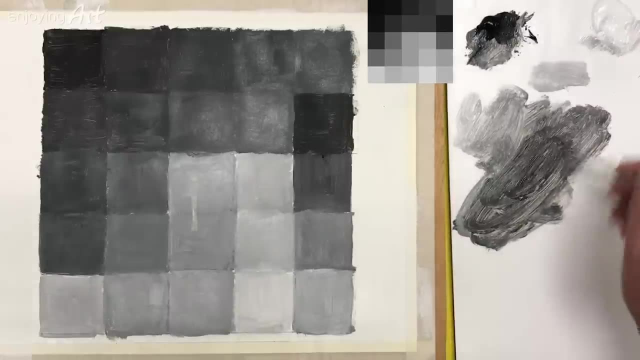 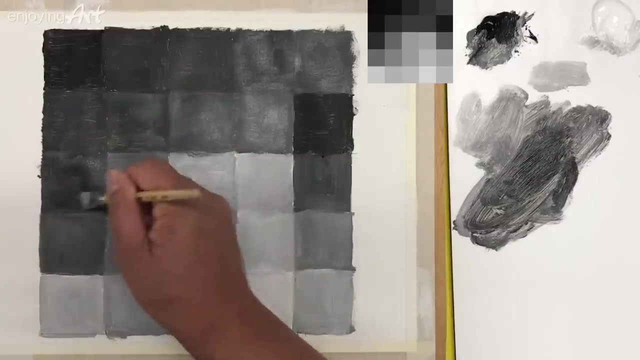 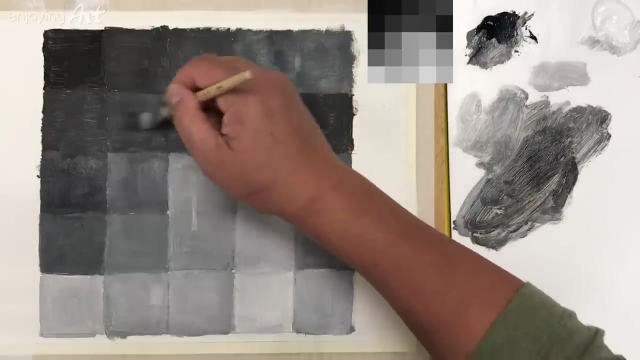 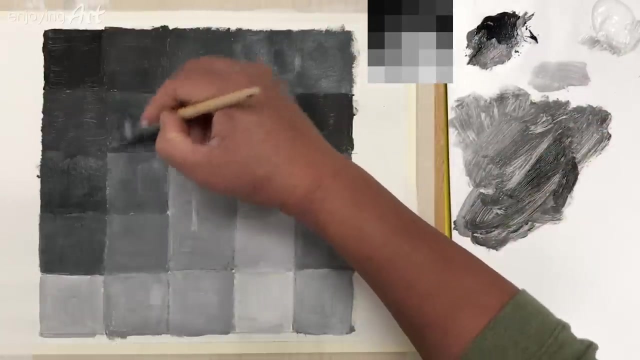 A little bit darker And maybe a little bit more darker. Okay, Like this. Now we're going to continue This color. very much, right, This color, and this color a little bit lighter than that color. So mix a little bit white into this color. So now let's see. 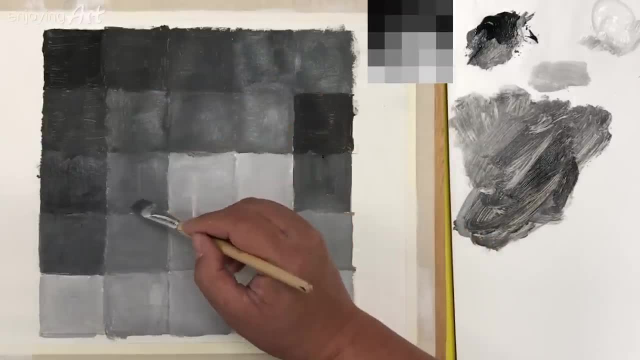 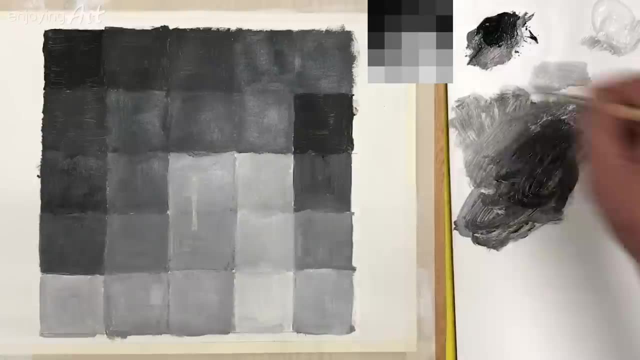 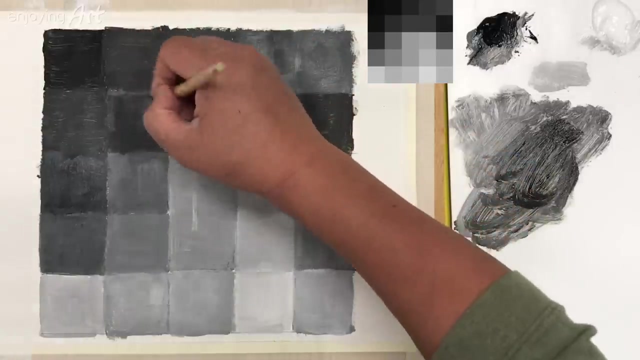 This color should be much darker than this. So it looks like that And this color looks like the right tone. So now I'm going to make a little bit change And it should be a little bit darker. So, kind of comparing two or three colors together, you can find the connection. That's I call. 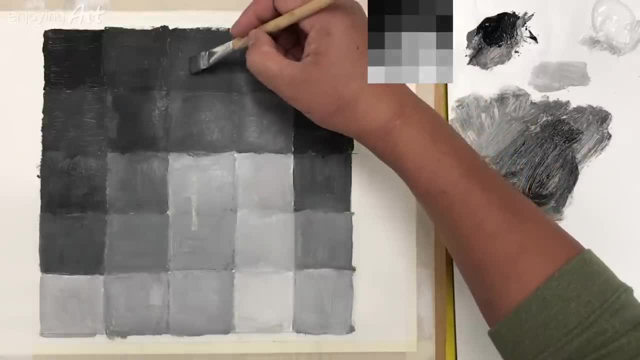 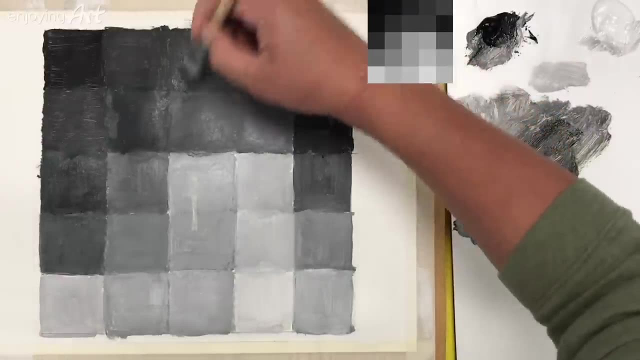 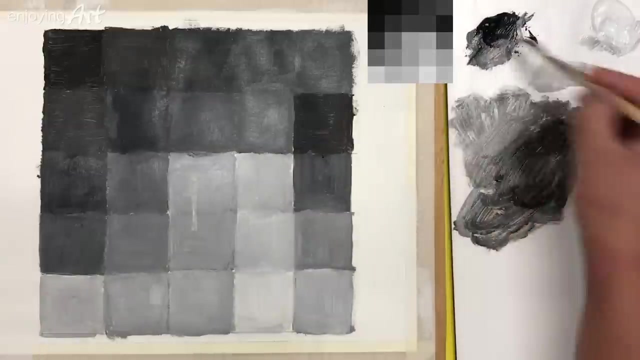 this connection. I think this is good. Now, this color is similar to this color, but a little bit darker, So I'm going to make it a little bit darker, Get a little bit darker. coming over here, Here you go, It's about right, and slightly a little bit darker because you can see a bit darker than. 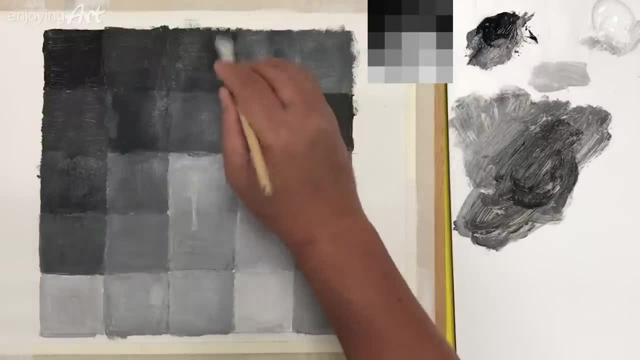 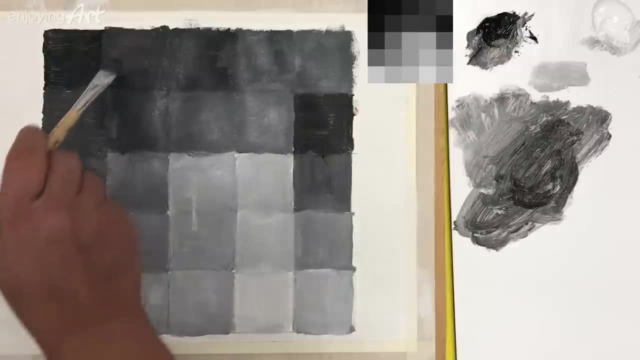 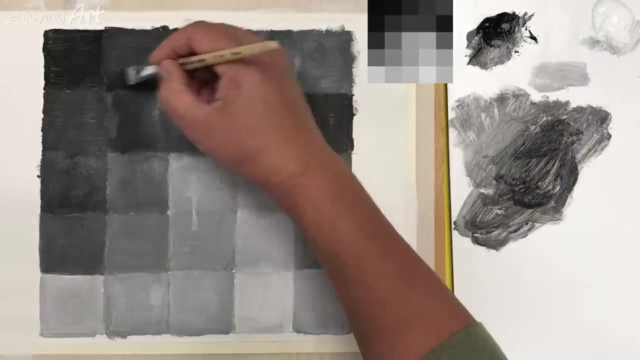 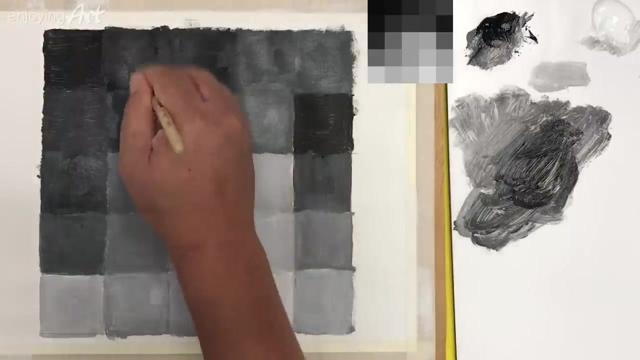 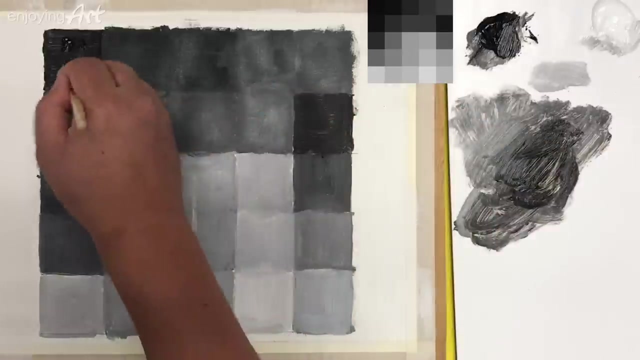 this color. Right, That's good. Now we come here. This color darker than this color. Now I am mixing a little bit more black into the mixture. Now this color should be a little bit darker, Like this: Now this color is the darkest. I'm going to just put the black color in here. 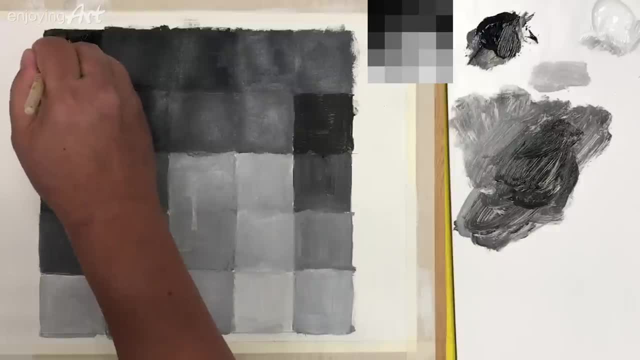 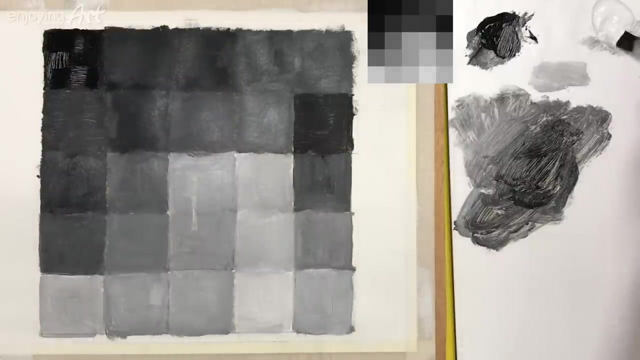 Make it a little bit thicker, Make the color a little bit better. This is dark, Okay, Let's see. And this color is just a little bit lighter than this. I'm going to take a little white, Not too much white, Okay, I'm going to make this color. 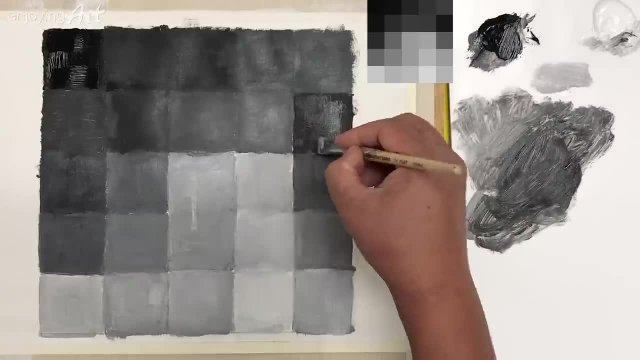 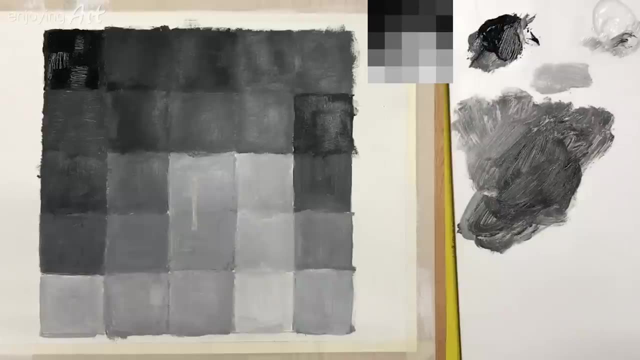 look a little bit nicer, A little bit thicker. Sorry, This is my second run. The chances you have to do another run. Okay, You're feeling kind of, oh my god. Okay, It's okay. So now I think there's the white color here, The lightest color, need to be even lighter. 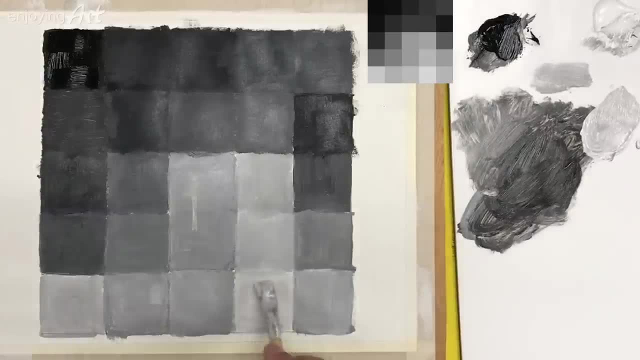 So I'm going to just take this, I'm going to put it over here And still have too much, too much black in the brush. So you need to totally clean it as much as you can And just take the white color in here, Make it a little bit lighter. I want to show, Thank you. I. 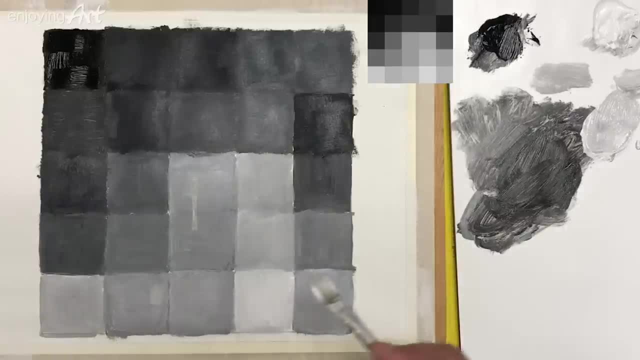 want to show you, I want to show this to be the lightest spot, And now I look at here: A little bit too, a little bit too dark Should be closer to this value. So I'm just going to put a little lighter color, A little bit lighter, Not as 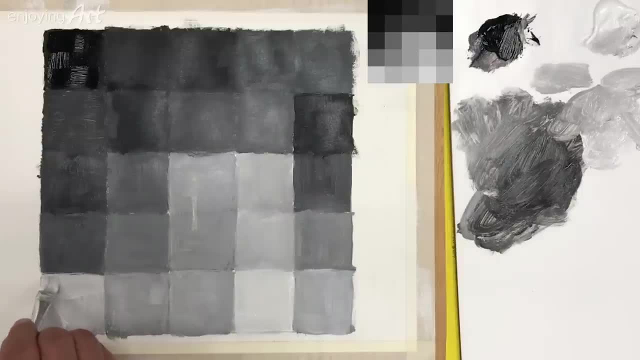 light as that color, So and so on. So you can do the number three run And number four run, And also at the same time, if you're doing a portrait or landscape or still life painting And you're going to get into more and more and more and more details, A little 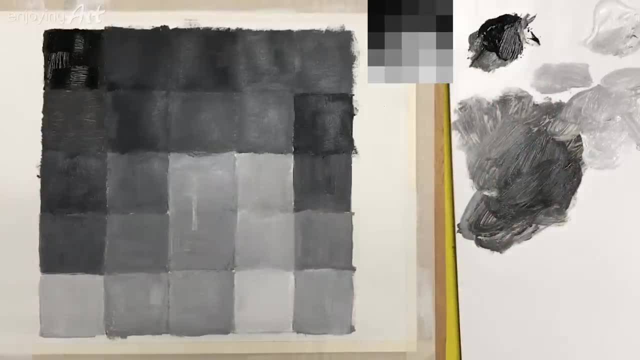 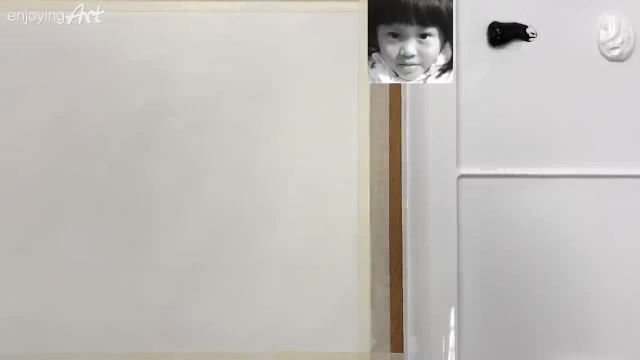 bit smaller and smaller differences And you're analyzing speed, Faster and faster And you become a good painter. So I'm going to use the same analytic techniques to paint a portrait- Black and white, Two colors- And next week we're going to learn to color. But we have to see the different value between. 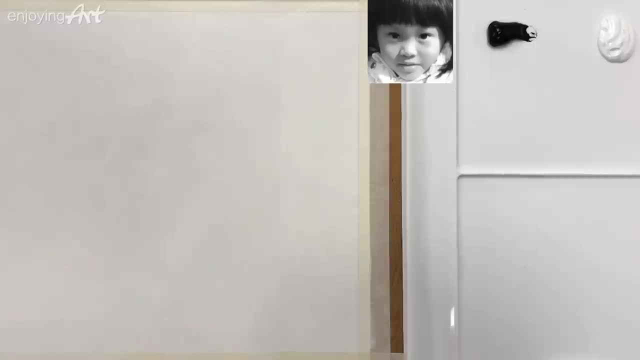 those colors In order to pick different colors. Okay, The first thing I like you to do as a homework, I want you to draw it with a pencil. Draw the area, Like the face over here, A little bit rounded. Coming over here, The hair is about this much on the top, So use 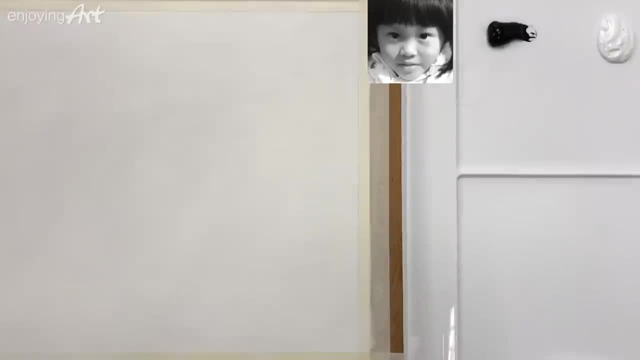 the pencil, Draw all those details. It might take you 20 minutes to do that. So, because, unless you have a really good drawing skill, Just directly paint. That's fine. This is what I'm going to do. So the first thing I'm going to do I'm going to use a larger brush. Okay, Mine is probably. 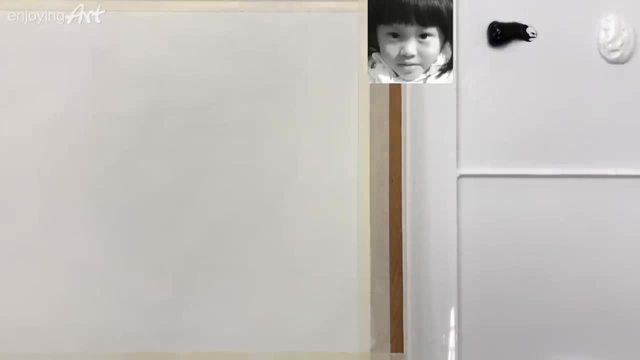 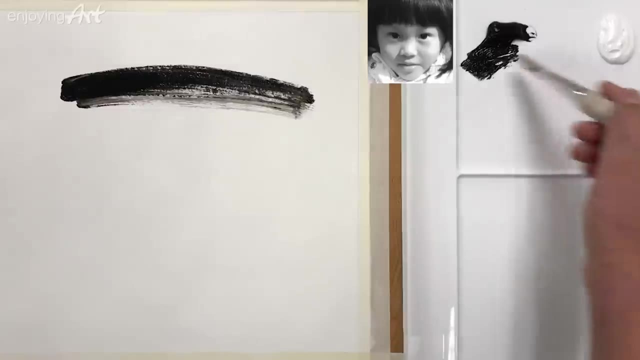 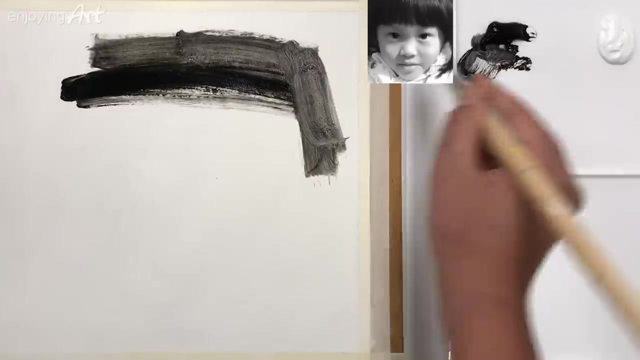 number 12. Or even larger. What I want to do now? First, I'm going to mark the whole area over here. I want to see the big area before the smaller area. Okay, This is the dark color I'm going to see. So the face with coming. 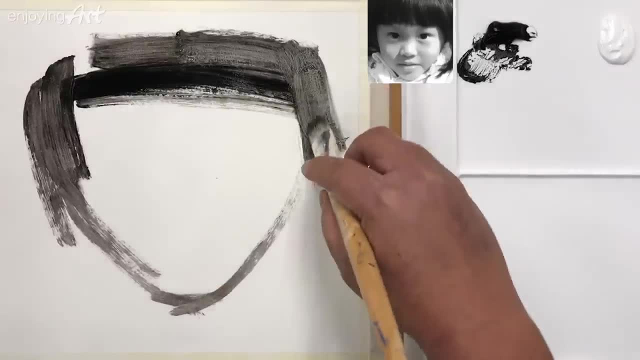 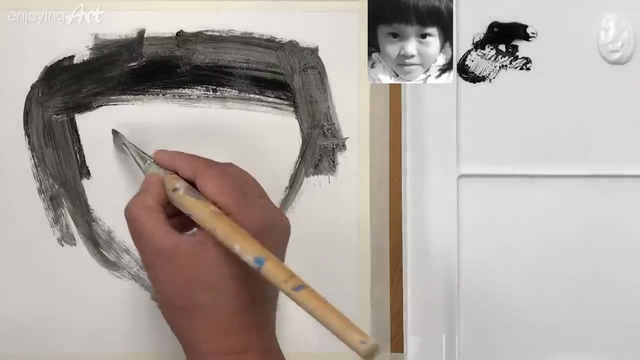 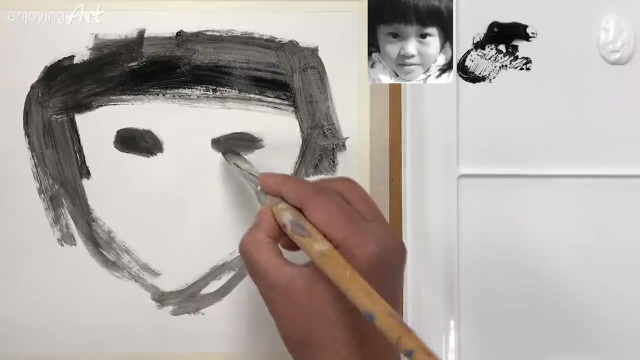 over here Like this And come up Right, You can use the graphite pencil. Do the same thing. Like this, And the eye- It'll be the two eyes over here, Like that. Well, you might be thinking about wait, wait, wait, wait. What about inside the eye? No, 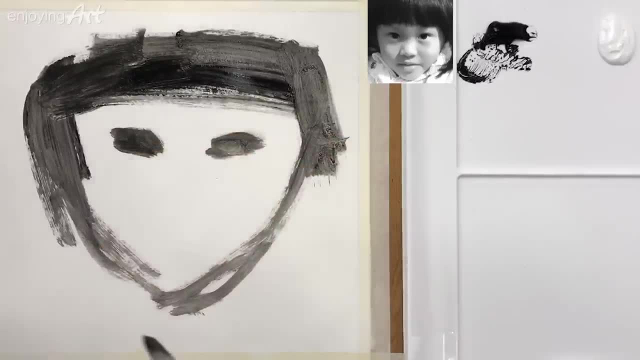 We're not thinking about the smaller area, We're thinking about big areas. So you have to make sure you're in the correct process. Now. the nose over here- That's the nose area And actually you can see they catch the shadow from the nose over here. 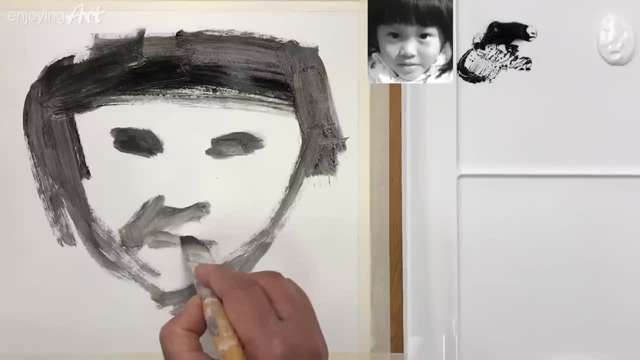 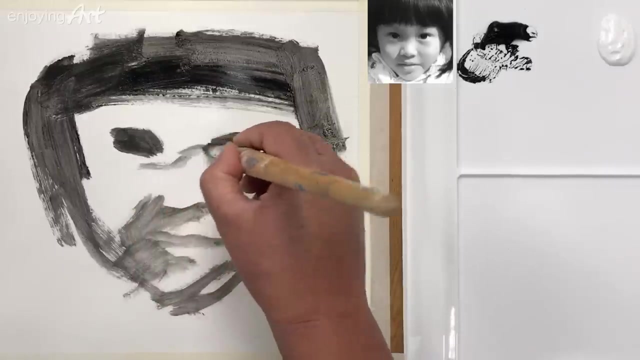 And what's the mouth? The mouth is about here. Like that, Spend some time, Draw out with the pencil Or with the brush And on this side have a little bit soft color. Okay, Of course, on this side it has darker color. You see that You mark the area. 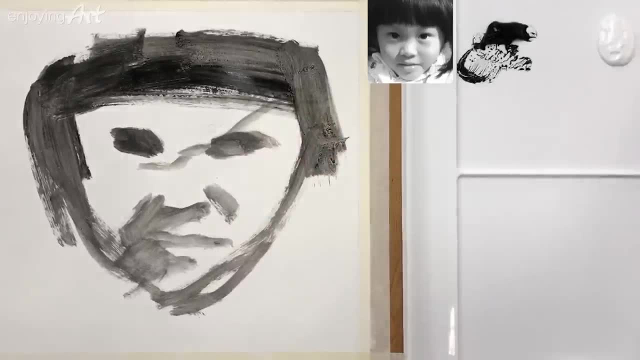 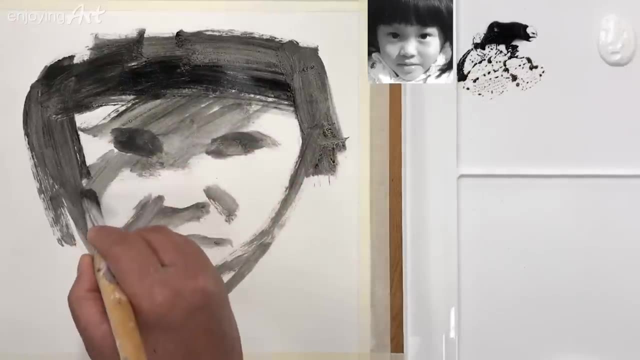 There's a little bit in a similar value. You ready, So I'm going to put the similar value over here. You see that This is the similar value, So you can see the positive space and negative space. You see the negative space over. 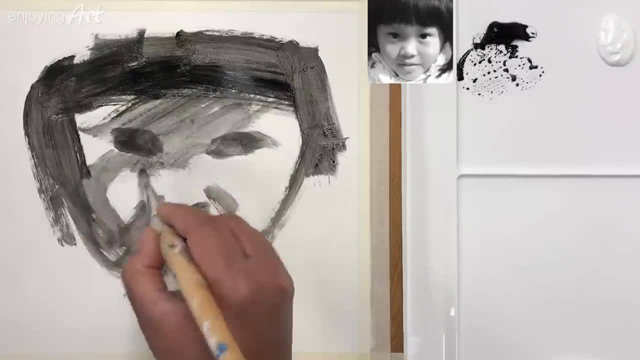 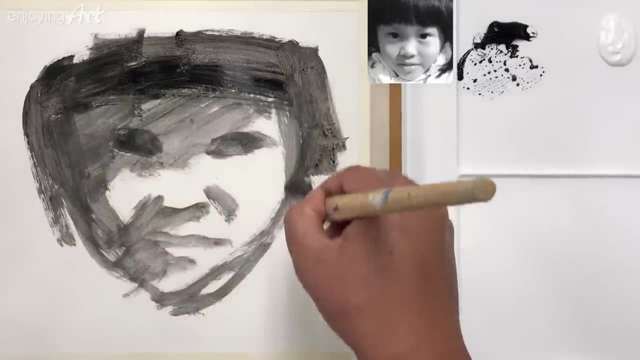 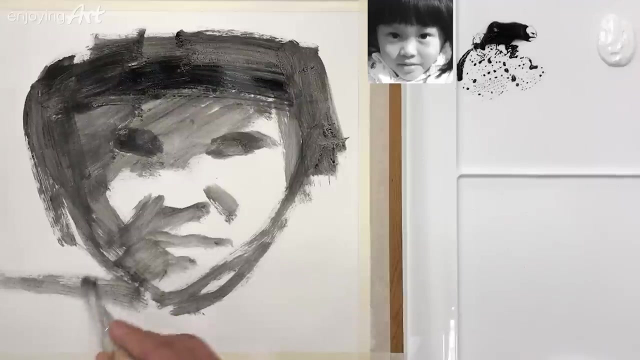 here, Look like a little triangle or the heart shape. You see that Over here, Like this, Like that And a little catch the shadow on this side, Like this, And also see that a lot of detail on the coat. But you have to see the shadow side and the light side. On this side it is. 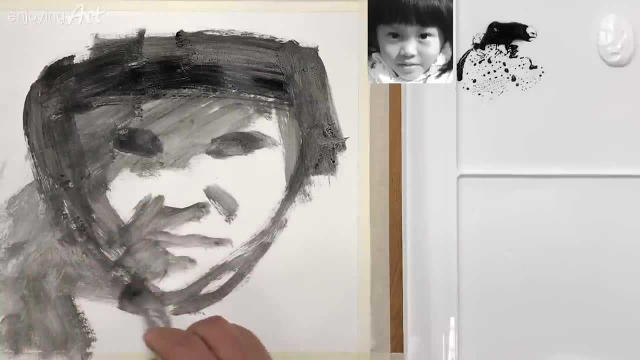 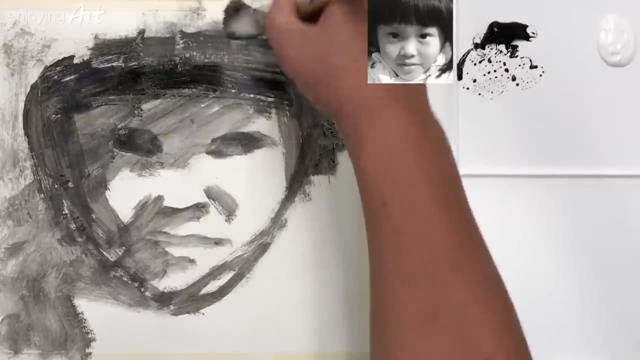 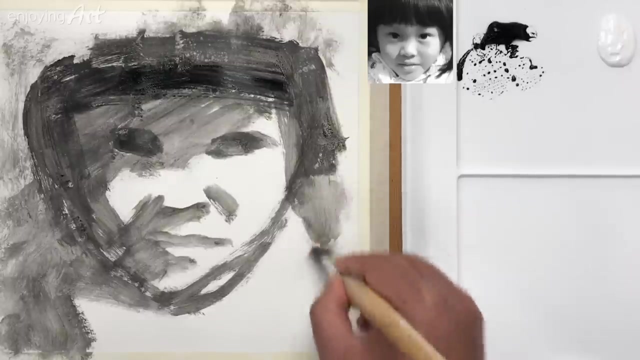 a little darker than this side And of course, a little catch the shadow over here And this is dark too, On the top over here And the hair over here is a little bit lighter. So when I say it's the hair over here, I just say that area is the hair. But, however, when you paint what you try to. 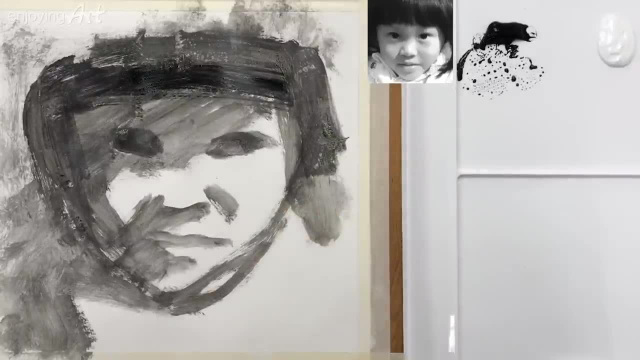 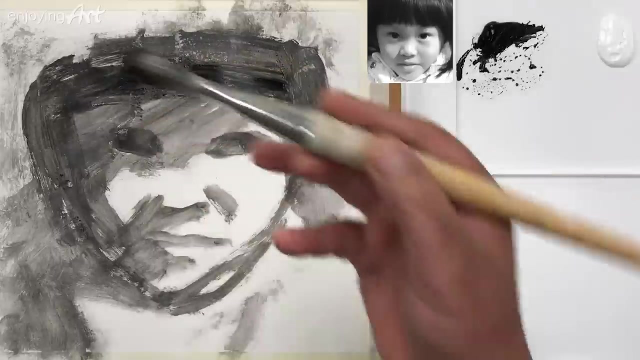 pick up is how dark is the area Or how light is the area, And that's all you need to think about Now. I just finished the drawing with my brush, Alright, And now what I want to do is put it easy. Now I'm going to making sure there's a few areas, if the color value is in the proper contrast. 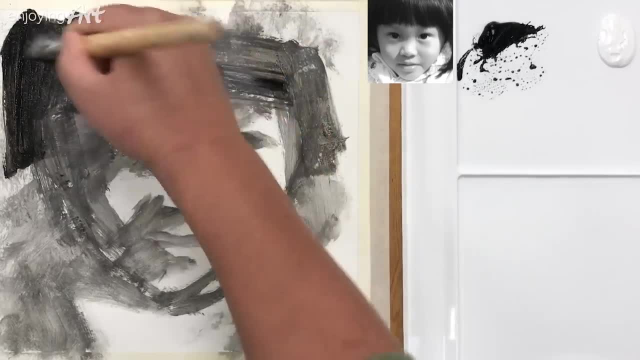 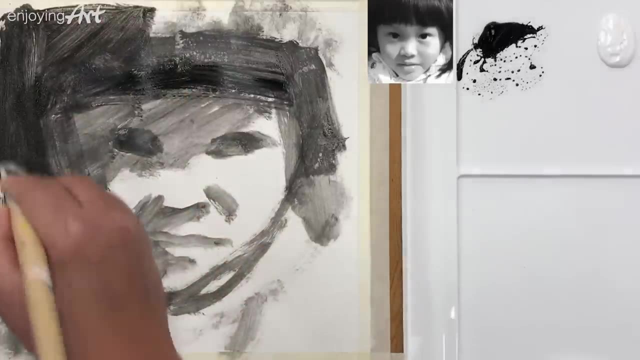 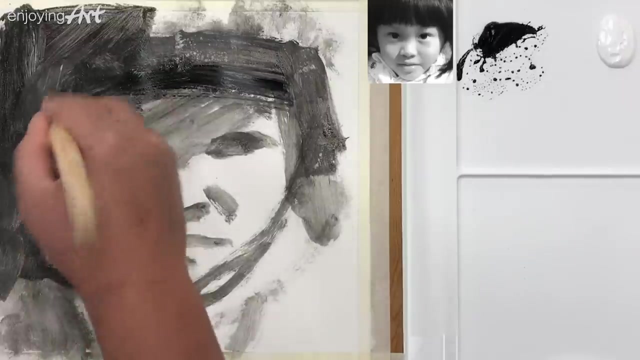 The first thing: Over here It's dark, So I make a dark color over here And all the way coming down here, The dark color And coming in a little bit. Look at that shape Like this: And that's the first. 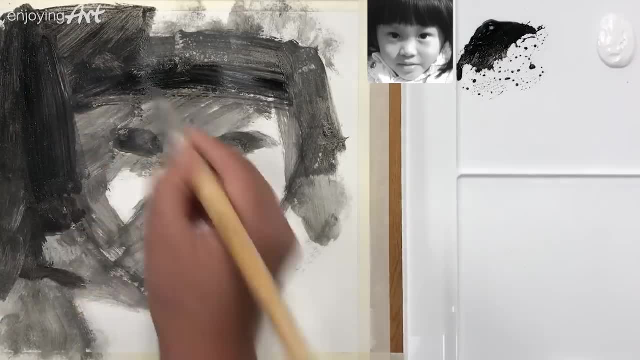 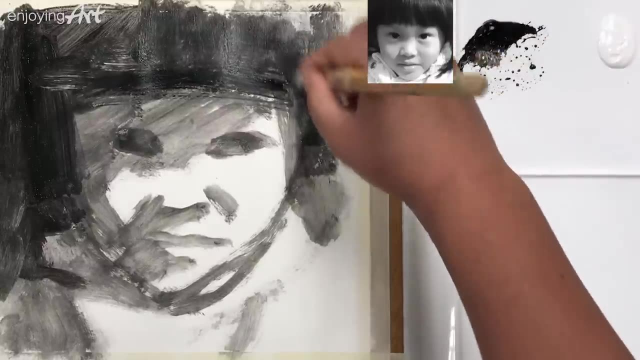 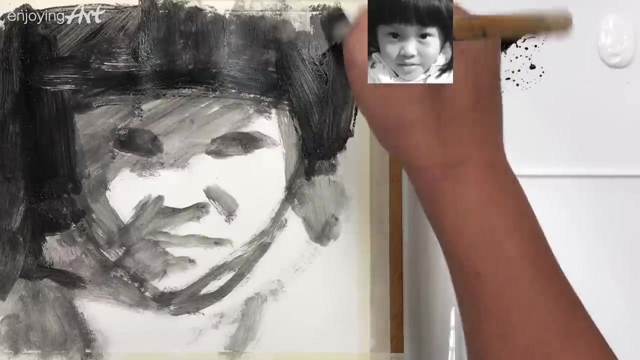 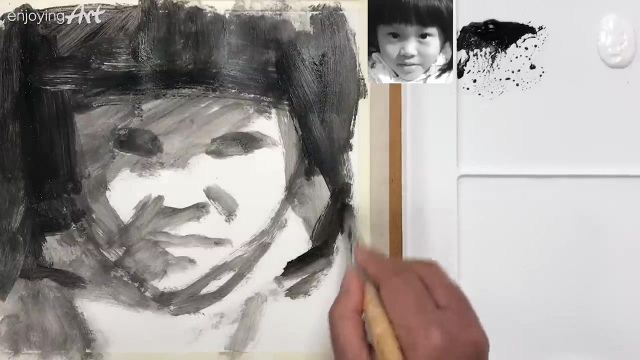 Is the really dark color And really dark color on this side. Really dark color. Use the big brush Before you use the smaller brush And the hair. coming over here And looking at the shape, How dark is that shape? This is the very dark area. 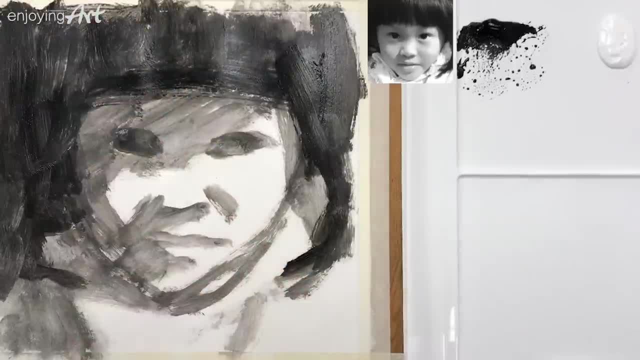 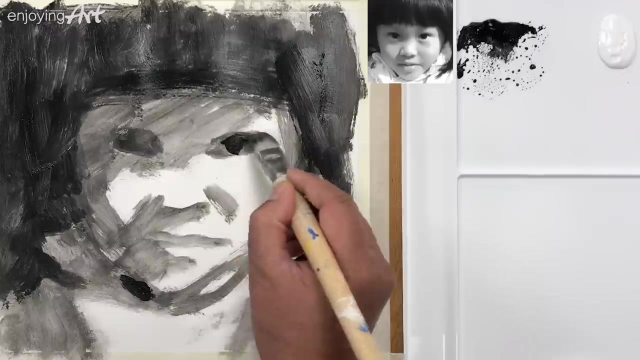 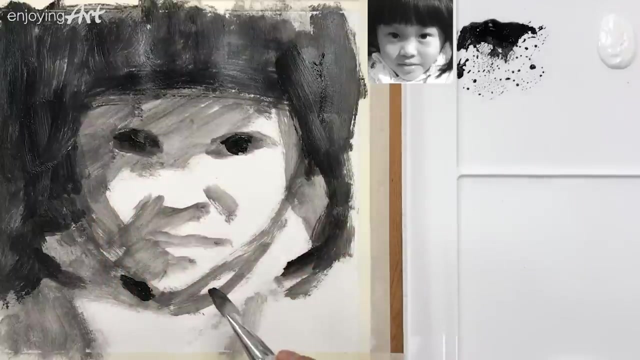 And we are practicing the thinking process And what you look for. And a little dark color over here, Like that. Maybe I throw a little dark color in the eye, The iris over here, Like that Dark color over here. And now I'm going to throw the other two colors. One is the light color. 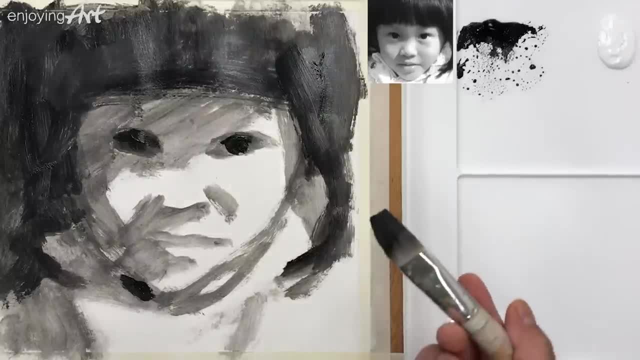 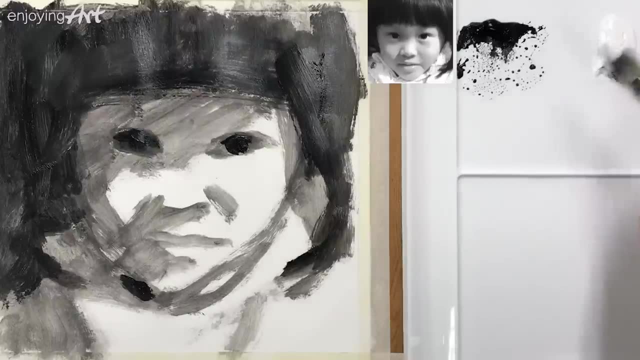 One is the middle tone. Now I'm going to maybe use the same brush. I'm going to let go some of the dark color first, Now mix a little white Here, And then I'm going to go into this color. Now, what is this color? This color looks like the middle tone. I'm 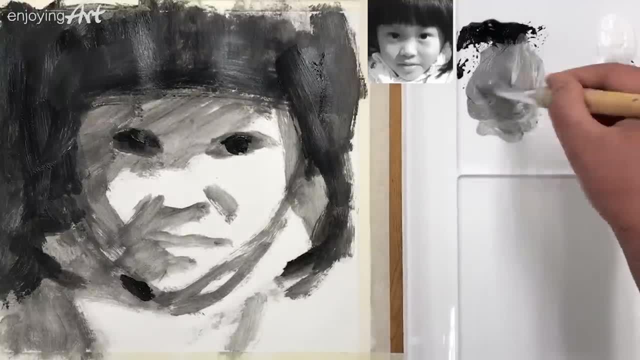 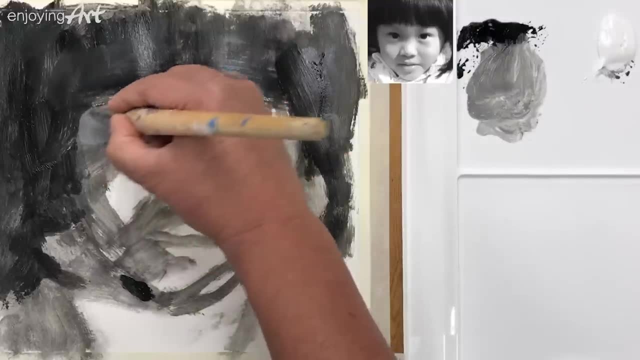 going to take this a little bit darker, Like this: Alright, That's good. Now what I want to look for? This color, Alright, This is the middle tone. You see that It's a little bit easier than doing the square. Seems like doing the square a little bit easier Because 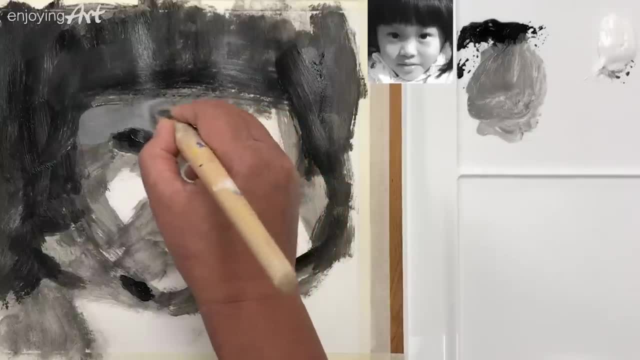 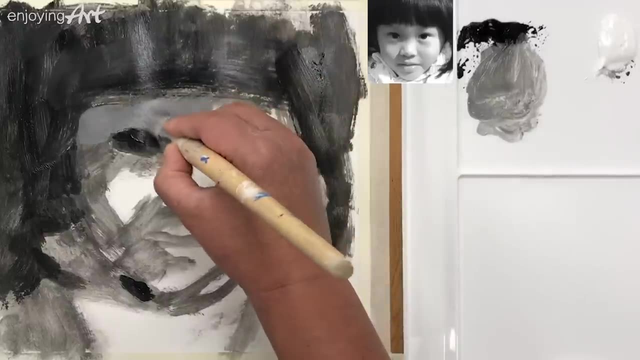 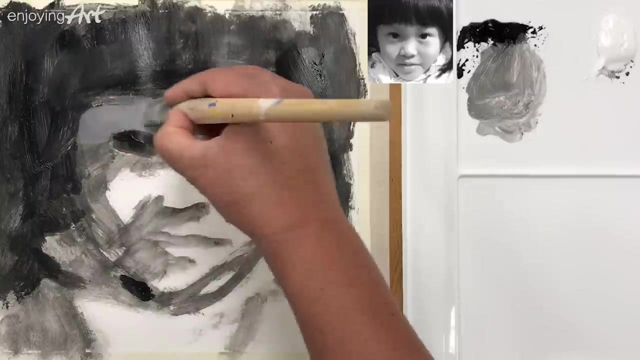 it's. There's just no fear Because it's just the square colors. But when you're thinking about a portrait, Just thinking about as is the square of colors, Is that easy? Like if you think about over here, This is Okay, This is one area of color And coming over, 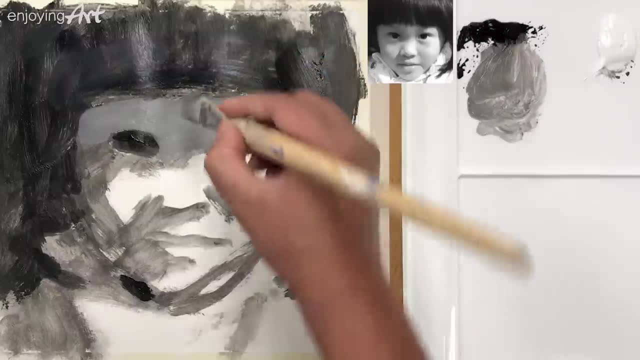 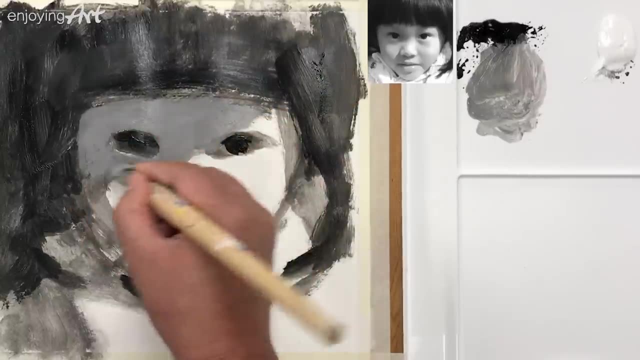 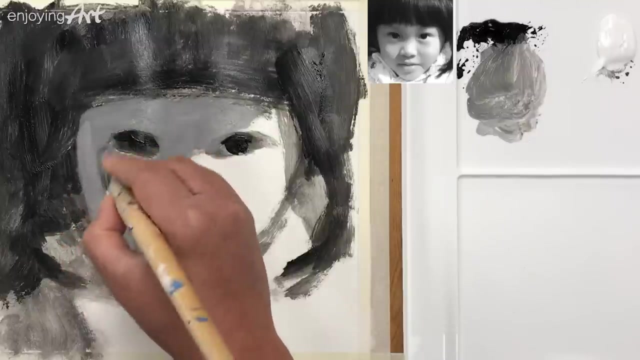 here. I'm going to make this similar color together, Coming over here. It's very similar Because it belongs to the same shadow side And we're going to coming down Like this And coming down like this, Looking for the shape, And if you're looking, Just thinking, 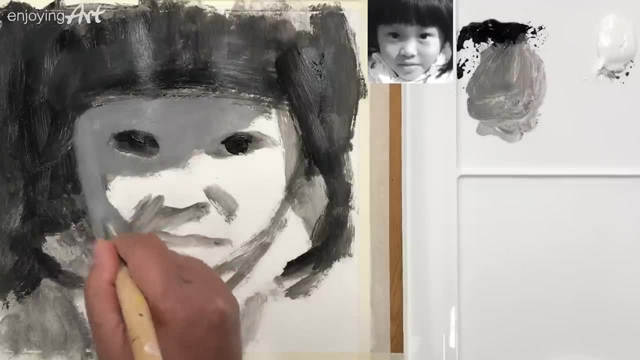 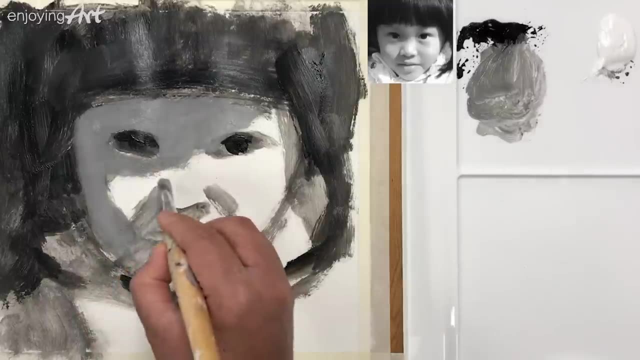 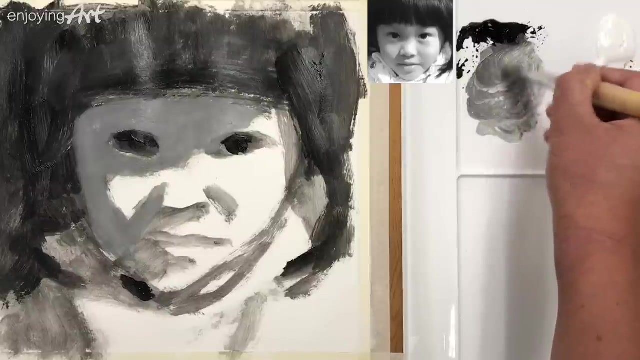 about the shapes. You won't feel a little fear Because you're. It's not actually hurting this beautiful baby, It's not. It's just What you try to do is to find a shape And actually over here Maybe a little bit darker Right, Just think about one of the square. 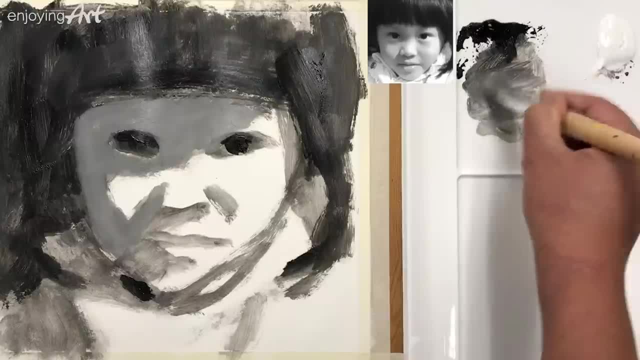 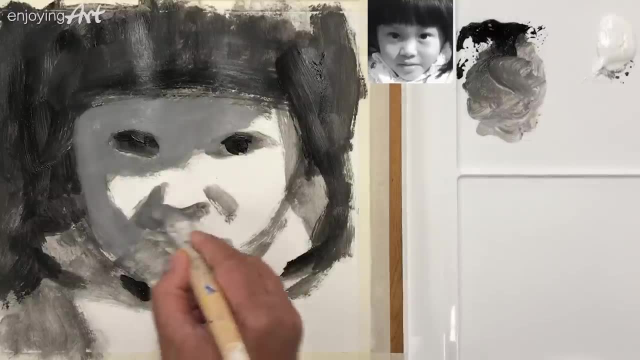 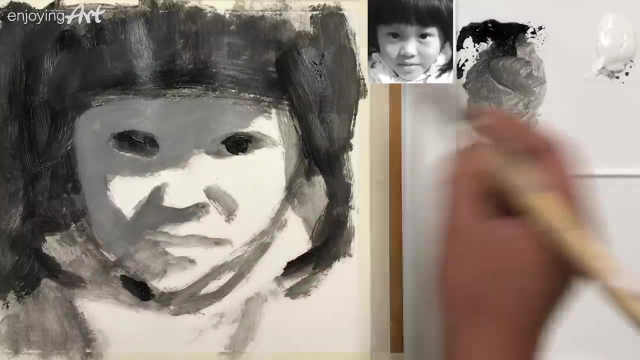 The value. And what value is it? And this about this color, A little bit darker Like this, Like right over here, Okay, And coming down Like this, And now a little bit lighter, Join that color And also the same value over here You think about. It's also up here. 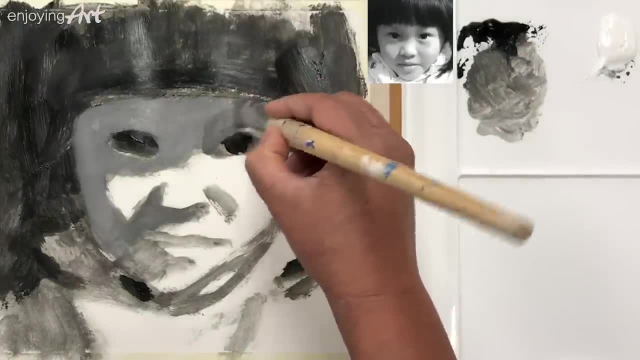 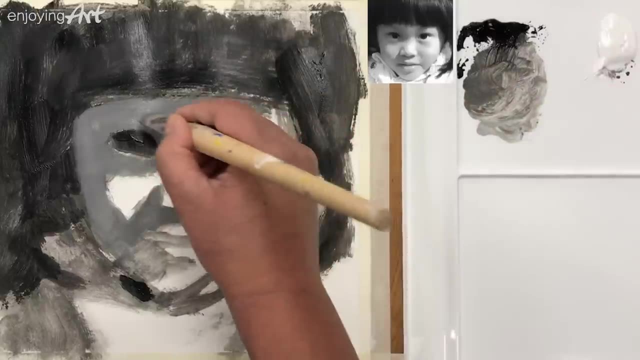 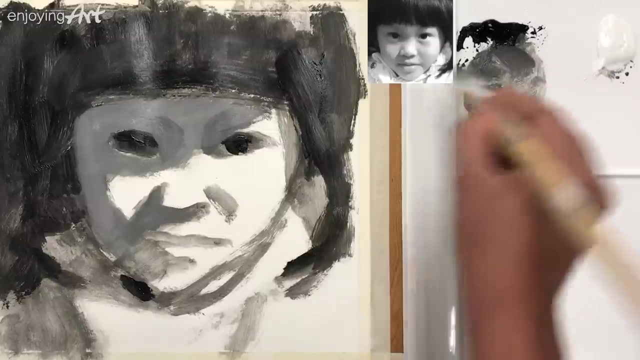 A little bit darker too Like that, And also the similar value That also over here Make a little bit darker too, Right In your mind. They are all Different shape of colors, A different value. Right now We don't even 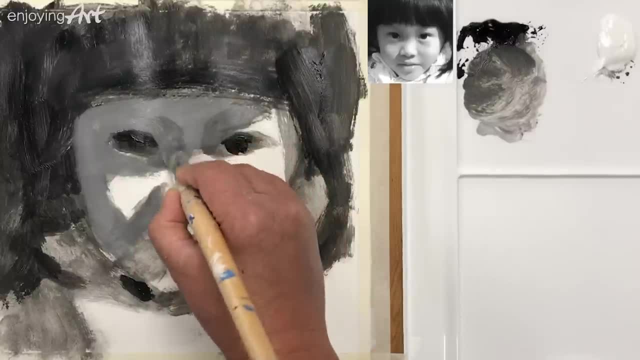 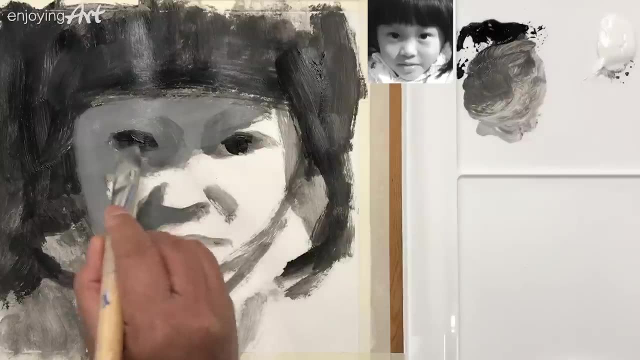 thinking about. What is there? How much is the red, How much the blue, How much the yellow? You just think about How dark is that color? Because we only use One color, Which is Black Plus the white, Actually two colors And the corner over here. Now I'm going to 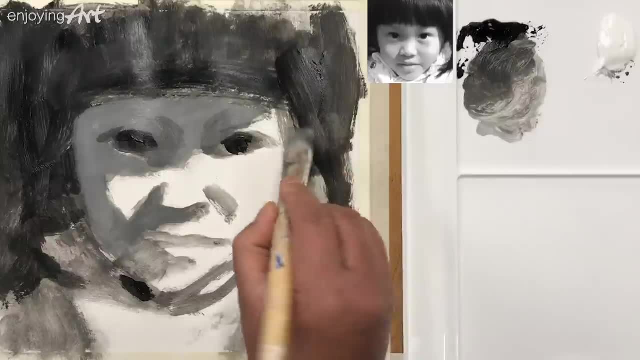 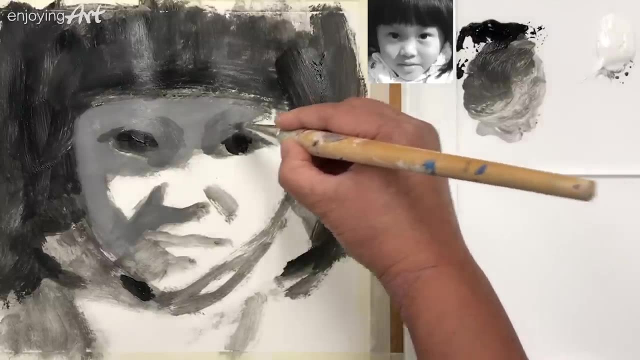 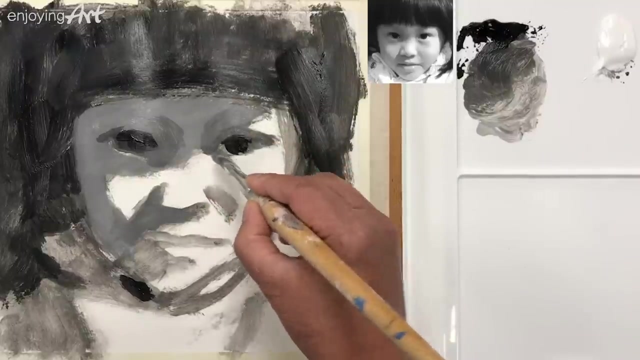 think of like smaller That, also a little bit darker That color, And here I'm going to just use A corner of this big brush And put over here. That's a little bit darker color Right over here, Like that, And a little bit tip color over here Also the similar. 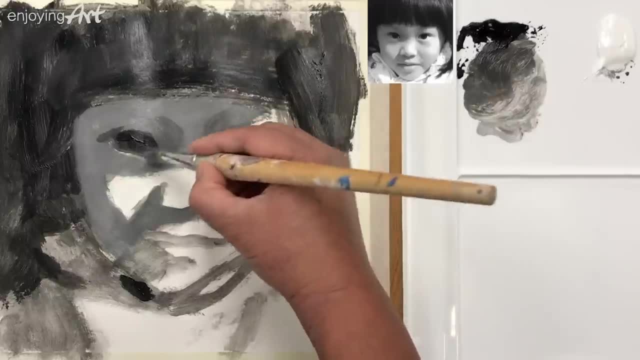 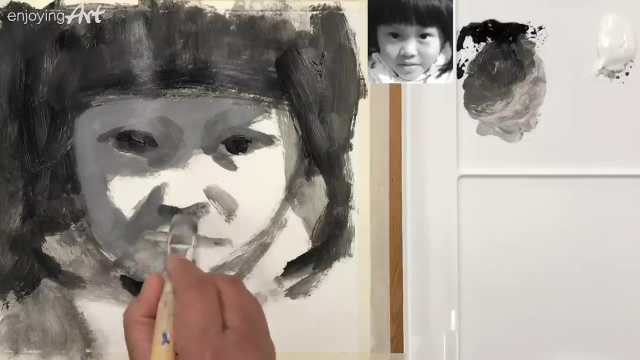 value as that. Yeah, Okay. Now take a look, And under the nose over here I see that actually A little bit darker in here. That's Just think about. that Is the color, And now I'm going to put a little dark color over here. Okay, 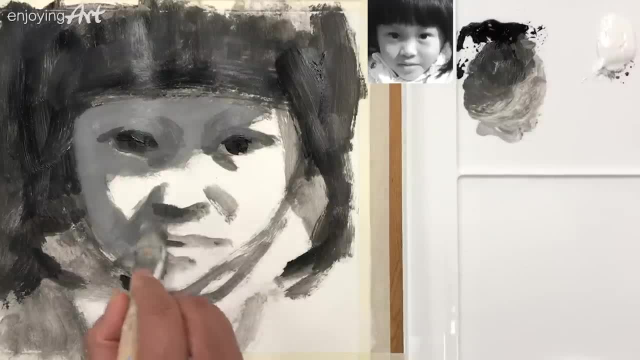 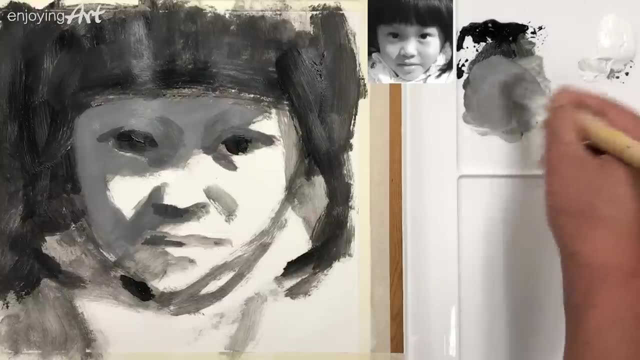 And actually This is similar color as this, So I'm going to mix a little bit lighter color. Just think about they are all colored chips And how you going to mix those color. So first, what I'm going to do, I'm going to put the color in here, Or maybe a little bit too light. 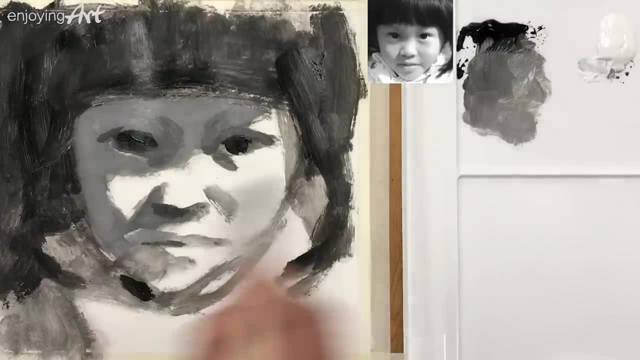 Now you can see After this exercise You just did In the last hour And you can Mix those colors Pretty easy, Like over here Coming through, This is good Now coming down over here. See the color over here, See the big color shape. This color adds a little bit lighter, Like that. And 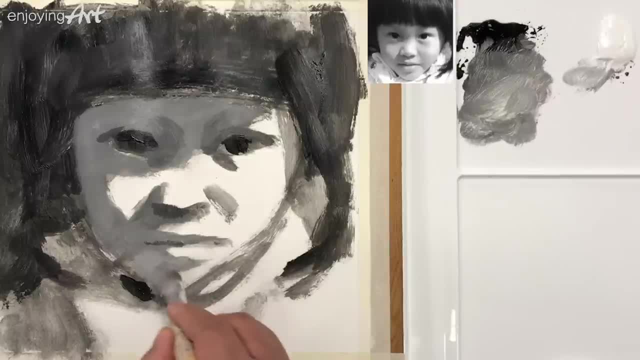 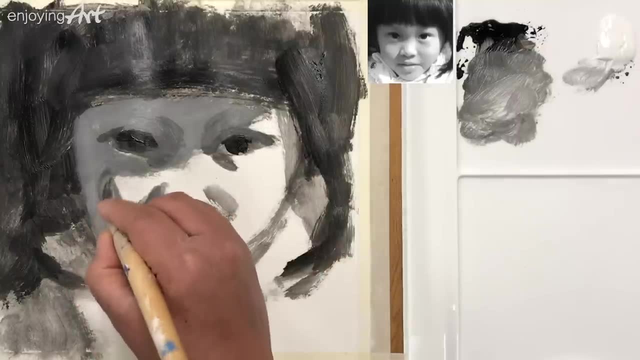 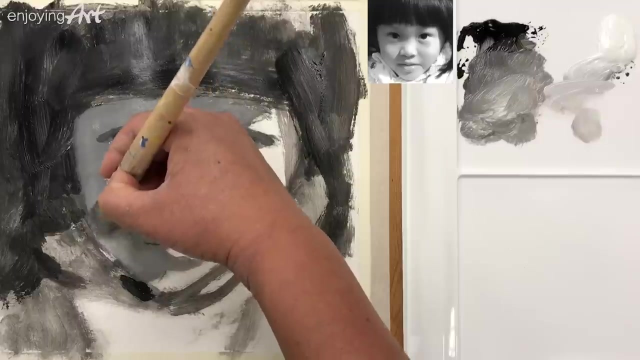 come through over here And There you go, Take a look at this color And coming through And have some reflected light, So And the edge over here adds a little bit lighter. Like that, Put a little bit lighter color chip And the edge over here And coming. 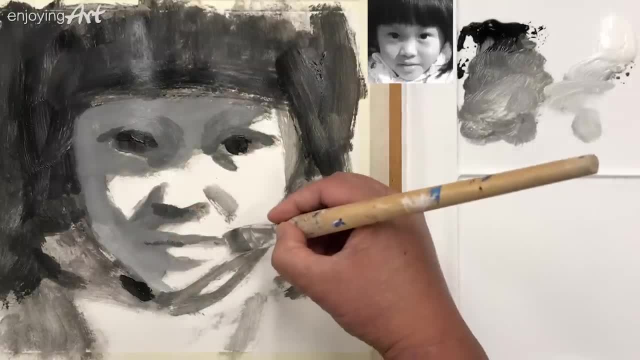 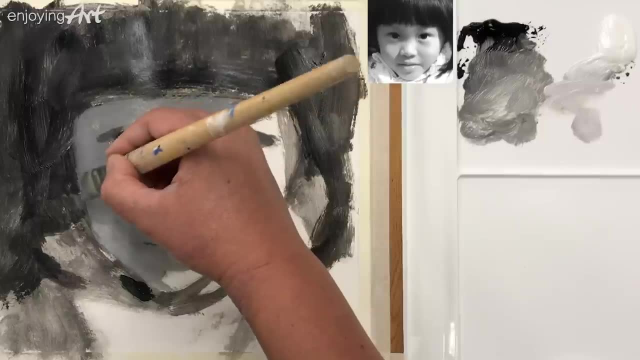 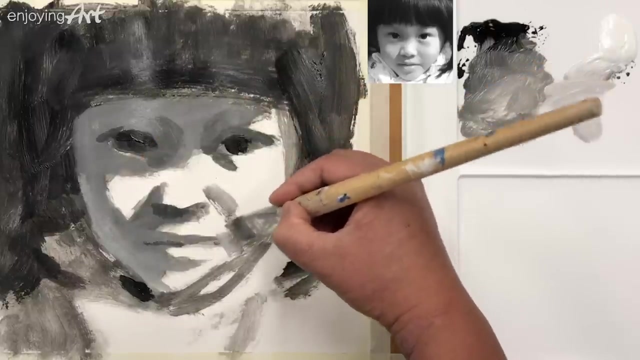 through over here Like that And the corner over here. You can see there is a shape. There is a little bit darker shape. Actually you analyze it. This value, Similar to this value, And actually it should be a little bit lighter The corner over here. So this is similar value. 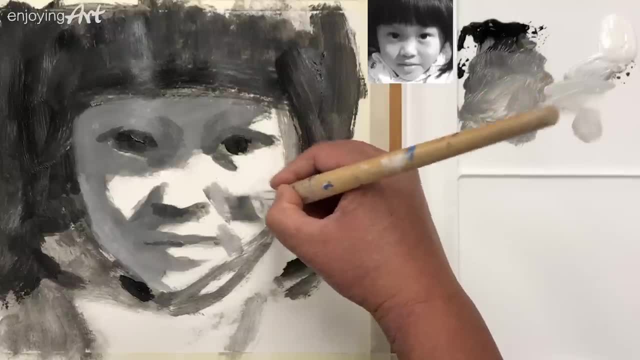 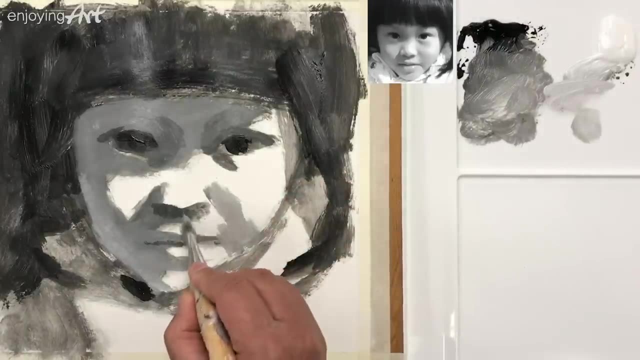 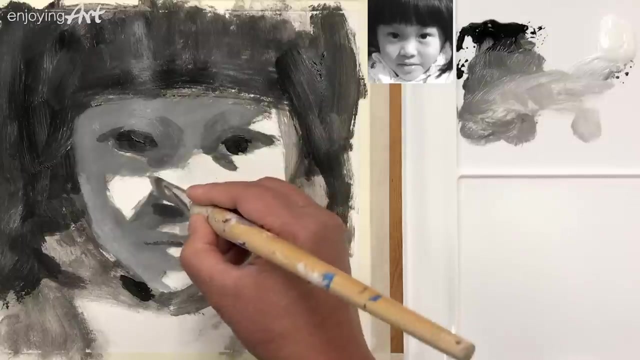 So this value also connect with this color And coming up Like this, And then you can see this Right And also Have a little color chip over here Also. this value. Now, looking at When you do this value Also, you analyze it On the nose Over here And also. 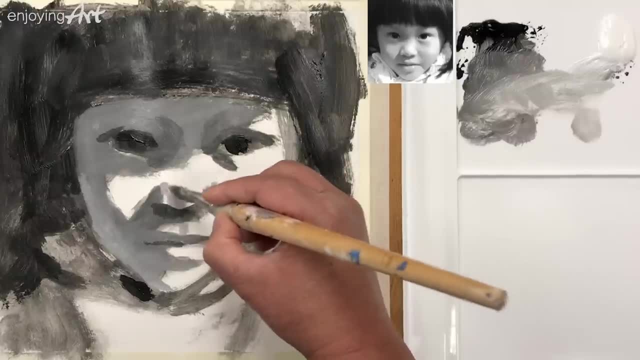 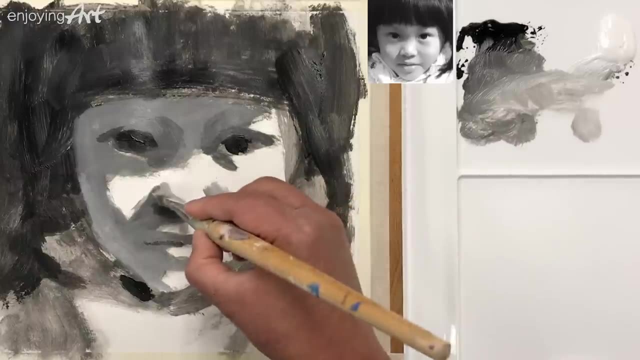 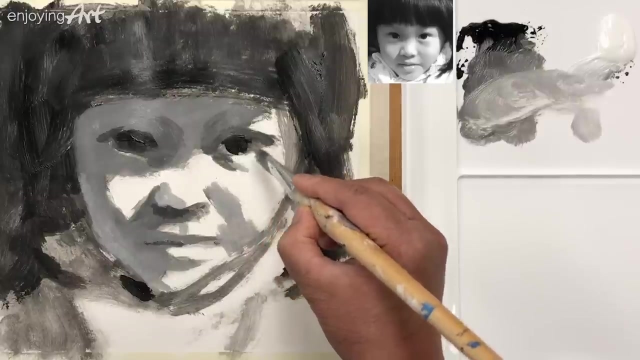 see a little value Over here Now The shape get a little bit smaller and smaller Over here. Also have a little bit Shape over here too, Like that. Now we haven't go into The lighter value yet We stay in the, The middle tone Like that. Put a little color Graduate. 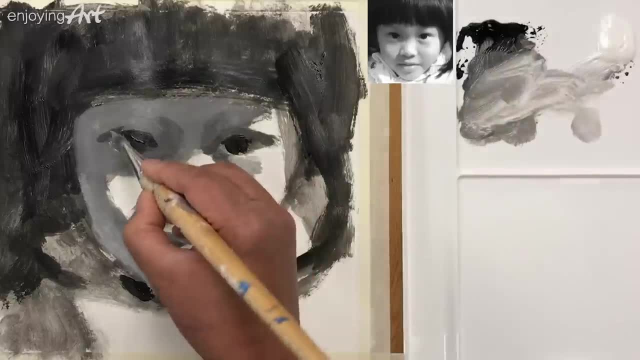 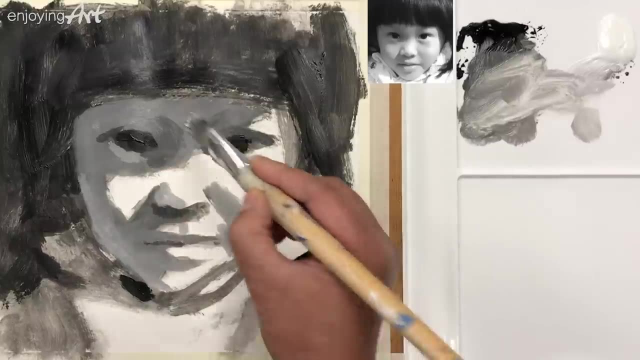 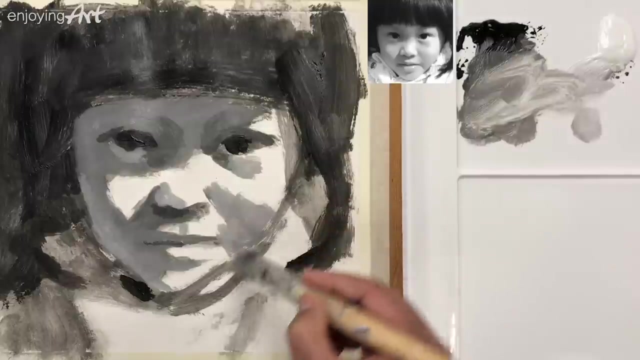 from there And this color actually also looking for same as the color over here, Like that. Okay, That's good. I'm gonna gradually make this color Get a little bit lighter and lighter coming Coming up Now. I'm gonna mix it a little bit lighter And then I'm gonna mix. 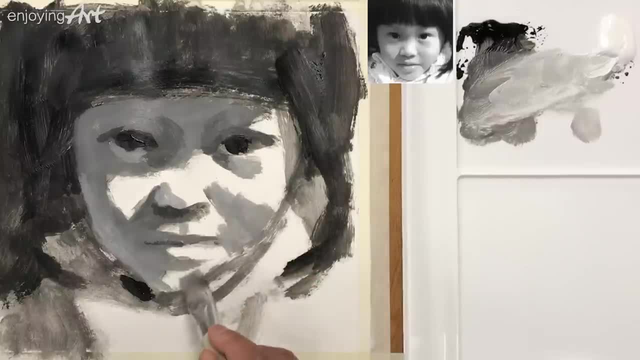 the color now Right, A little lighter value. You see, this value is like this Over here, Looking for this shape And looking for what color is it, How dark, How light is that color? I've been seeing this Every time And then coming up over here And the value over here. 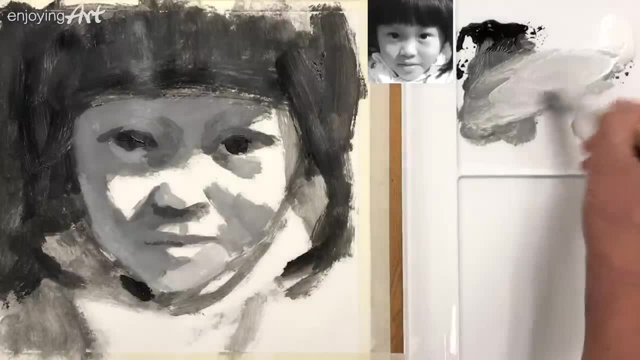 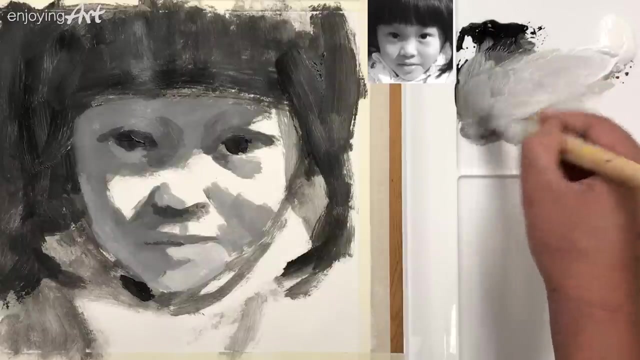 Just a little bit lighter, Like that. Now I'm come to The little lighter value over here. So Don't lost. Get lost In all the different shapes here And don't get distracted. Say, oh, Oh, my god, This is a baby. No, This is not a baby, This is only colors. Okay Now. 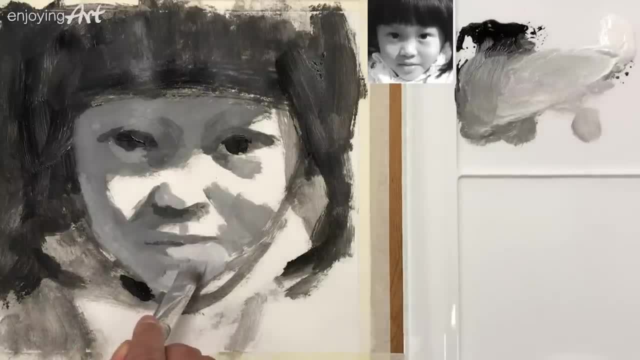 I'm gonna have this color And coming through like this, Like that A little bit lighter color Coming through over here. Let's just use the corner of this big brush Like this, Like that Now coming up over here. Now I'm gonna get a little bit lighter color And 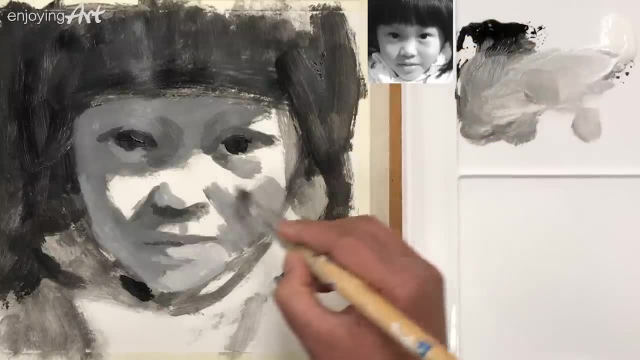 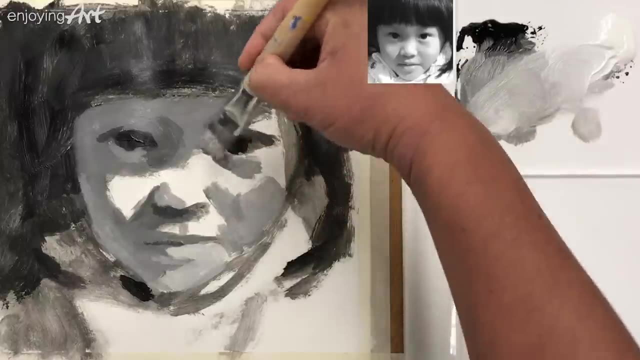 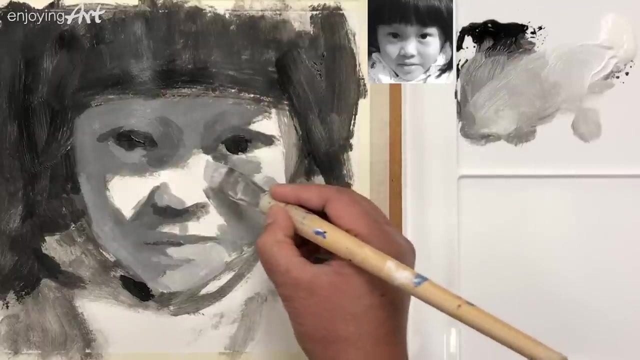 over here. Now I'm gonna get a little bit lighter. Okay, And now I'm gonna use a little lighter color Coming, Or maybe just Get a little bit graduate, Like this area, Not the lightest area, Like coming over here. Okay, Don't, Don't give up And don't get. 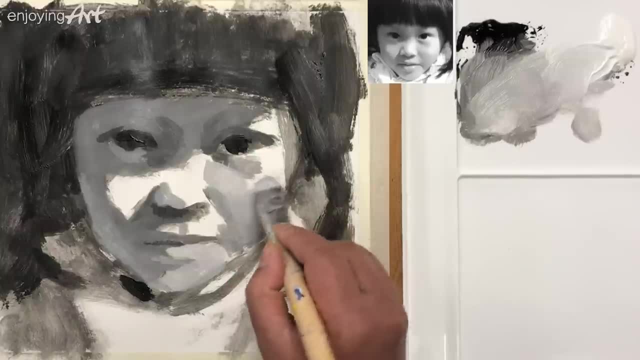 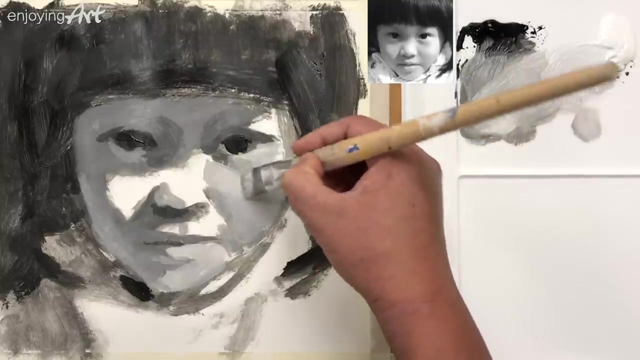 confused With a person. This is not a person. However, you wanna do it, How? Doesn't matter how, How hard you do it, It's never gonna be. You will make a baby On the paper. All you can do is to make the shape Of colors. Now, 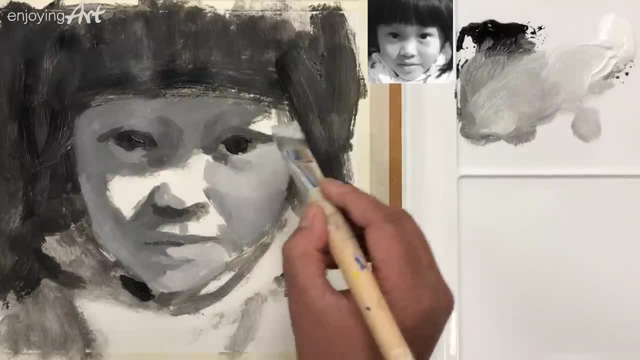 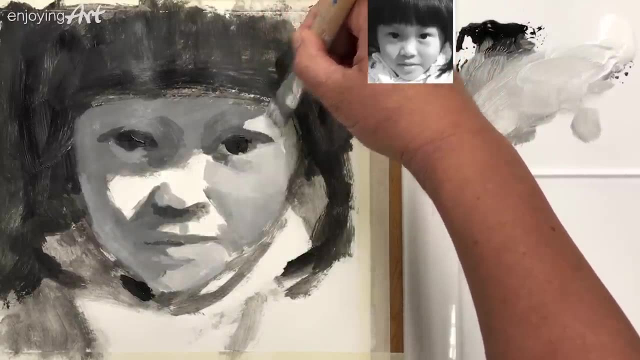 I'm gonna put this shape Looking for the angle of this shape. Now I'm gonna keep going Over here. There's a little triangle, Looks like a triangle, And the top over here Like this Top over here, Just looking for the shape, And that make you feel a little bit. 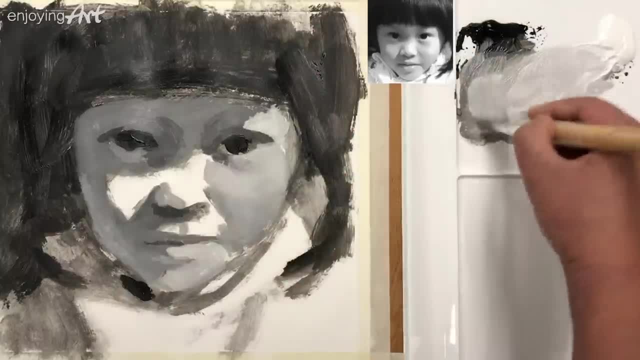 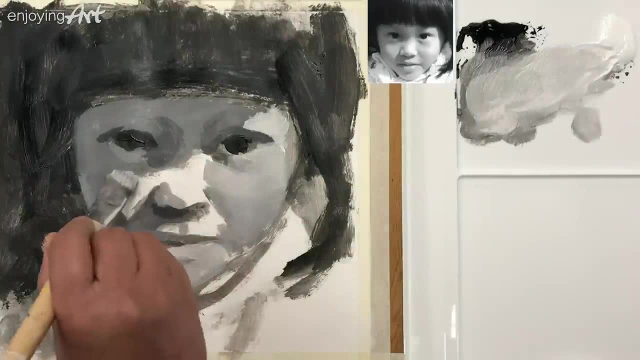 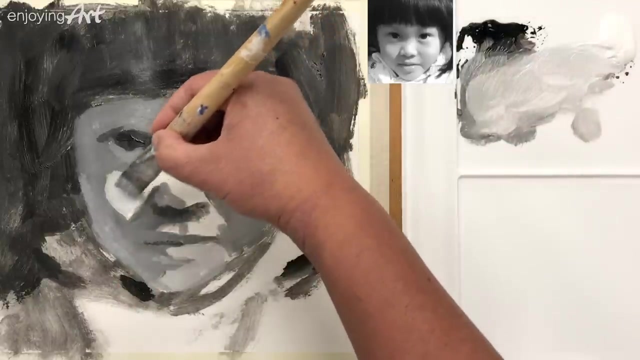 better, A little bit easier. Hopefully It does. And Coming over here, I'm gonna putting this color in here, So Don't think it's a person, Just The shape. The same thing that you did In the Uh Squares, This Coming up Here. 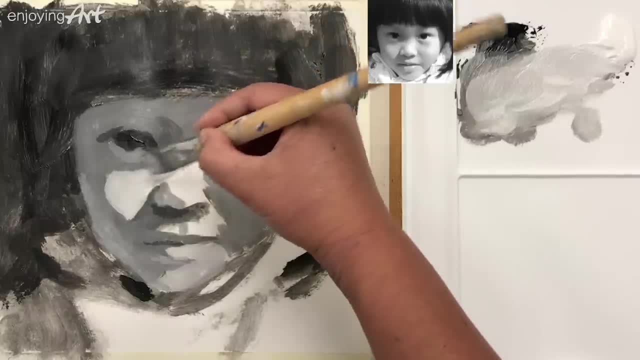 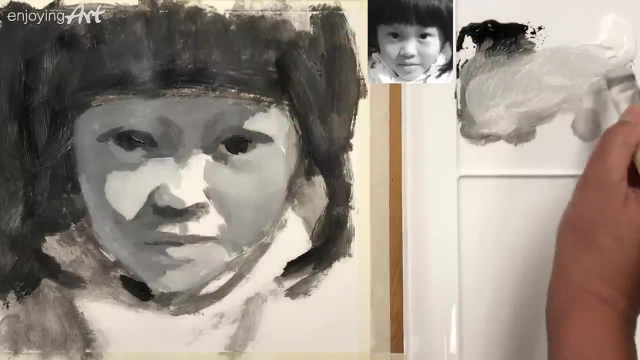 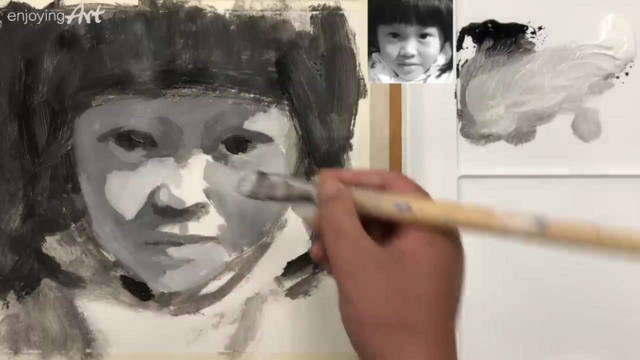 you go Coming through over here Looking for the shape And I think this color A little bit connected In here, Like this Coming up This, And I'm gonna throw a little color Into a little bit shape Over here, Like Right here, And make it look like the side. 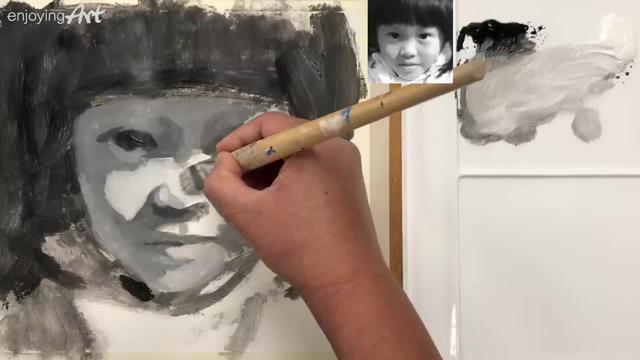 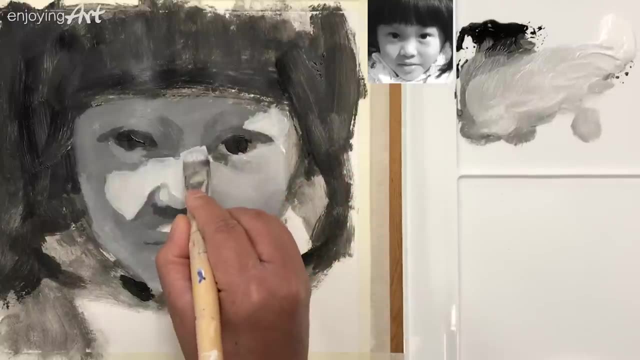 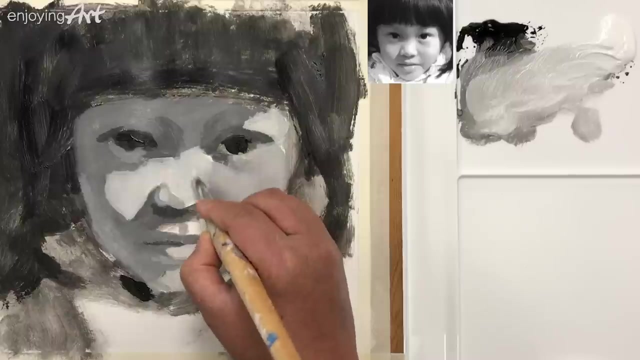 of the nose And Coming through On this side Looking for the shape. Okay, Here you go, Coming up here And throw a little color in here, Like that, And this color Gradually turn into this color. Okay, We're gonna use A smaller brush To fine tune The smaller. 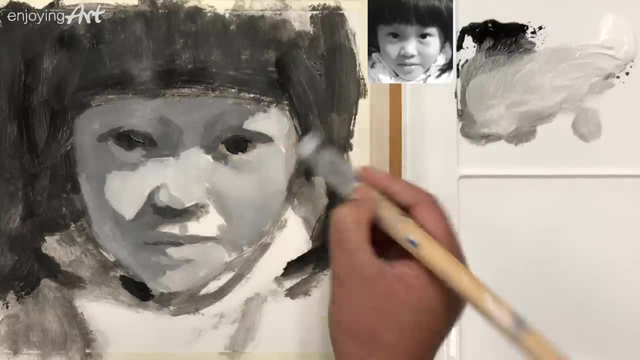 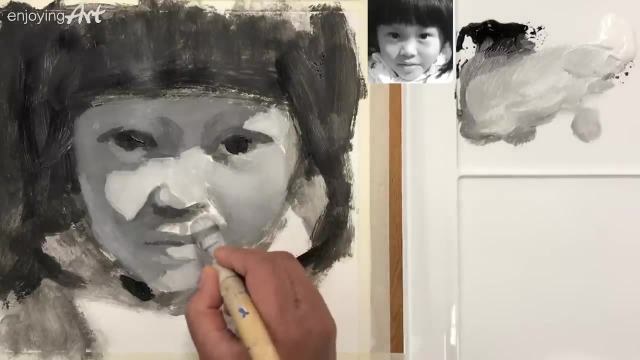 shape Like this, Like that. And now I'm gonna Add a little Light color In here too. Just pretend this is your first round Of your exercise. Uh, With the Uh 16 or 25 square, Add a little color in here. You can make a little raw. That's fine, Like that. 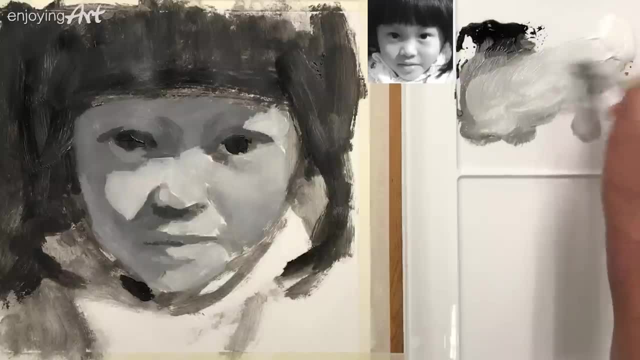 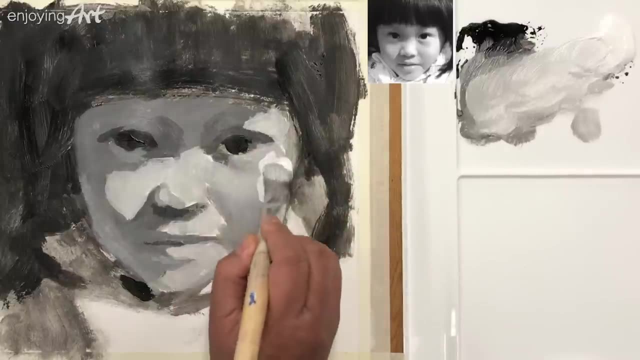 Now I'm gonna throw the lighter color. So Are you gonna do that? I'm gonna throw the color- Lighter color- Right over here And Have that shape. I'm gonna make the Brush a little bit thinner And I have the little. 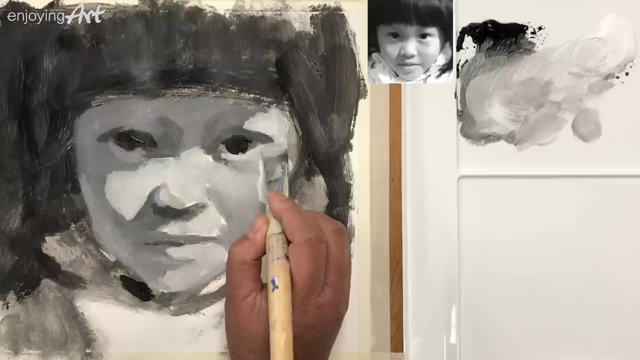 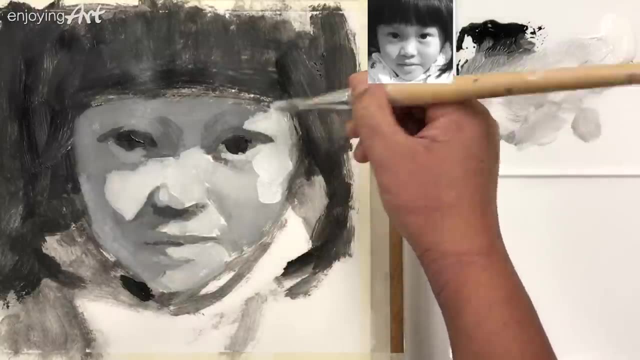 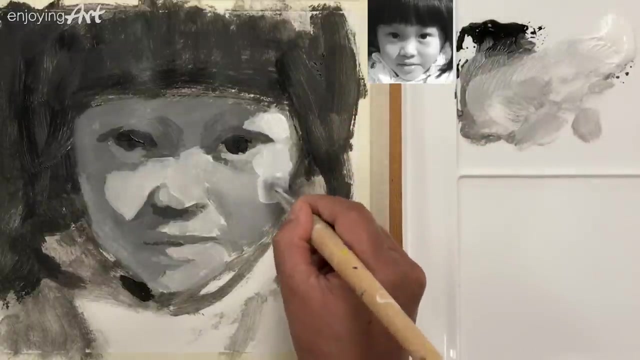 bit lighter shape Coming over here And coming through here. There you go, Make a little lighter value Coming like this, Coming up, And the top over here A little bit lighter. So I'm gonna Make a little lighter, Like that Coming up, Coming down over here A. 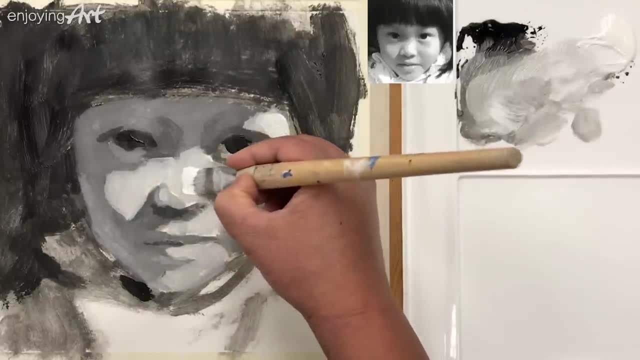 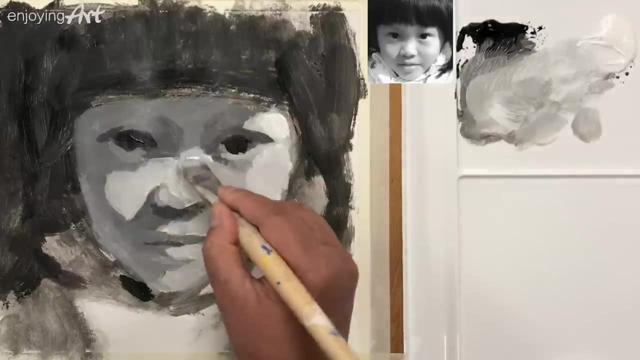 little bit lighter. Now I'm gonna throw a little lighter color On this side. See that Inside this shape Also, I have area On the side over here Because facing to the light side And a little bit lighter Like this And also a little bit lighter Over here. 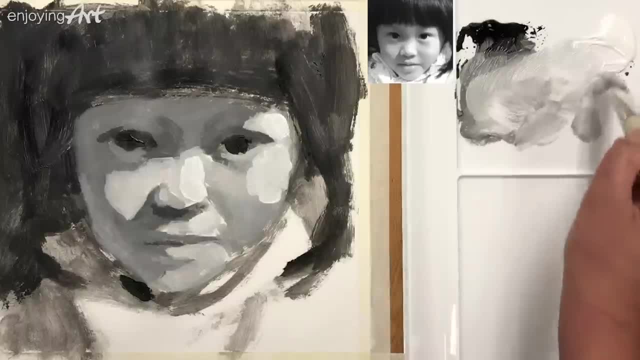 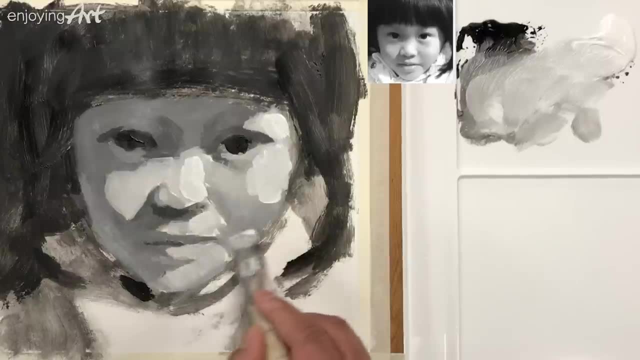 Now I'm gonna, Yeah, Divide it into a smaller, A smaller area And a little bit Lighter Over here. Now you can see, After you dry It should be a little bit lighter. Now I'm gonna use a smaller brush And I'm gonna put a little Really light color. See that. 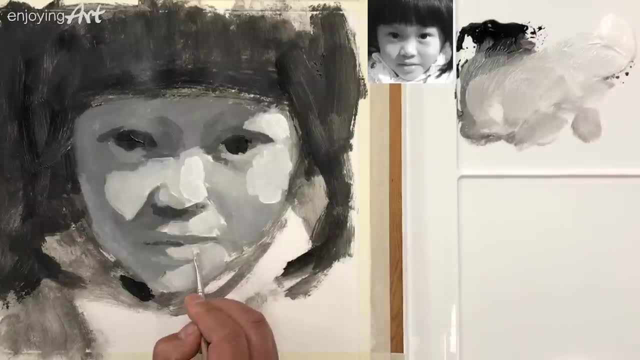 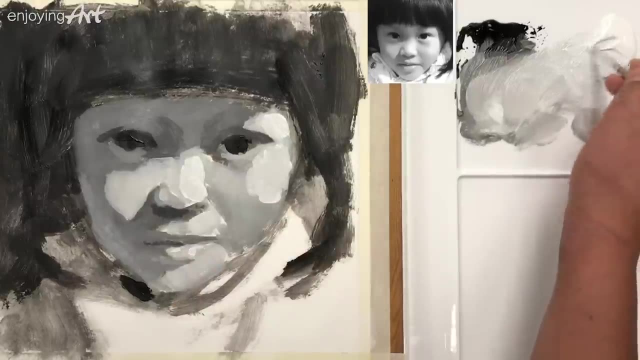 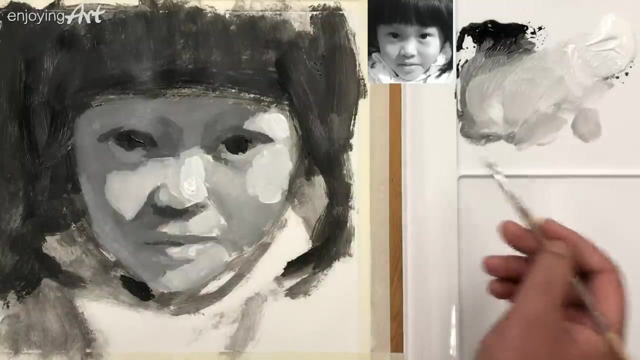 Little light color Right over here, Like that, A little bit light color Over here, And think about The nose over here. I'm just gonna throw a little white color For the highlight Right over here, Like this. Now I'm gonna Thinking about: Oh, there's a little. 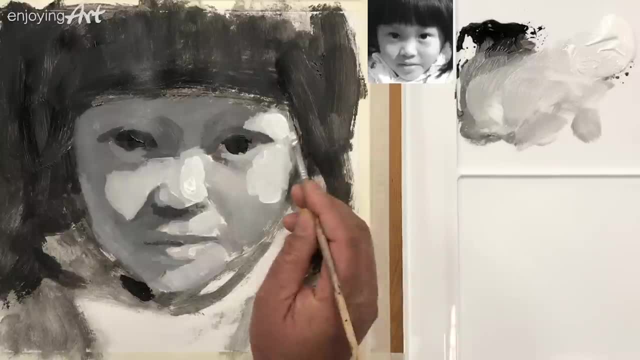 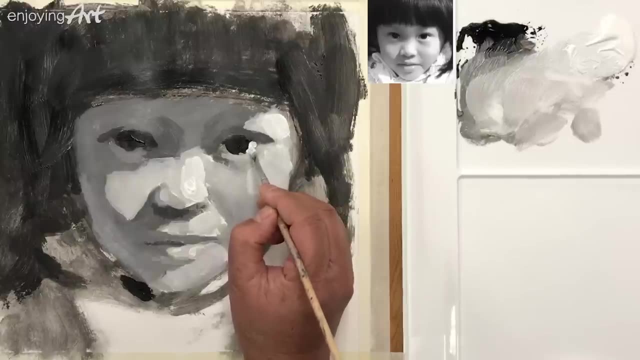 light shape Inside here. Don't even think this is an eye, It's just thinking about. There's a little light color Over here And Over here Like a little triangle. Just think about the shape And think about How dark. 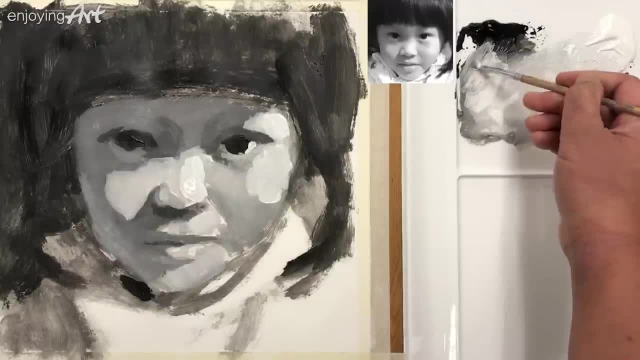 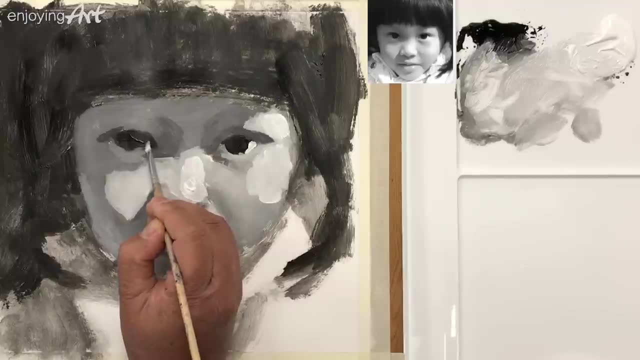 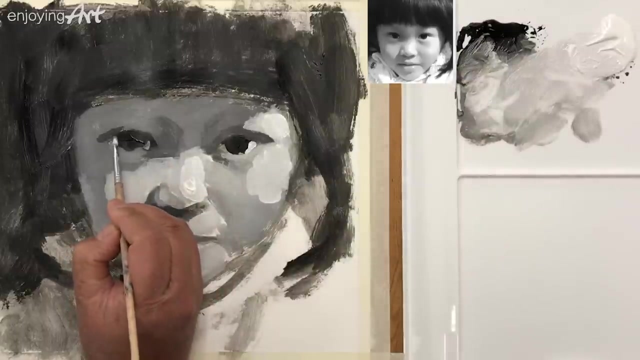 is the shape, And this side Have a little bit darker. So I'm gonna Make a little Darker color For this corner. Just throw a little Corner over here On the other side A little bit darker. Now I'm gonna throw a little shape over here. Got a little bit smaller. 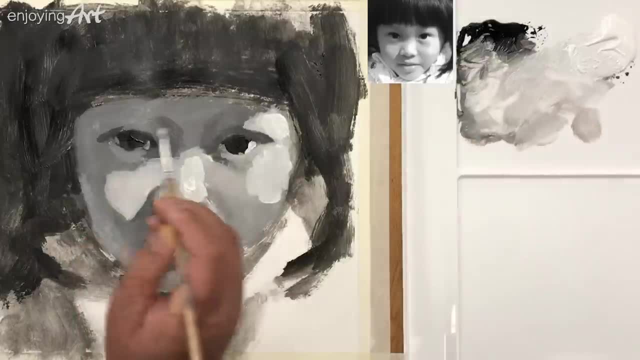 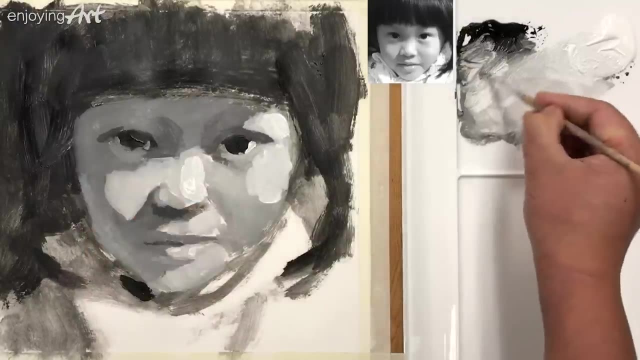 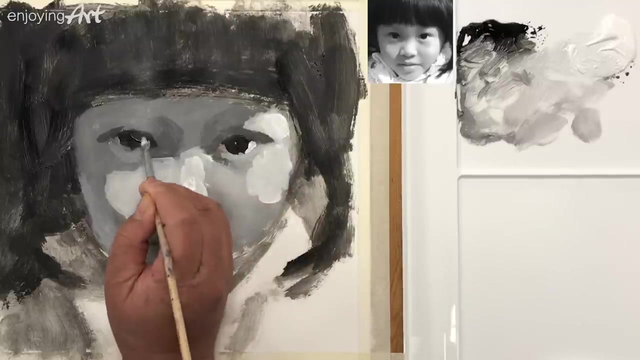 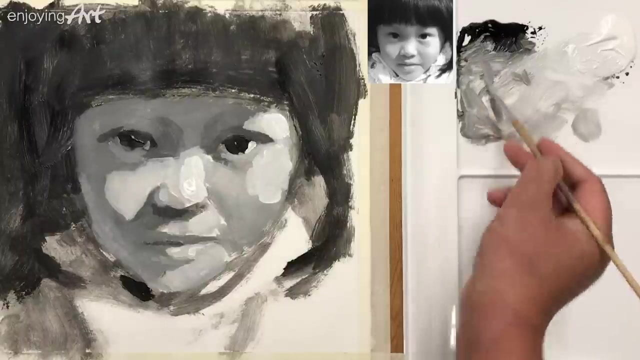 After you Control The bigger shape Right Now Over here, I'm gonna just draw a little color in here, Like that, And then Also Throw a little, A little bit Dirt over here, A little bit dirt Over here, And then Think about: Okay, On the other side It looks like. 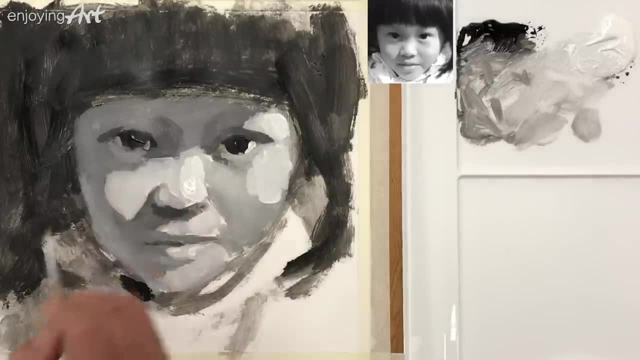 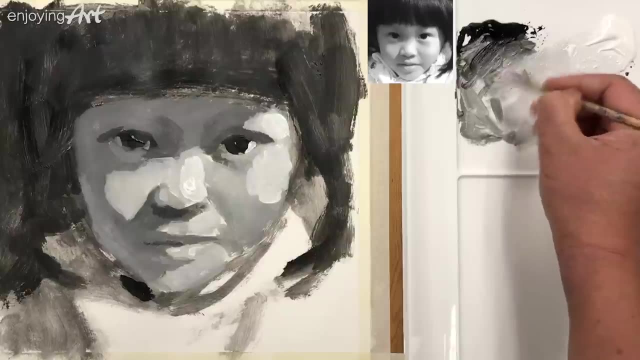 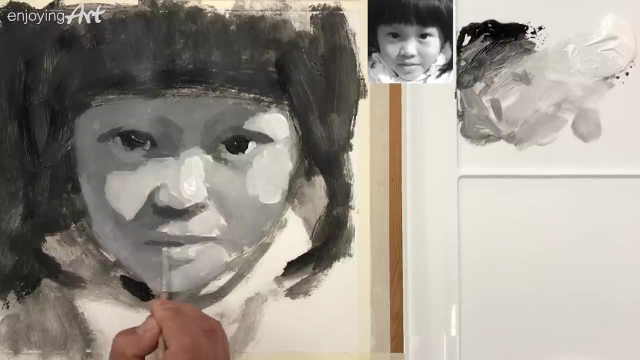 This shape can be a little bit more Coming through over here. And now Take a look And looks like In this area. You don't have to say this is a mouth Or nose. Just a little area over here Looks like It's a slight Little Line, A little bit darker, A little bit darker. 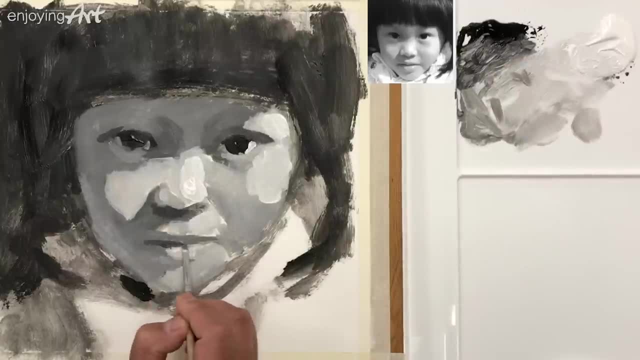 Even darker than this, So you can analyze Different values In the exercise. You can Do the same thing: Analyze The values Looking at Look like a person. Now I'm gonna blend this color together, I'm gonna have this And. 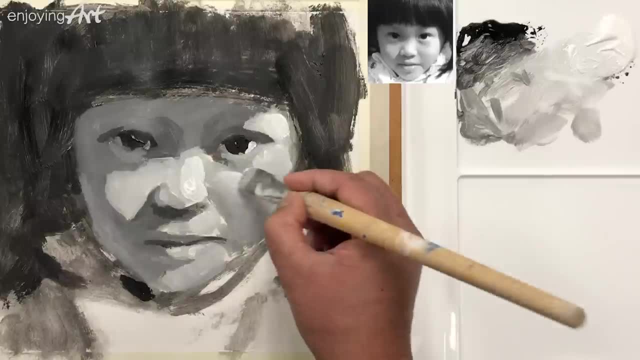 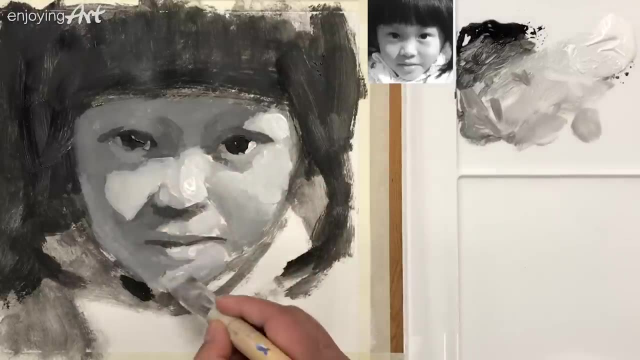 Blend it together a little bit, A little transition, A little bit softer, Like this, And you're gonna see Very easy Okay Coming through like that, And most of the time We just get confused And you, You have, You're afraid of trying. 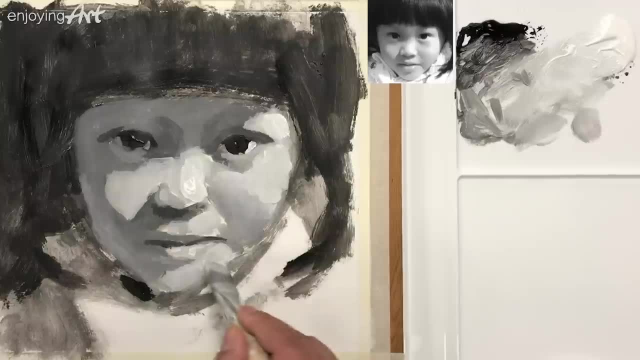 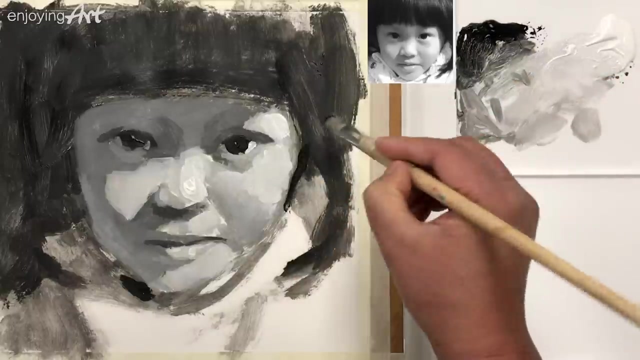 it, But It's supposed to be easy. If you Just thinking about, They are Just different shapes. Now I'm gonna come in over here. Come a little darker color. Now I'm gonna fine tune it. There's a little Line over here, Darker. Okay, I'm gonna get a little. 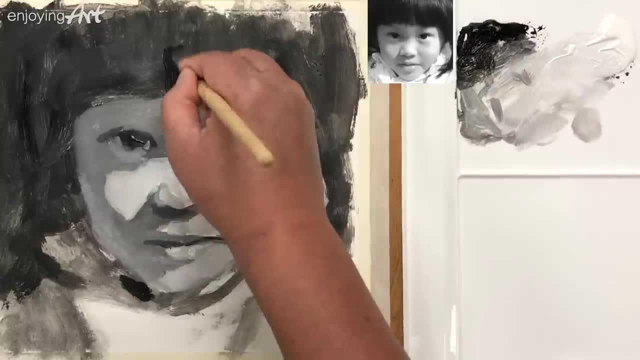 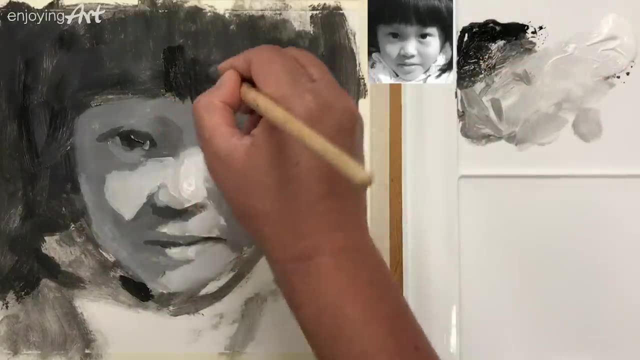 color over here And Here you go. I'm gonna Give a little bit like this: Watch, You can do this. I'm sure you can do it Right, It's pretty easy Like this: Just throw the The. 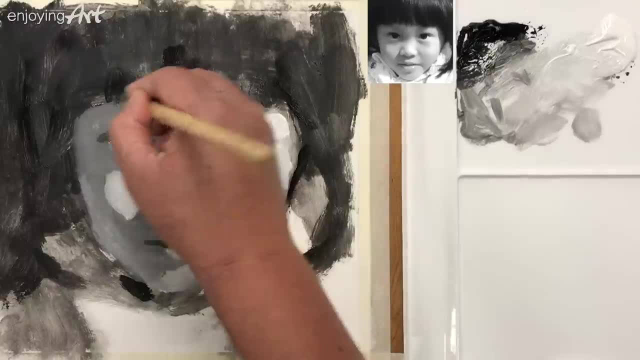 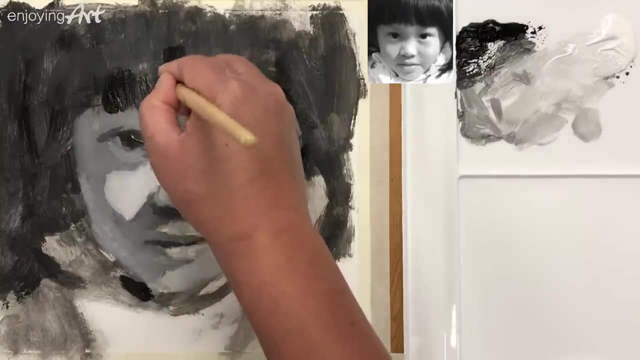 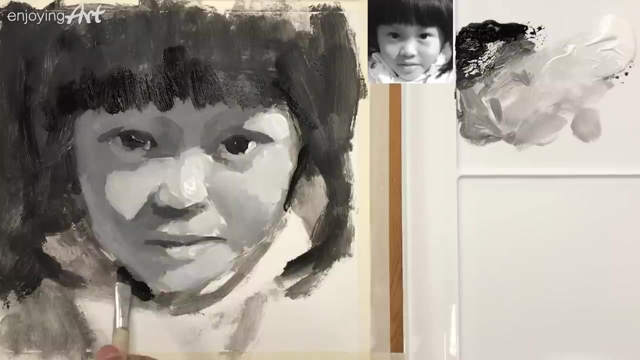 brush, Because that's just the edge. It's supposed to be The edge of the The hair. So you Have a little Like an old brush. It will work better, Like this, Like this. That is suggestions Now coming over here. Now I'm gonna throw. 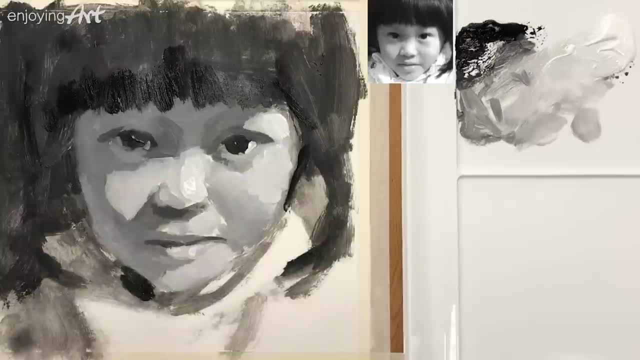 this line a little bit In, a little bit Like right over here. Now I'm gonna come in too To give a little Lighter value On the outside Over here too, Because it's not so dark. I want to make it look a little bit darker, Okay, And 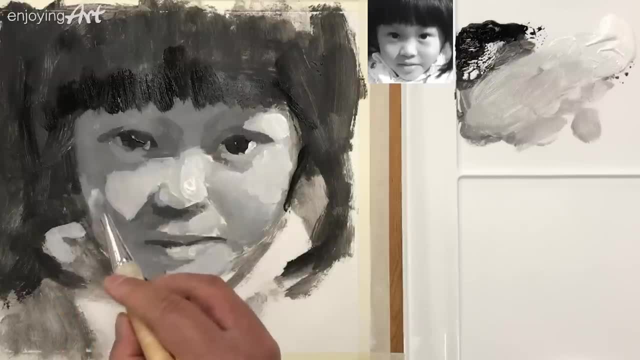 I want to make it look a little bit nice And, Just like this, Throw a little color, A little color in here Coming through, Like that Good, And then on this side I'm gonna have A little thicker color, So It will look a little bit better In the shadow side. 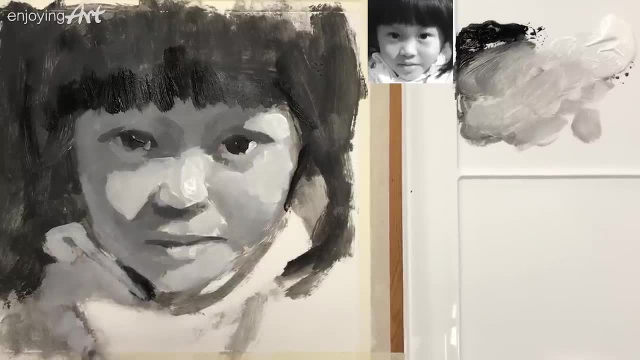 At the same time You clean up the color. Okay, Like this. Yeah, Here you go, Like that, And a little color in here, It will be nice, And on this side I'm gonna give a little color, And on this, The other side, Oh, I can throw a little color, Not the darkest. 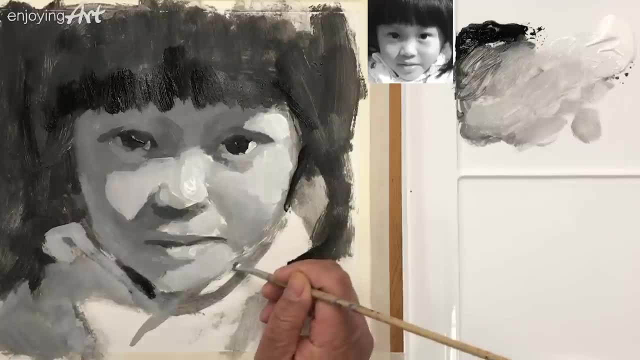 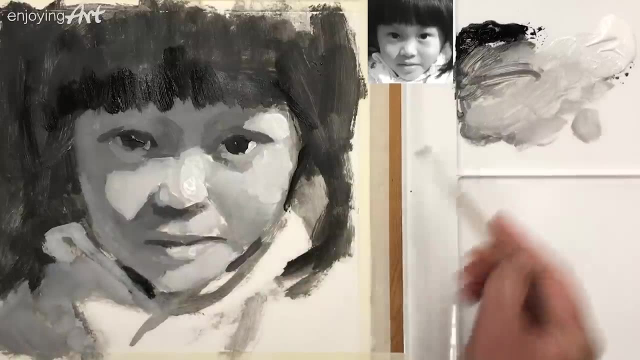 color, Just something like over here On the edge over here You can throw the color over there. Now you can pay attention To the smaller, A smaller shape And now Throw the color in here Like that. Now I'm gonna start Putting a little Really light color On the clothing. 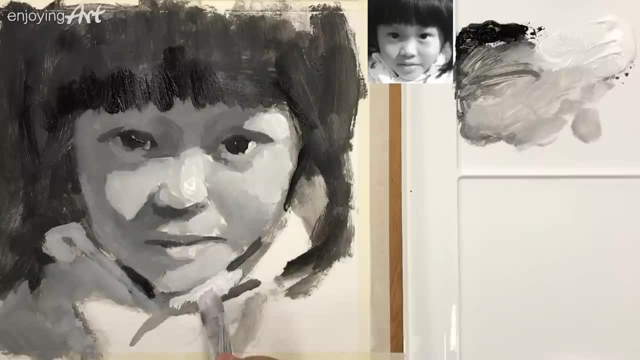 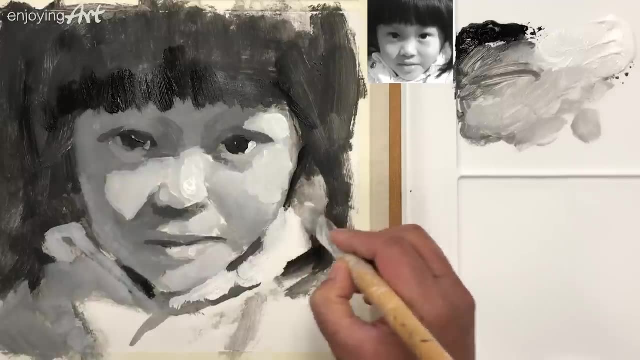 At the same time, Create a little bit more contrast Between the inside and the outside Of the face And you can think it's a face. But When you try to paint the face, You try to find out How dark is that color? Okay, And that's all you need to think about. You don't have 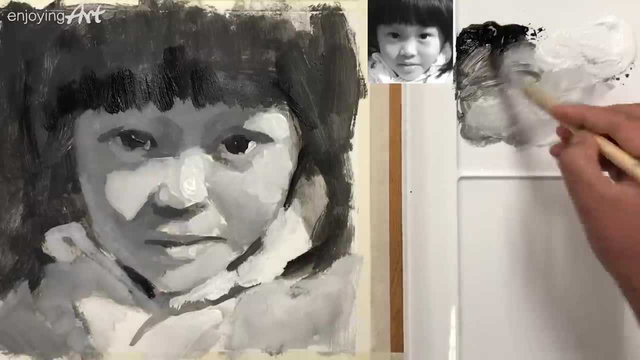 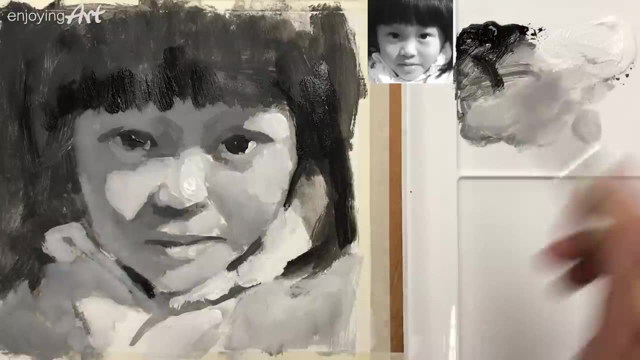 to say How I'm gonna make a face. I'm gonna come in over here To do A little bit, Make a little Lighter shape On the top over here. Now let's see What, How, What color is it? 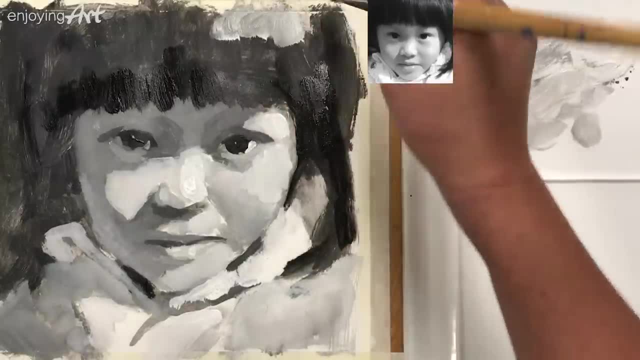 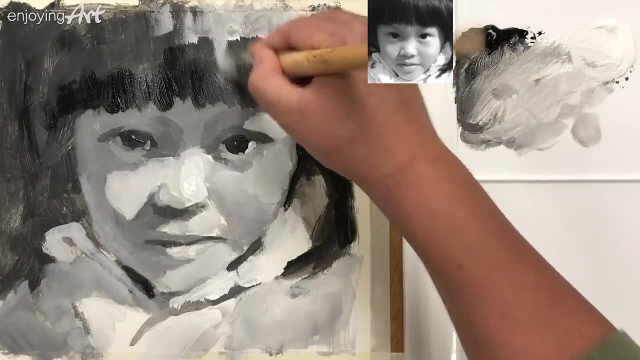 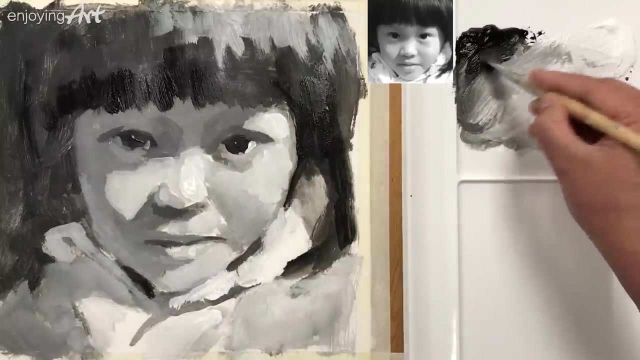 Over here Just A little Lighter. I think that's the middle tone. Like this, Okay, Like this. And if you Oh The color Too light, Coming down too much, You can use the Dark color And push it Coming back. 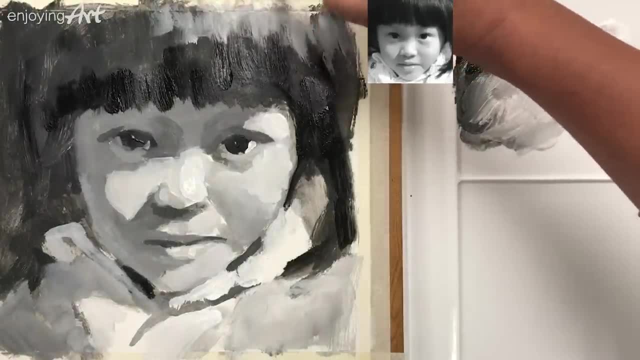 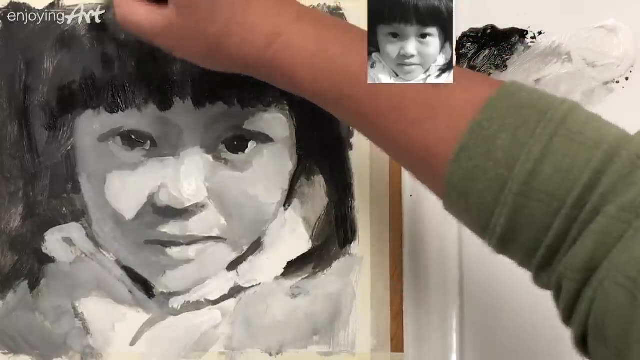 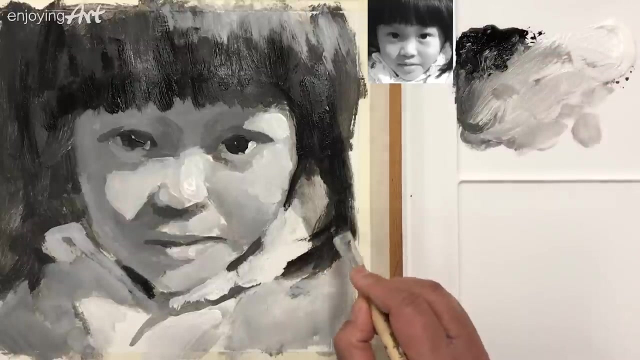 Like this And There's a little rough texture, Rough contact, And actually make it look more As The feeling of the hair Right. So If you continue Doing a little more And the painting will look more finished, But This is. 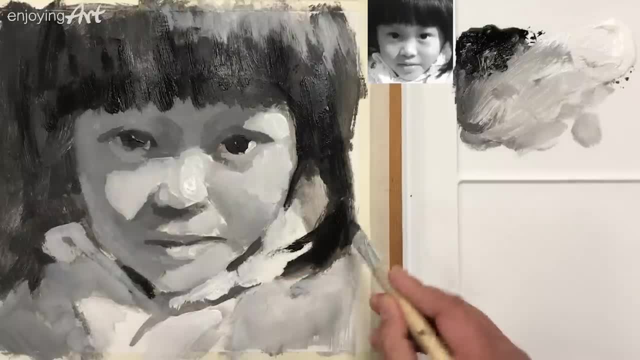 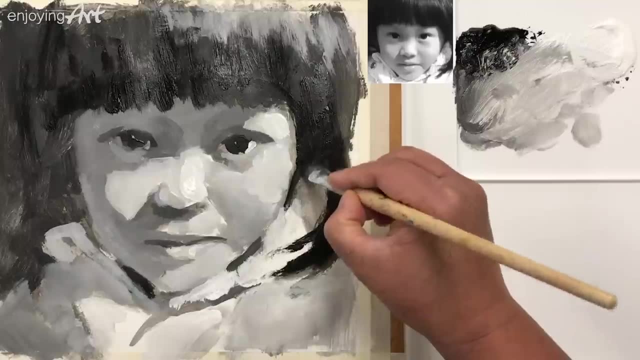 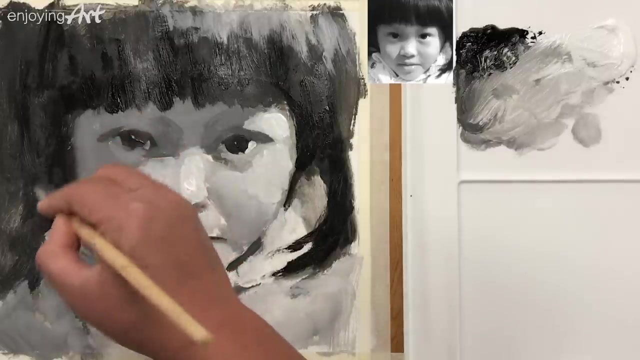 how It started And this is how You can Paint anything, Make it look like It, If you only thinking about How dark is that color And How to mix that color And put it in the place Painting anything. 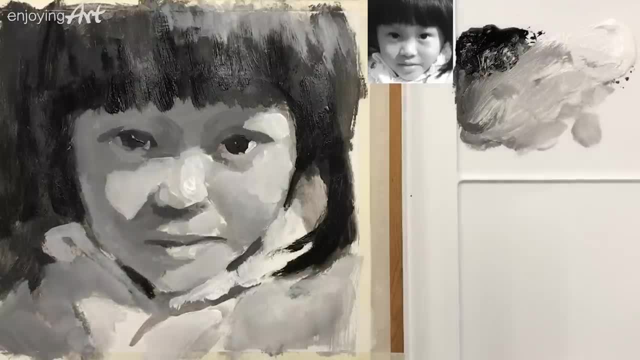 Just like find out The twenty five blocks of colors, And that's it. So painting is that simple? Most of the time We cannot paint because we confuse ourselves. We keep thinking about, Oh, How I'm going to make that eye. As soon as you think about, it's not an eye.